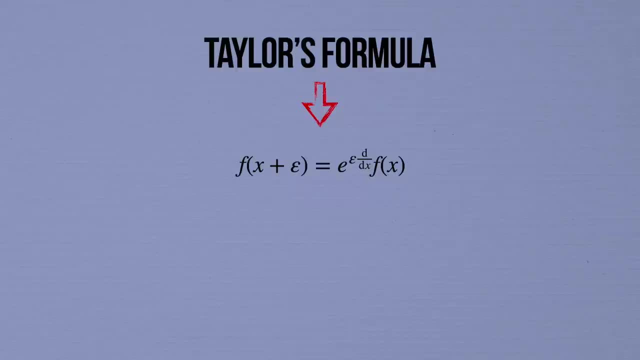 you've taken a calculus class. though you might not have written it in this nice and compact notation, I'll show you that it's equivalent to the Taylor series that lets us expand any smooth function in powers of x. In the first half of the video I'm going 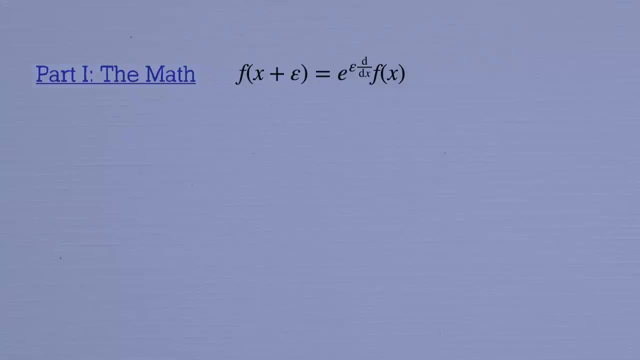 to explain where this incredibly important formula comes from and what it means, And then, in the second half, I'll tell you about three applications in physics where it shows up, Though, again, you'd be hard-pressed to find a chapter of any physics textbook where 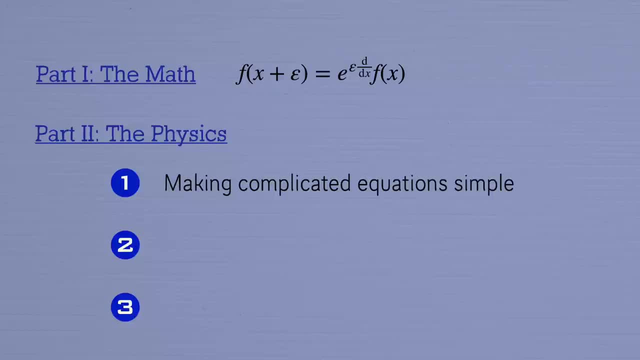 it's not applied. Number one: we'll look at how the Taylor series enables us to understand the complicated equations we often need to solve in physics by studying a limit where the equations simplify. Second, I'll show you how Einstein's E equals mc squared, or actually his more general formula for the energy of a relativistic particle. 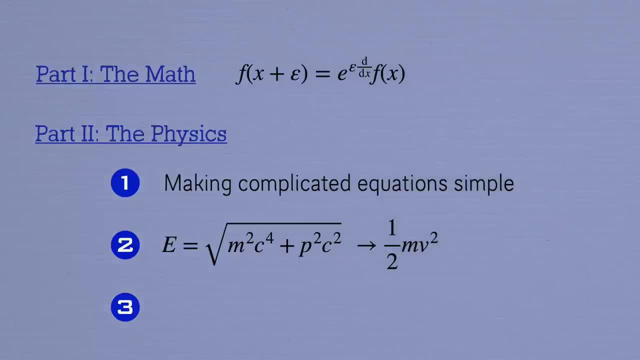 of mass m and momentum p, correctly reproduces the more familiar kinetic energy, one-half mv squared for particles that aren't moving too close to the speed of light. And also how that same Taylor series leads to the fine structure of the energy that we need to solve. 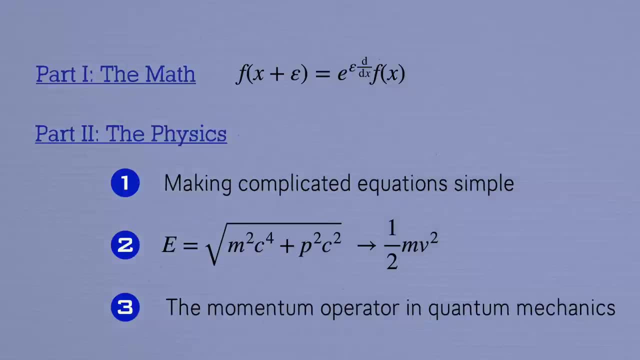 for the energy levels of the hydrogen atom. And third, we'll look at how Taylor's formula leads directly to the definition of the momentum operator in quantum mechanics. I'm not assuming you've learned much about relativity or quantum mechanics before, by the way. The point is just to see some of the different ways that. 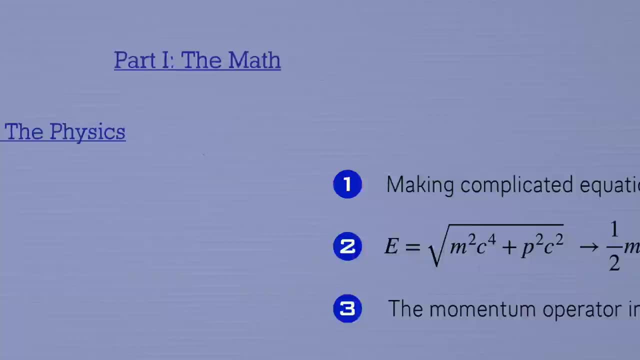 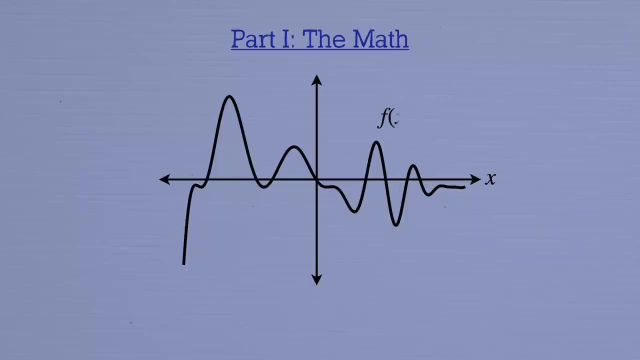 Taylor's formula shows up in different areas of physics, So let's start with the math and understand what this formula is all about. Say we have some function f. Here's a random example. It looks really complicated. But instead of trying to understand the whole complicated equation, we'll use the formula to solve for the momentum operator in quantum mechanics. 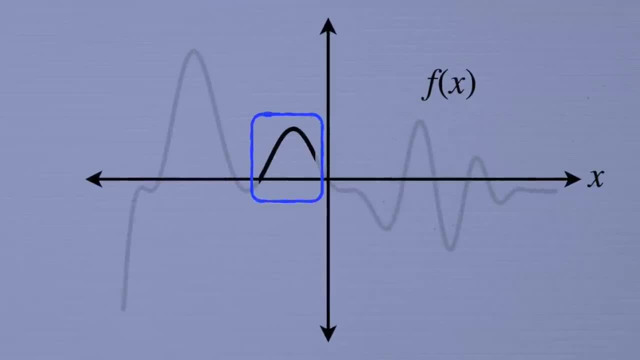 Let's zoom in and look at it in a smaller region, where it's a lot simpler. Take this point here, for example, And let's choose our origin, so that this point is sitting at. x equals zero, So the height of the function there is f. Imagine that this curve is the. 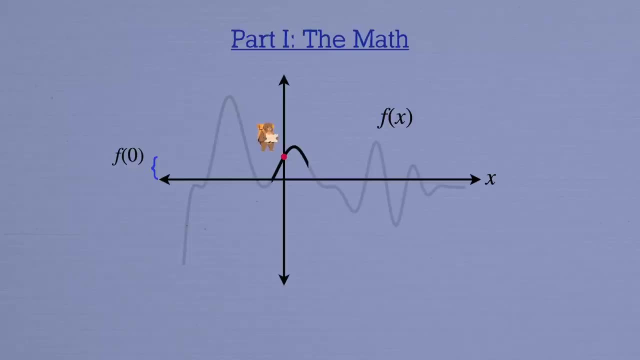 shape of a treacherous mountain and you're an intrepid explorer plotting out its map. You're high up in the air and it's very foggy, so you can't see very far in either direction. You just need to carefully walk along the mountain and record its shape using an altimeter. that 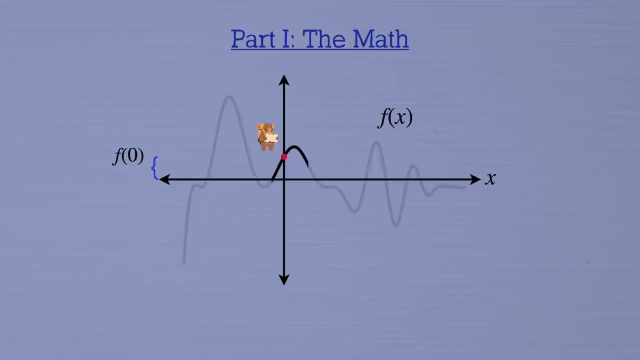 measures your height above the ground. starting from this point, x equals zero. Initially, all you can say is that your starting height is f. For all you know, the whole mountain might just be a flat horizontal line at this height. Then, when you try to, 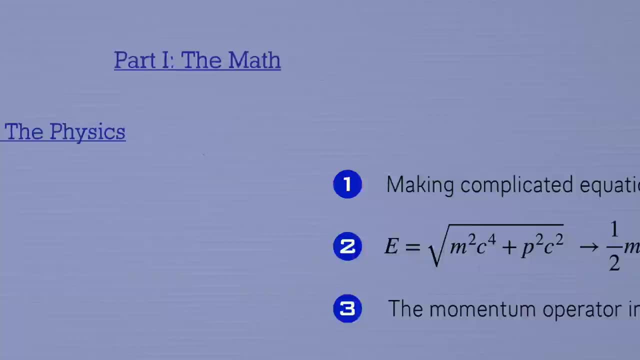 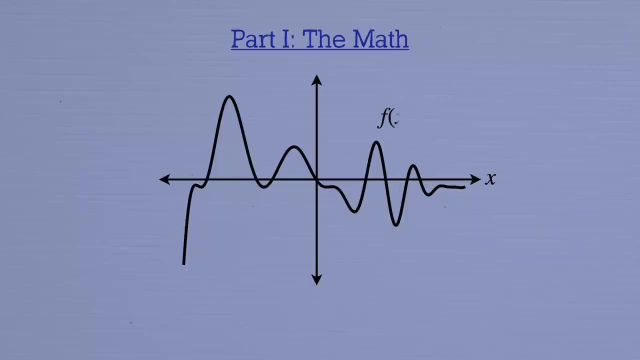 Taylor's formula shows up in different areas of physics, So let's start with the math and understand what this formula is all about. Say we have some function f of x. Here's a random example. It looks really complicated. But instead of trying to understand the whole complicated equation, we'll use the formula to solve for the momentum operator in quantum mechanics. 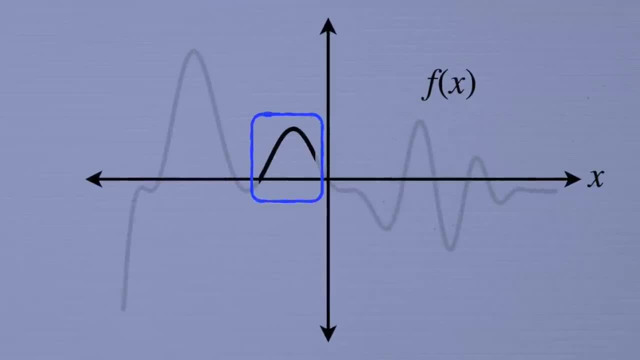 Let's zoom in and look at it in a smaller region, where it's a lot simpler. Take this point here, for example, And let's choose our origin, so that this point is sitting at x equals 0. So the height of the function there is f of 0.. Imagine that this curve is the 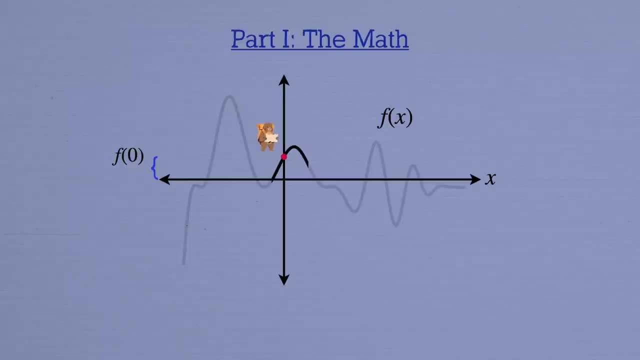 shape of a treacherous mountain and you're an intrepid explorer plotting out its map. You're high up in the air and it's very foggy, so you can't see very far in either direction. You just need to carefully walk along the mountain and record its shape using an altimeter. 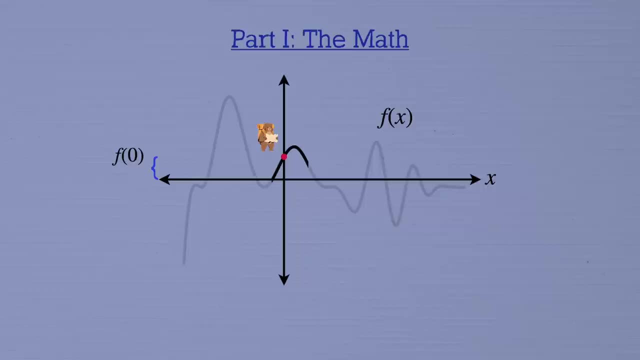 that measures your height above the ground. starting from this point, x equals 0.. Initially, all you can say is that your starting height is f of 0. For all you know, the whole mountain might just be a flat horizontal line at this height. Then, when you try to write, 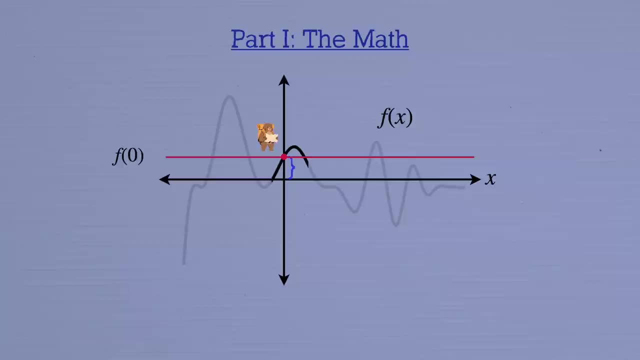 down in your field journal a function that describes the height of the mountain. your first guess is just: f of x equals f of 0, a horizontal line at your starting height. But now you take a little hop to the right and you discover that the height of the mountain 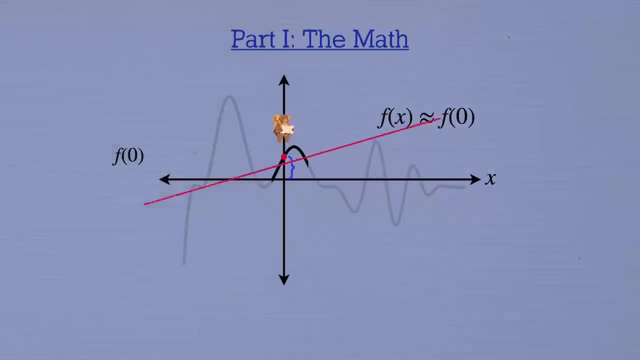 has changed. Instead, as far as you can tell, now it looks like a line that's sloped at an angle where the slope is given by the first derivative of f at x equals 0.. Now your new best guess for the height function is the equation of this sloped line: f of x equals f of 0 plus. 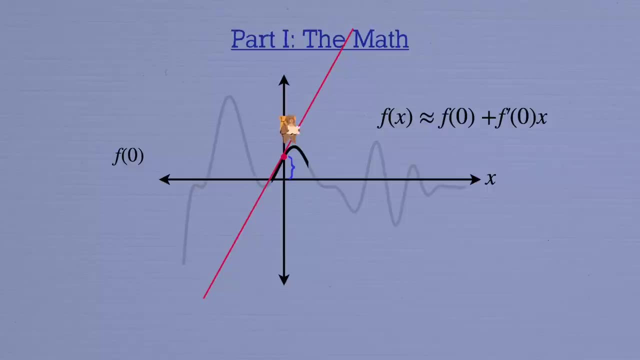 f prime of 0 times x. But now you take another hop and you discover that the curve isn't a straight line after all. Instead it starts to deflect away from a line like a parabola. So now you expect there's a better approximation to the function, like this: 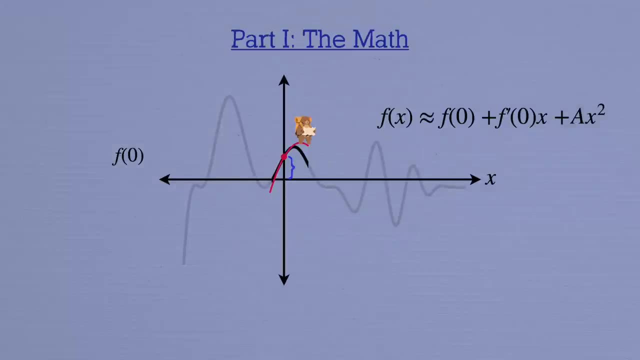 With an x squared term and some coefficient a in front of it. But at this point you start to think to yourself that you might be able to get an even better description of the function over a wider range by including many more powers of x, x, cubed, x to the fourth and 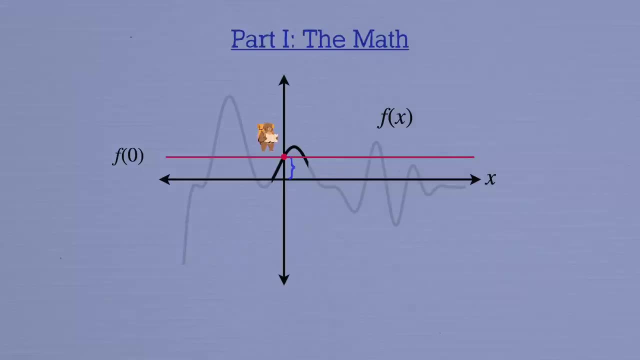 write down in your field journal a function that describes the height of the mountain. your first guess is just: f equals f, a horizontal line at your starting height. But now you take a little hop to the right and you discover that the height of the mountain 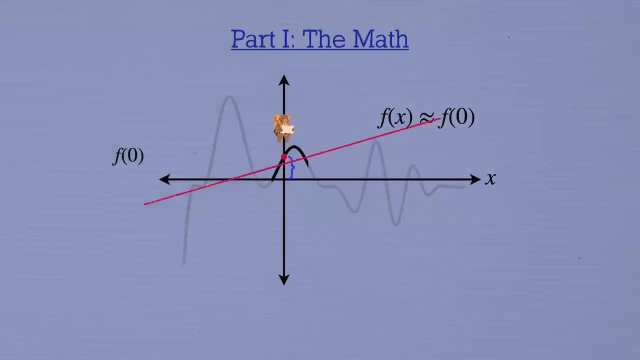 has changed, So it's not actually an f a line. Instead, as far as you can tell, now it looks like a line that's sloped at an angle, where the slope is given by the first derivative of f, at x equals zero. 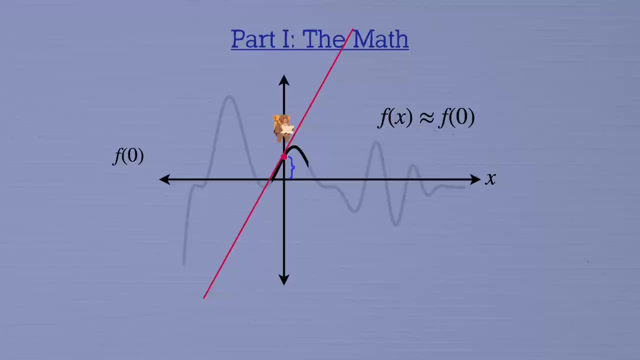 Now your new best guess for the height function is the equation of this sloped line: f of x equals f of zero plus f, prime of zero times x. But now you take another hop and you discover that the curve isn't a straight line after: 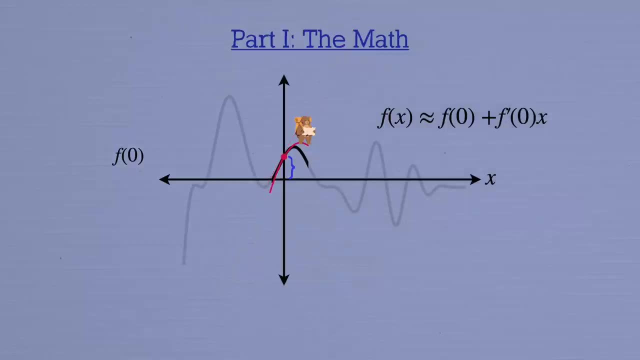 all. Instead it starts to deflect away from a line like a parabola. So now you expect there's a better approximation to the function like this, with an x squared term and some coefficient a in front of it. But at this point you start to think to yourself that you might be able to get an even better. 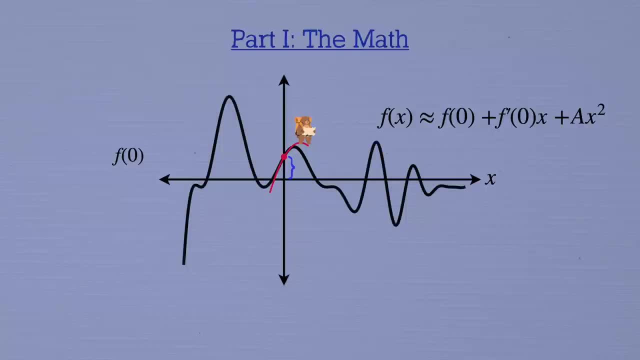 description of the function over a wider range by including many more powers of x, x, cubed x to the fourth, and so on. So you stop exploring for a moment and sit down to do some math. You want to express this function, f, as a sum of powers of x, with some coefficients c. 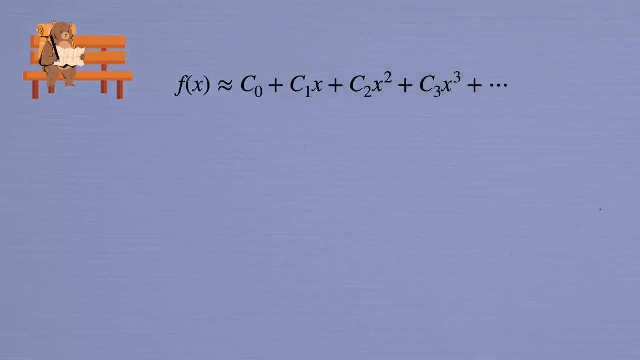 zero, c one, c two and so on. The question is how to pick these numbers so that this series does a good job of matching up with f. Well, we've already seen what the first couple of coefficients are. When we plug in, x equals zero, everything except the first term disappears and we get. 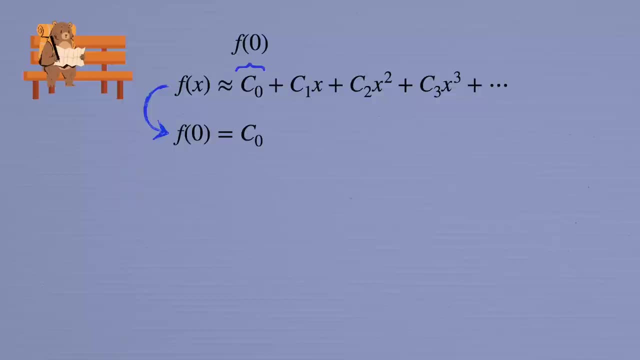 f of zero equals c zero. So that first number in the series is just the value of the function. at our starting point, x equals zero. As for the next one, c, one x and everything after it disappears when we plug in, x equals zero. 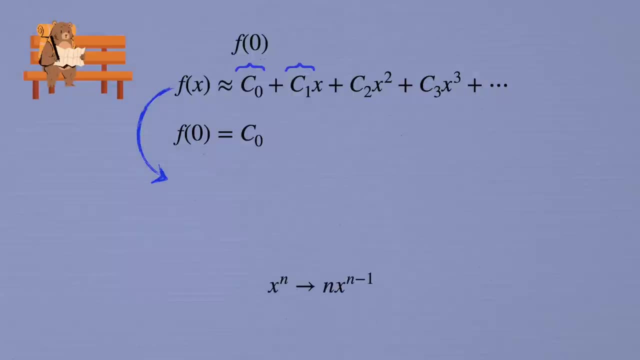 But what if we take the derivative first, Remembering the rule that to take the derivative of x to the n we bring the power down out front and then reduce the exponent by one. We get f. prime of x equals c. one plus two, c two times x plus three. c, three x squared. 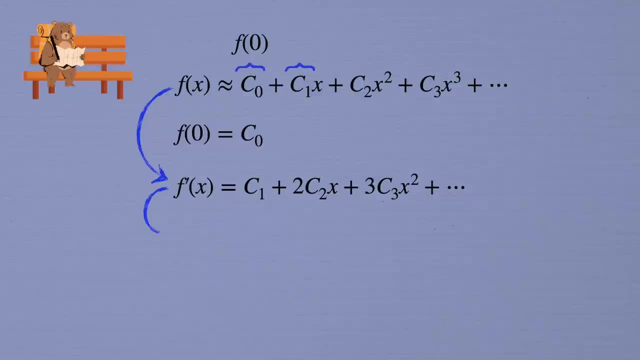 plus dot dot dot. Now, when we plug in x equals zero, the c one term survives: F. prime of zero equals c one. So again, like we already knew, we should set this first coefficient, c one, to be the derivative of f at x equals zero. 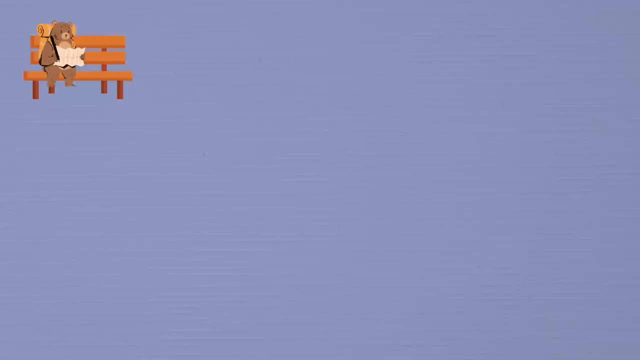 so on. So you stop exploring for a moment and sit down to do some math. You want to express this function, f, as a sum of powers of x with some coefficients: c0,, c1,, c2, and so on, So that this series does a good job of matching up with f. 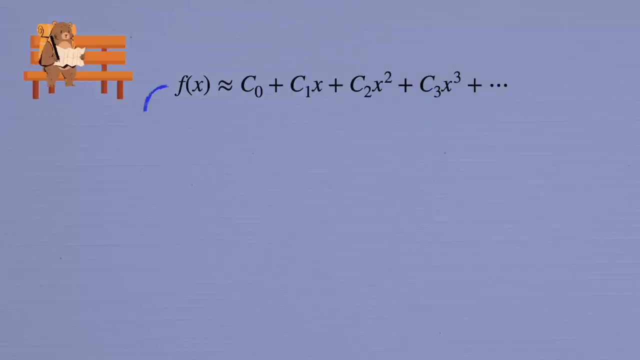 Well, we've already seen what the first couple of coefficients are. When we plug in, x equals 0, everything except the first term disappears and we get f of 0 equals c0.. So that first number in the series is just the value of the function at our starting point. x equals. 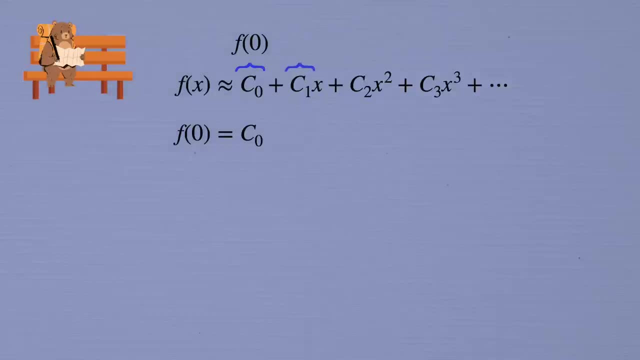 0.. As for the next one, c1, and everything after it disappears when we plug in: x equals 0.. But what if we take the derivative first, Remembering the rule that, to take the derivative of x to the n, we bring the power of x to the p, squared over the first value of the? 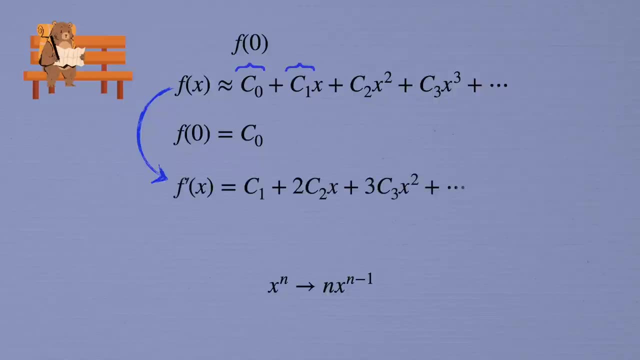 down out front and then reduce the exponent by 1. We get f prime of x equals c1 plus 2c2 times x plus 3c3, x squared plus dot dot dot. Now when we plug in, x equals 0, the c1 term survives. 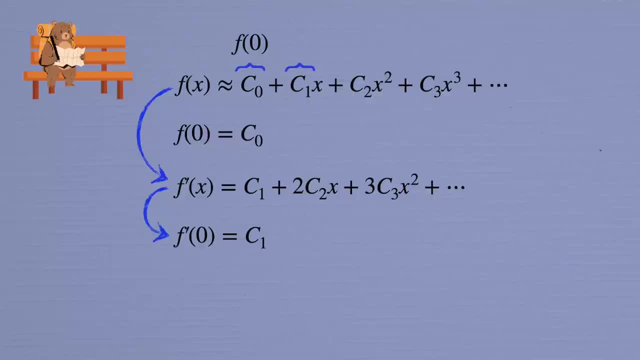 f prime of 0 equals c1. So again, like we already knew, we should set this first coefficient, c1, to be the derivative of f at x equals 0. But now we've got the idea. If we take the derivative again, we get f double prime of x equals 2c2, plus 3 times 2, c3, x, and so on. And so when we plug in, 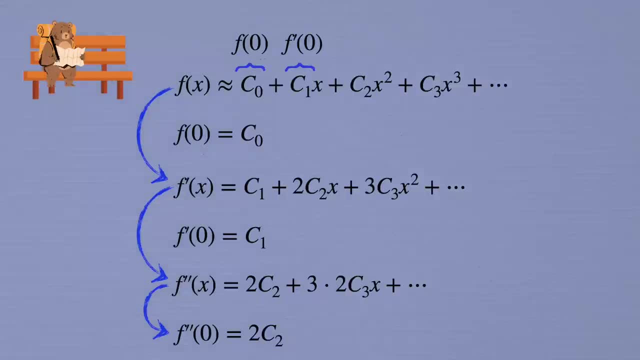 x equals 0, we learn that f double prime of 0 equals 2c2.. Then we should choose c2 to be half, the second derivative of f at x equals 0. And on and on it goes. Hopefully you see the pattern. 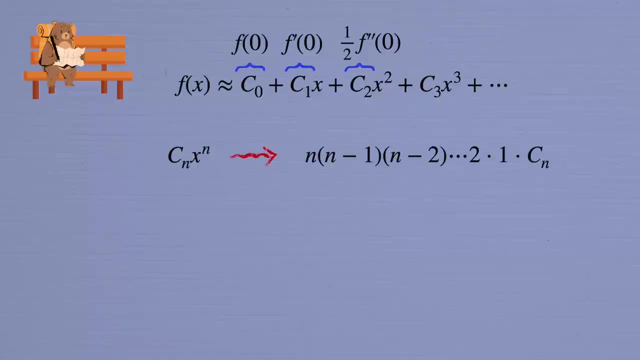 For the x to the n term in the sum, we need to take the derivative n times until this is the only term that's around. when we plug in, x equals 0.. Each derivative brings down a pattern of x to the n term in the sum. Each derivative brings down a pattern of x to the n. 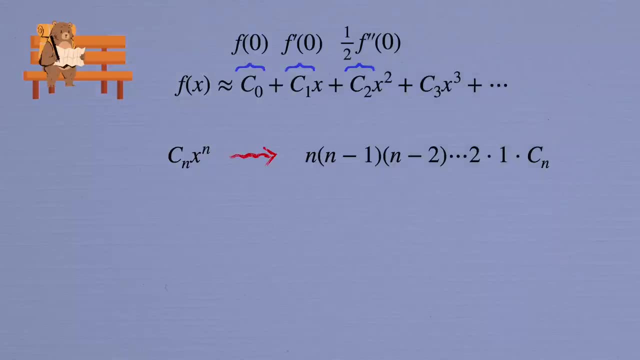 term in the sum. Each derivative brings down a pattern of x to the n term in the sum, First n, then n minus 1, n minus 2,, and so on all the way down to 3,, 2,, 1.. In other words, the nth derivative. 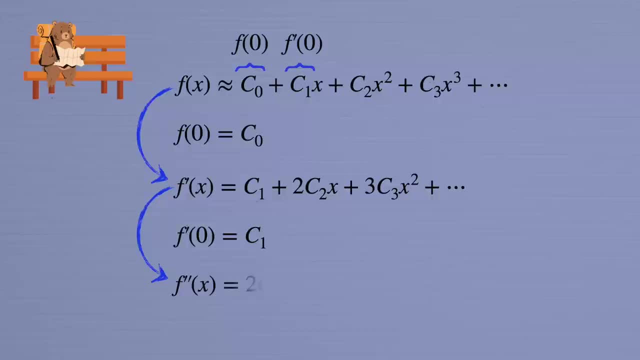 But now we've got the idea. If we take the derivative again, we get f prime of zero plus two c, two times x plus dot dot dot. So again we get f double prime of x equals two c, two plus three times two c, three x. and. 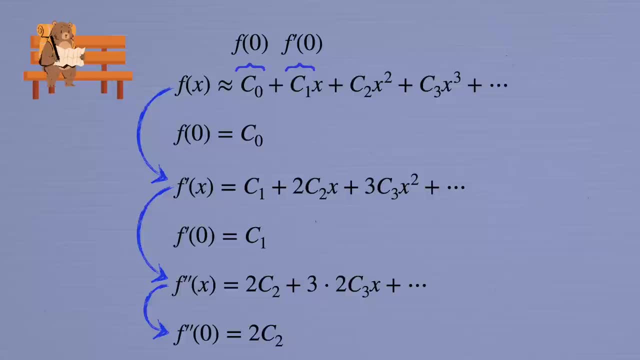 so on. And so when we plug in x equals zero, we learn that f, double prime of zero, equals two, c two. Then we should choose c two to be half the second derivative of f at x equals zero. And on and on it goes. 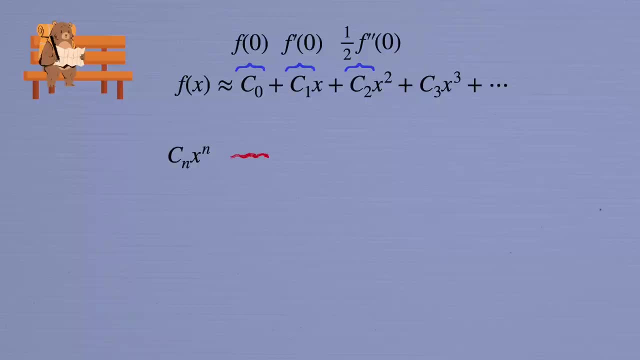 Hopefully you see the pattern. For the x to the n term in the sum, we need to take the derivative n times until this is the only term that's around. when we plug in, x equals zero. Each derivative brings down a power, First n, then n minus one, n minus two, and so on all the way down to three, two, one. 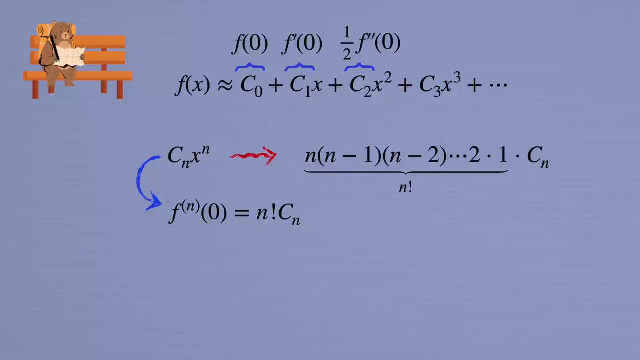 In other words, the nth derivative is n factorial times, c, n. So the nth coefficient is one over n factorial times. the nth derivative of f, evaluated at x, equals zero For this x cubed term. for example, we get one over three factorial, which is one. sixth, 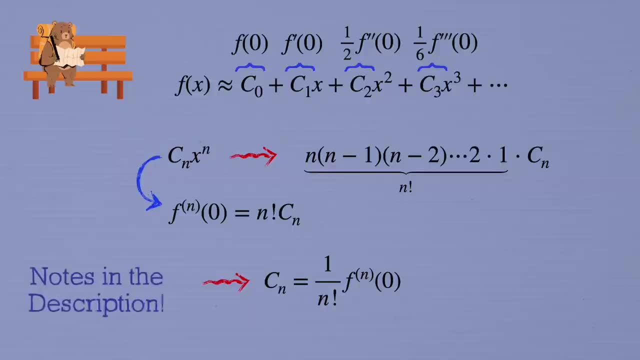 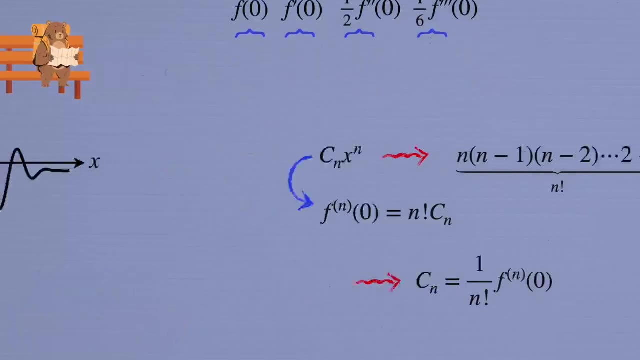 times the third derivative of f at zero. By the way, I go through all this step by step in the notes which you can get at the link in the description. You can dig through all the details here after you've watched. Now we're in business. 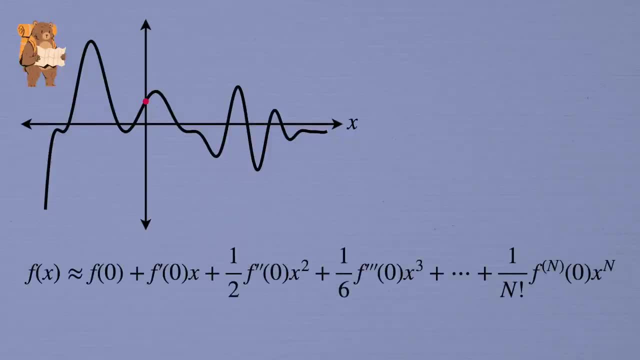 We've written an approximation for our function f as the sum of powers of x. This is the Taylor series for f When x is tiny, so that we're close to the starting point here, each higher power of x is an even tinier number than the one that came before it. 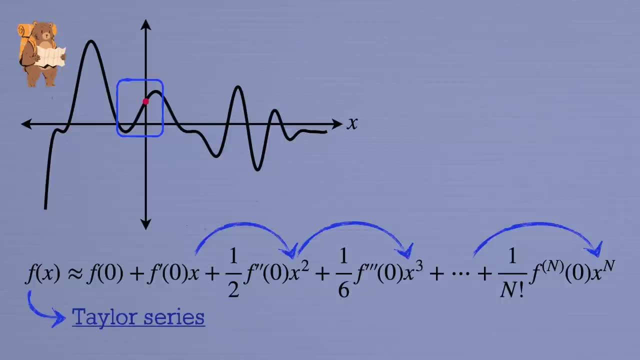 And so we already get a good approximation by keeping just the first few terms in the series. The farther away we venture from x equals zero- the more terms we need to include in the series in order to get a good description. But now that we have the general formula for the coefficients, we can include as many. 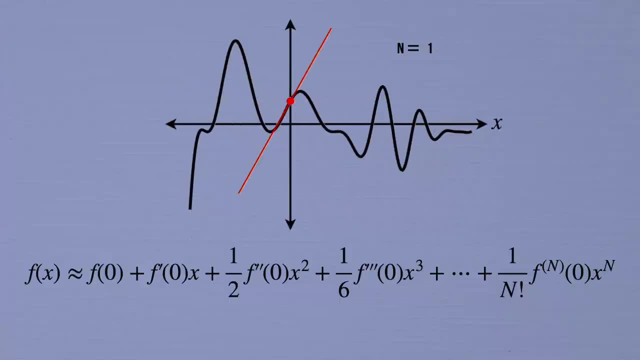 terms as we like. Here's what it looks like for this function. as we make the total number of terms bigger and bigger, You can see that the series approximation matches the curve better and better as n gets large. And here's the kicker: When we include all the terms by summing up the infinite series over all powers of x. 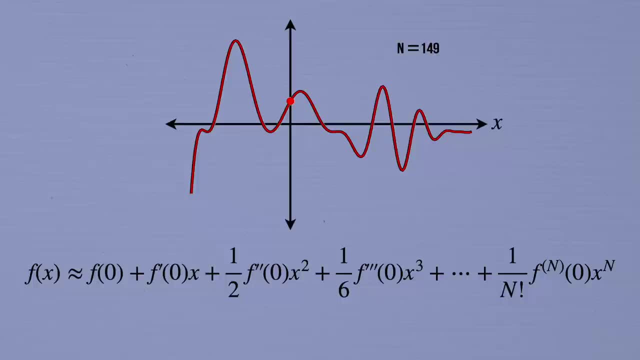 we actually reproduce the exact function that we started with, as long as it was smooth and well-behaved and the series converges. This is truly the best way to do it. I hope you enjoyed this video. It says that if we know all the derivatives of a smooth function, at a single point we 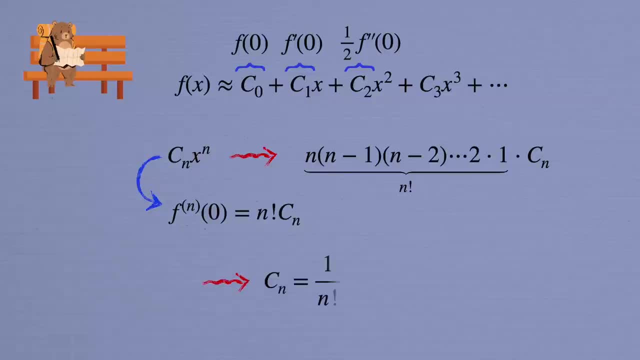 is n factorial times cn. So the nth coefficient is 1 over n factorial times. the nth derivative of f, evaluated at x, equals 0.. For this x cubed term, for example, we get 1 over 3 factorial, which is 1 sixth times the third derivative of f at 0.. By the way, I go through all this step, 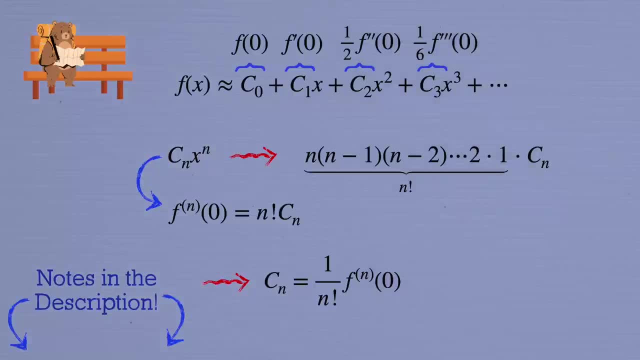 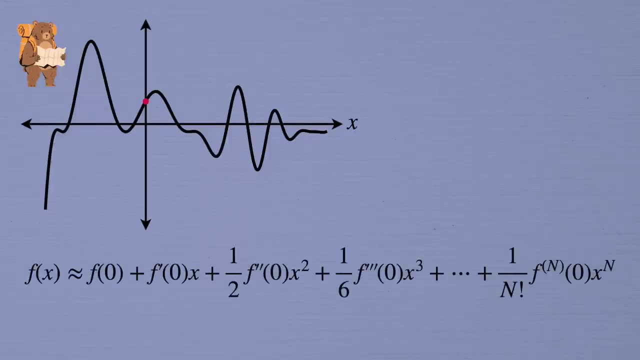 by step in the notes which you can get at the link in the description to dig through all the details here after you've watched. Now we're in business. We've written an approximation for our function f as the sum of powers of x. This is the Taylor series for f. 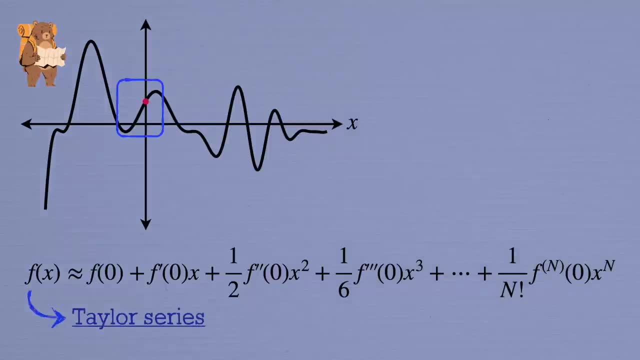 When x is tiny, so that we're close to the starting point here. each higher power of x is an even tinier number than the one that came before it, And so we already get a good approximation by keeping just the first few terms in the series. The farther away we venture from x. 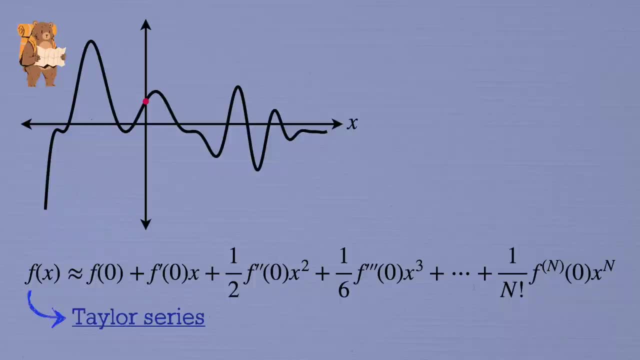 equals 0,, the more terms we need to include in the series in order to get a good description of the function. But now that we have the general formula for the coefficients, we can include as many terms as we like. Here's what it looks like for this function as we make the total number of 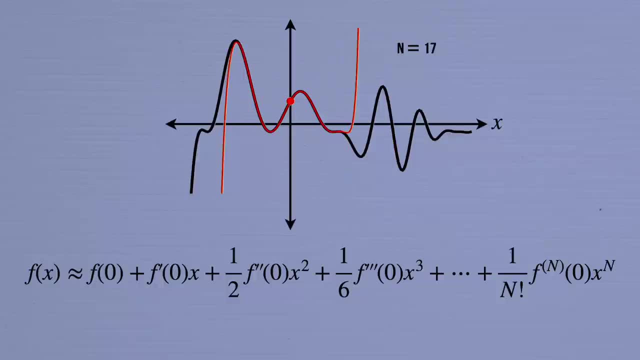 terms, bigger and bigger. You can see that the series approximation matches the curve better and better as n gets large. And here's the kicker: When we include all the terms by summing up the infinite series over all powers of x, we actually reproduce the exact function that we started with. 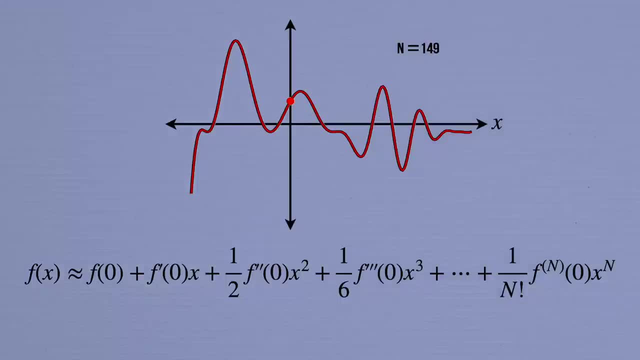 as long as it was smooth and well-behaved, and the series converges. This is truly a remarkable thing. It says that if we know all the derivatives of a smooth function at a single point, we can reconstruct the rest of the function everywhere else. Let's do some examples. 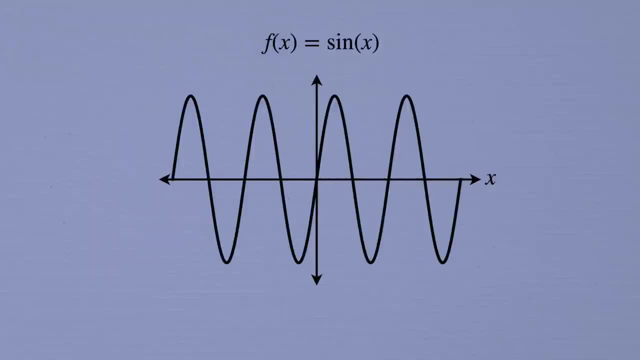 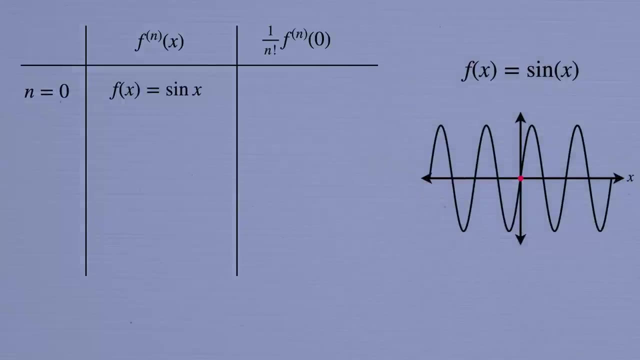 How about f of x equals sine of x. Let's write down its Taylor series around: x equals 0.. We just need to know what its derivatives are at that point. So let's make a little table. Sine of x passes through the origin, so we start off with: f of 0 equals 0. 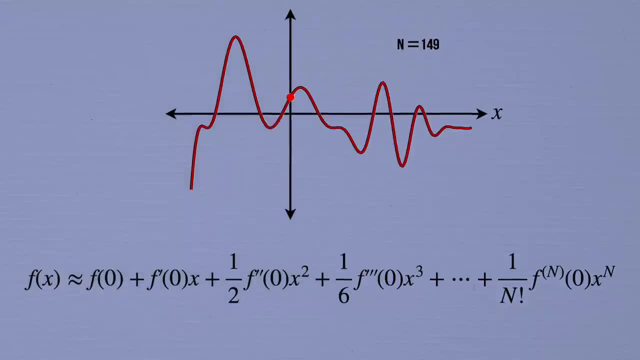 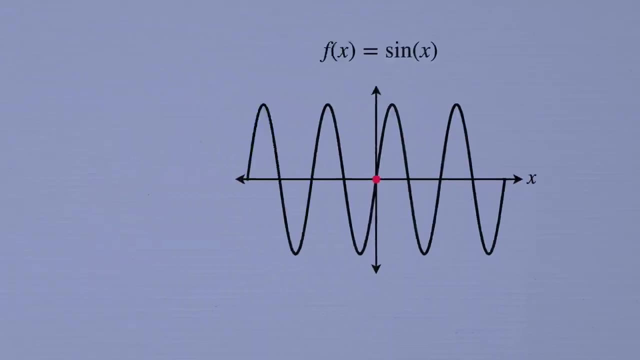 can reconstruct the rest of the function everywhere else. Let's do some examples. How about f of x equals sine of x. Let's write down its Taylor series around: x equals zero. We just need to know what its derivatives are at that point. 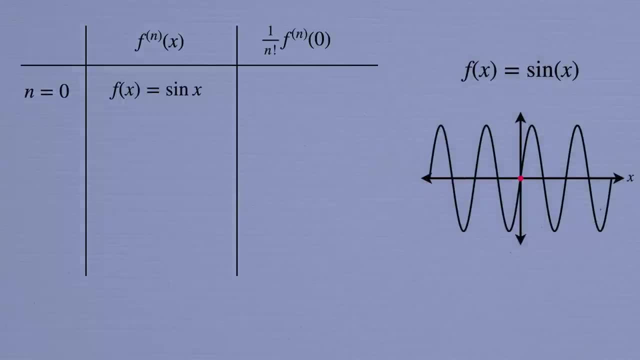 So let's make a little table. Sine of x passes through the origin, so we start off with f of zero equals zero. Zero factorial is defined to be one, by the way, and so this first term in the Taylor series is just zero. 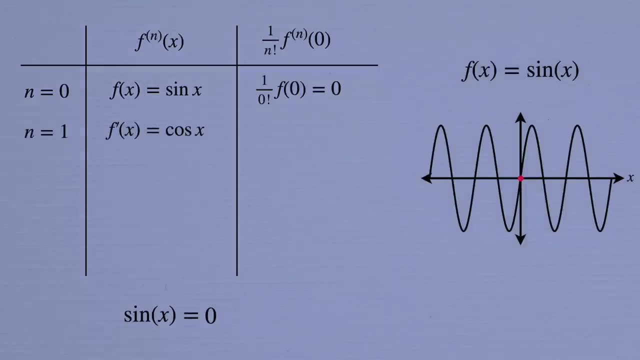 Next up we need the derivative of sine of x, which is cosine of x. Now when we plug in x equals zero, we get cosine of zero, which is one. And so the first interesting term in the Taylor series is just x, a straight line through. 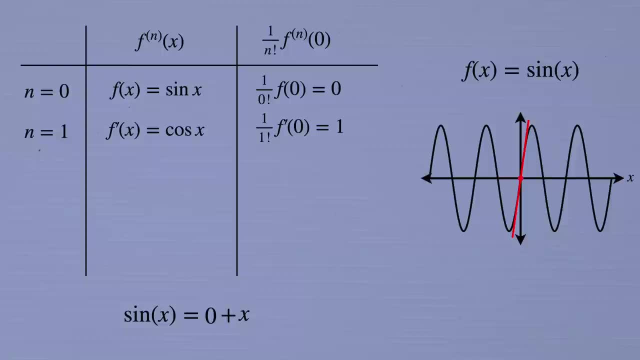 the origin with slope one. That's already a very good approximation to sine of x when x is a small number, and so we use the approximation sine of x equals x often in physics. But as x gets a little bigger, clearly the straight line isn't going to cut it anymore. 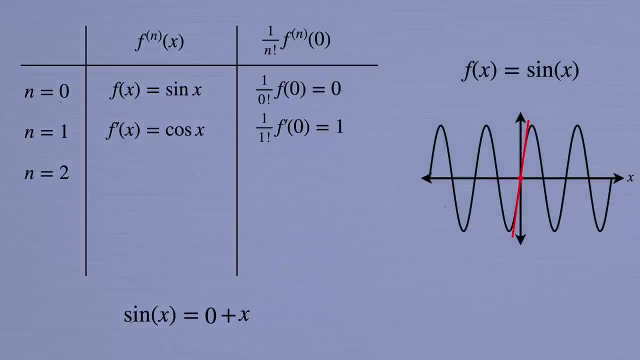 So let's keep going. For the next term we need the derivative of sine of x, which is cosine of x, which is cosine of x. Then we need the derivative of cosine of x, which is minus sine of x, But that vanishes again when x equals zero, and so the x squared term actually disappears. 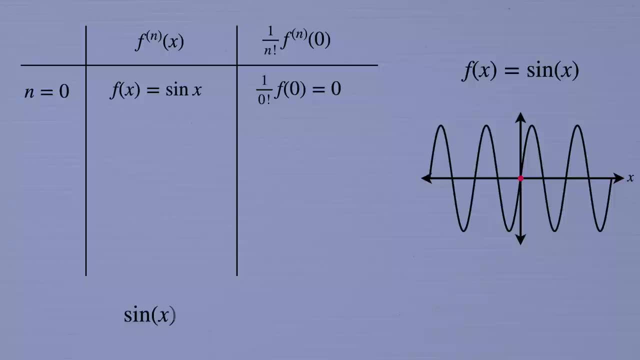 0. factorial is defined to be 1, by the way, and so this first term in the Taylor series is just 0.. Next up, we need the derivative of sine of x, which is cosine of x. Now, when we plug in x, 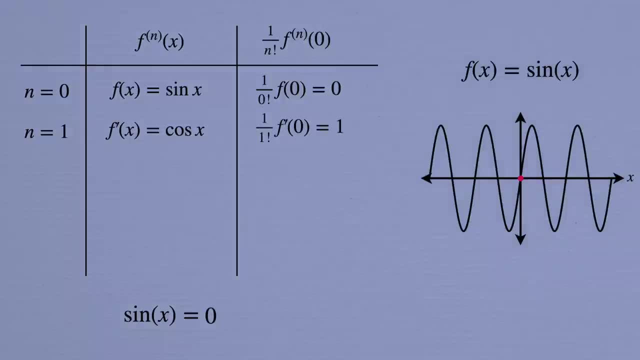 equals 0,, we get cosine of 0,, which is 1.. And so the first interesting term in the Taylor series is just x, a straight line through the origin with slope 1.. That's already a very good approximation to sine of x when x is a small number, and so we use the approximation sine of x equals x. 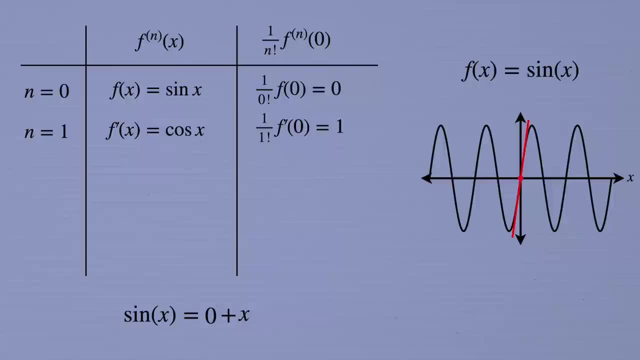 often in physics. But as x gets a little bigger, clearly the straight line isn't going to cut it anymore. So let's keep going For the next term. we need the derivative of sine of x, We need the derivative of cosine of x, which is minus sine of x. But that vanishes again when x. 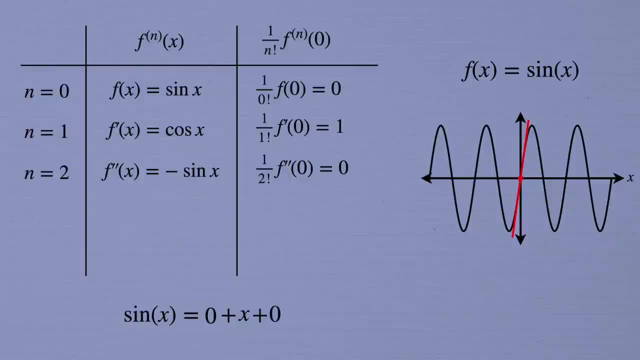 equals 0, and so the x squared term actually disappears. That's part of the reason the linear approximation was so good to begin with. Now for f triple prime of x, we need the derivative of minus sine and we get minus cosine. Then f triple prime of 0 equals minus 1,. 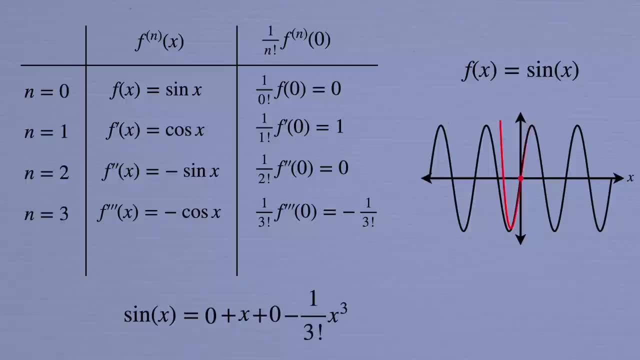 and so the cubic coefficient is minus 1 over 3 factorial. Let's do one more line. We want the derivative of minus cosine, which is sine. This vanishes again. x equals 0, and so there's no x to the 4 term in the series. We could keep going like this, and: 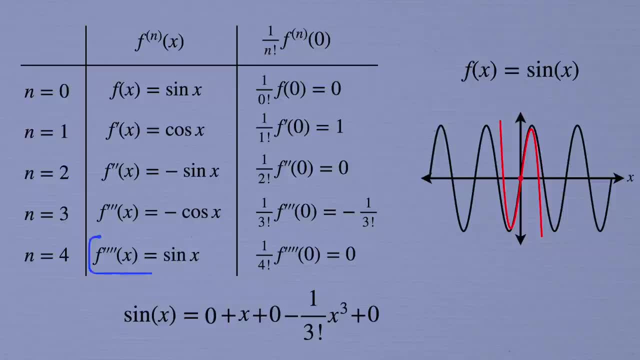 take more derivatives, But notice that with the fourth derivative here we've just gotten back to where we started with sine of x, So this same sequence of four derivatives is just going to repeat itself over and over again. Then we can just write down the whole series without any more work. 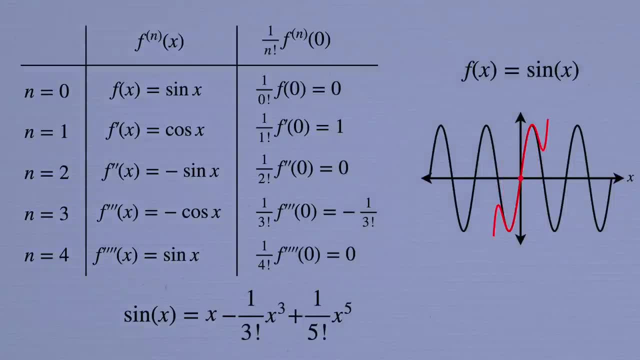 The next term is x to the fifth, over 5 factorial, followed by minus 1 over 7 factorial x to the seventh and plus 1 over 9 factorial x to the ninth. Here's what it looks like going up to x to the 29.. You can see that it does a good job reproducing. 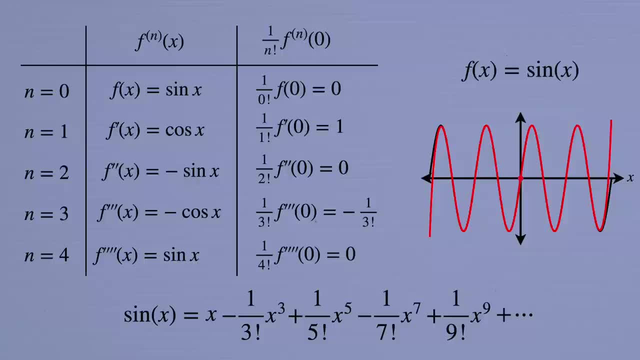 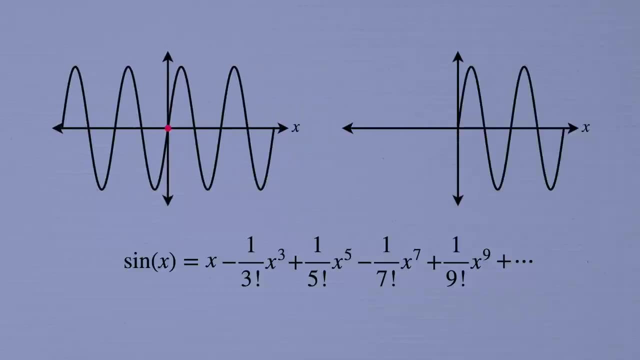 the sine curve right up to the edges of these four periods. Notice that only odd powers of x show up here in the Taylor series. That's because sine of x is an odd function. When you compare it on the right and left sides of the y-axis it looks the same, except that it's been flipped over. 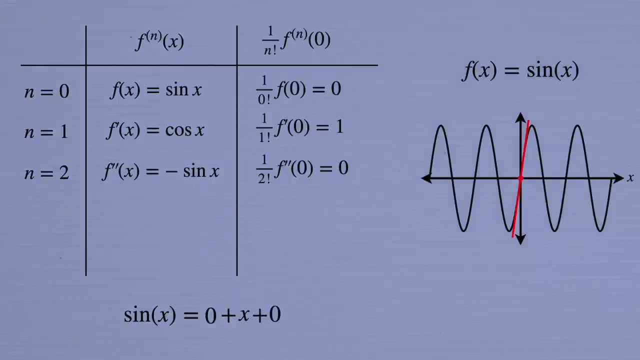 That's part of the reason the linear approximation was so good to begin with. Now for f triple prime of x, we need the derivative of minus sine, and we get minus cosine. Then f triple prime of zero equals minus one, and so the cubic coefficient is minus one. 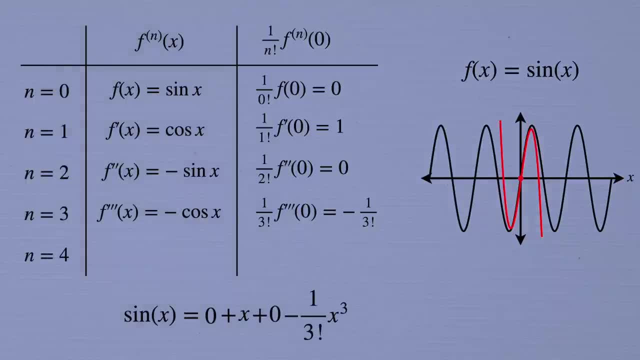 over three factorial. Let's do one more line. We want the derivative of minus cosine, which is sine. This vanishes again. Then we need the derivative of sine of x, which is cosine of x, which is cosine of zero, And so there's no x to the four term in the series. 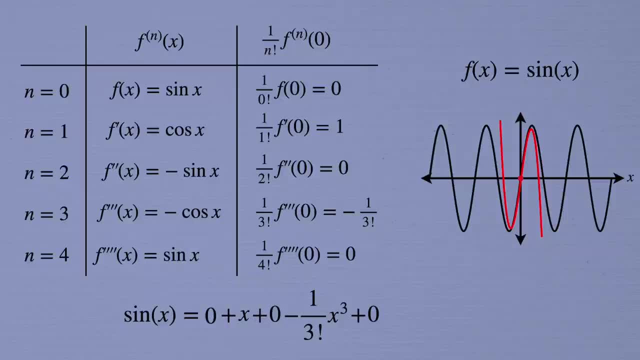 We could keep going like this and take more derivatives, But notice that with the fourth derivative here we've just gotten back to where we started with sine of x. So this same sequence of four derivatives is just going to repeat itself over and over again. 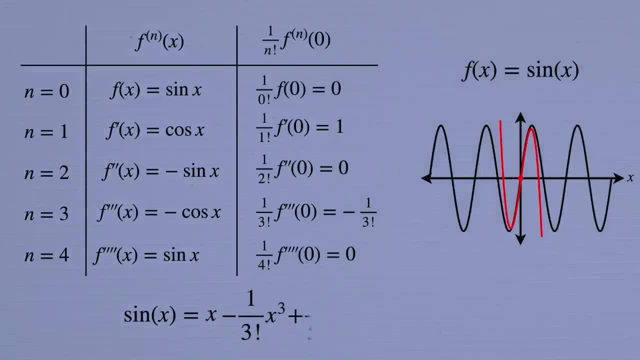 Then we can just write down the whole series without any more work. The next term is x to the fifth over five factorial, followed by minus one over seven factorial, x to the seventh And plus one over nine factorial, x to the nine, And so on. 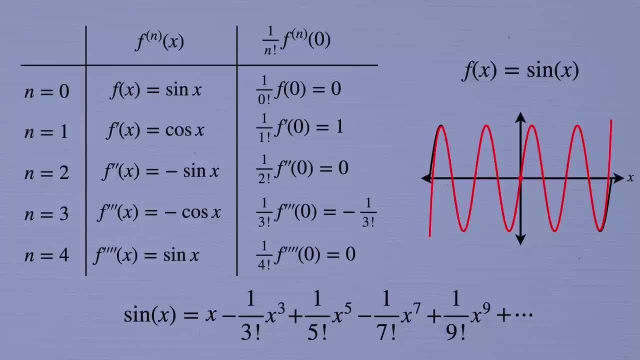 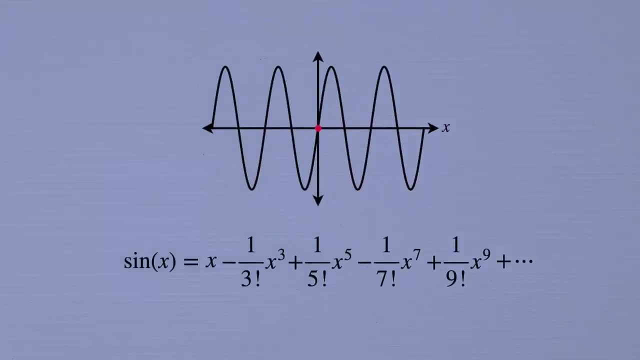 Here's what it looks like going up to x to the twenty-nine. You can see that it does a good job reproducing the sine curve right up to the edges of these four periods. Notice that only odd powers of x show up here in the Taylor series. 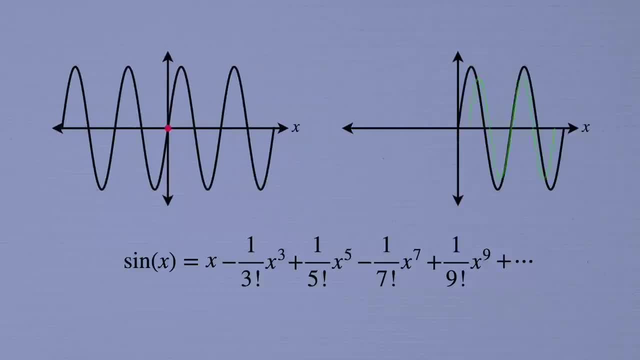 That's because sine of x is an odd function. When you compare it on the right and left sides of the y-axis it looks the same, except that it's been flipped over. In other words, sine of minus x equals minus sine of x. Odd powers of x share that property. 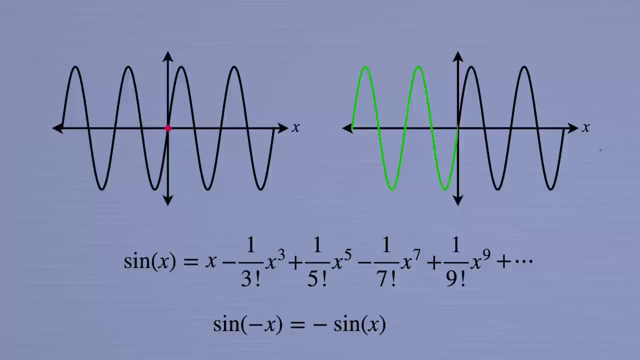 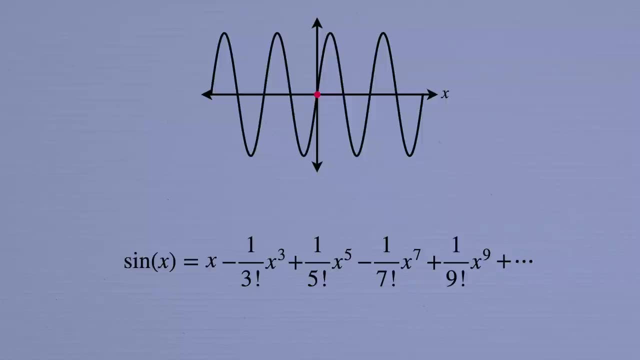 but even powers don't, And that's why there are no even powers of x in the Taylor series for sine. Like I mentioned before, oftentimes in physics we're not actually interested in the whole Taylor series. What we really want is a good approximation to a complicated function that makes a problem. 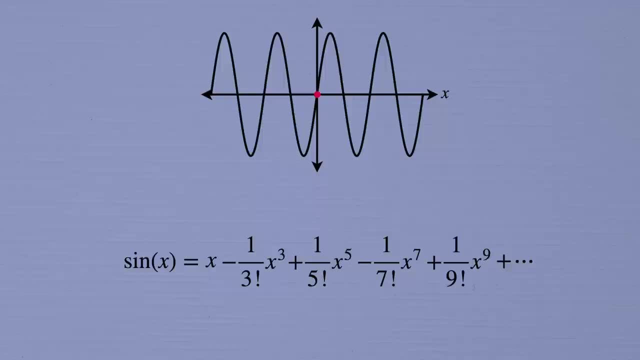 simpler to solve. I'll show you examples of what I mean in a minute. So in this case we might stop with the first term and just apply the fact that sine of x is approximately equal to x when x is small. This is called the small angle approximation, and you may have run into it in your first. 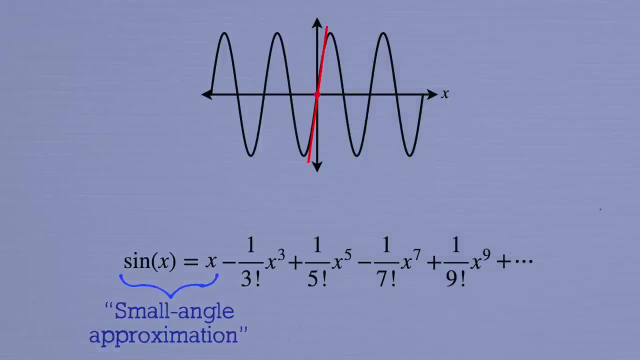 physics class. The key point here is that when x is small, like say 0.1,, then when we take larger powers of x in the successive terms in the Taylor series they get even smaller. x cubed equals 0.001,, x to the fifth equals 0.00001, and so on. 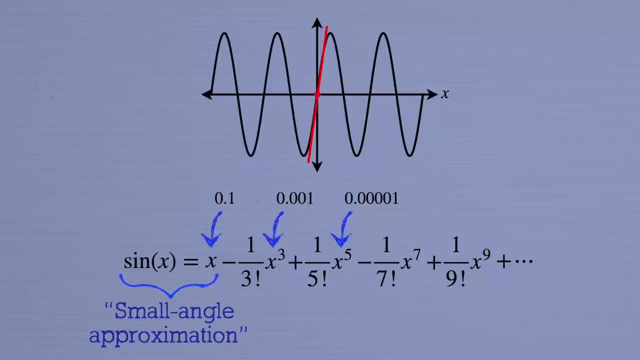 Not to mention the effect of the huge factorials in the denominators. That's why we can ignore the higher order terms for small x and get a good approximation to our function just by keeping the leading term. Let's do one more thing. 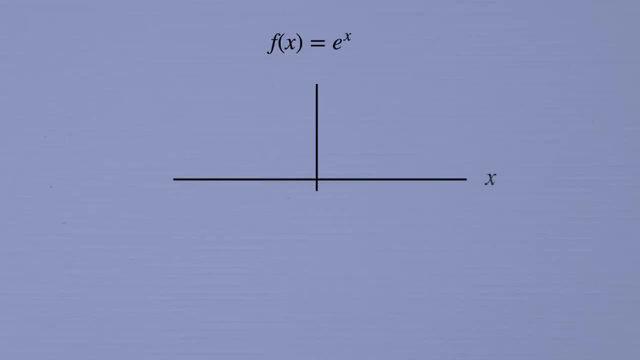 One more quick example: f of x equals e to the x. This will be important in a moment for seeing the slickest way to write down Taylor's formula. This one's easy, because the derivative of e to the x is just e to the x. again, and when. 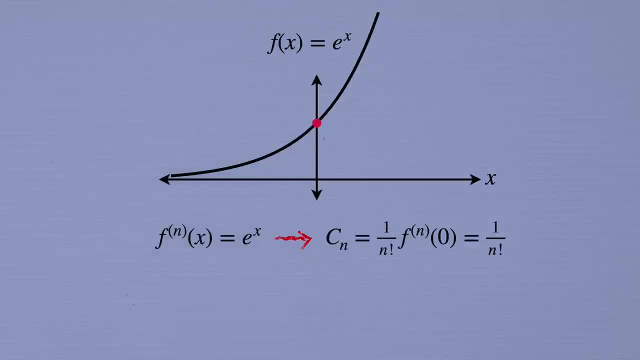 we plug in x equals 0,, we get 1.. And the coefficients are 1 over n factorial. So we can just jump right to the Taylor series e to the x equals 1 plus x plus 1 over 2 factorial x squared plus 1 over 3 factorial x cubed. 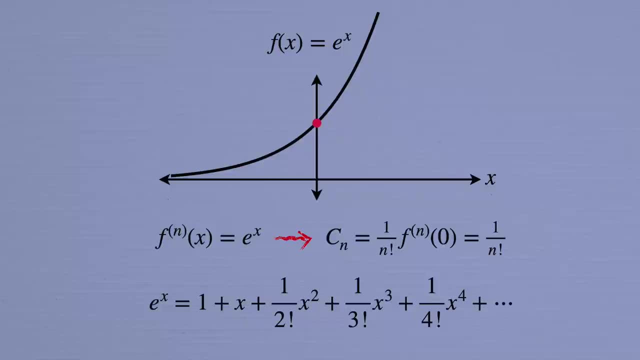 and so on. And once again, if x is tiny, then we can just plug in x to the x and we get 1 over n. factorial. We can get a good approximation by stopping at the linear term. It's not quite as good as we had for sin of x, though, because in that case the x squared. 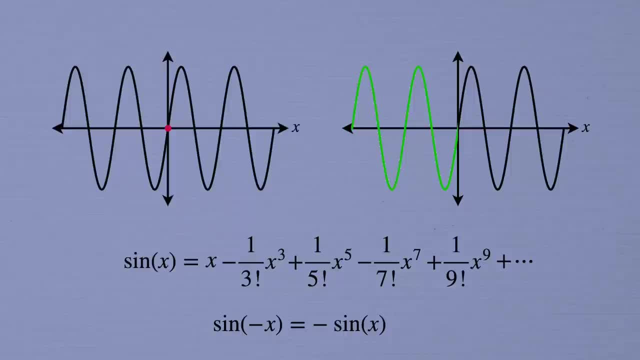 In other words, sine of minus x equals minus sine of x. Odd powers of x share that property, but even powers don't, And that's why there are no even powers of x in the Taylor series for sine. Like I mentioned before, oftentimes in physics we're not actually interested in the whole Taylor. 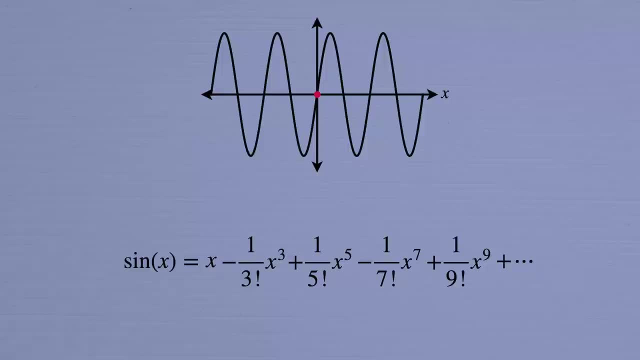 series. What we really want is a good approximation to a complicated function that makes a problem simpler to solve. I'll show you examples of what I mean in a minute. So in this case we might stop with the first term and just apply the fact that sine of x is approximately equal to x when x is. 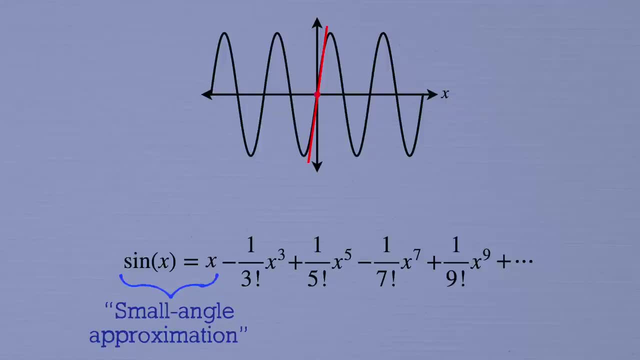 small. This is called the small angle approximation, And you may have run into it in your first physics class when you were just starting out with the first term. You might have run into it when you learned about the simple pendulum. The key point here is that when x is small, like, say, 0.1,. 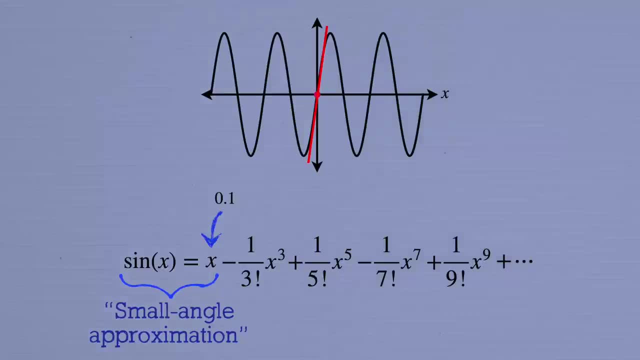 then when we take larger powers of x in the successive terms in the Taylor series, they get even smaller: x cubed equals 0.001,, x to the fifth equals 0.00001, and so on, Not to mention the effect of the huge factorials in the denominators. That's why we can ignore the higher. 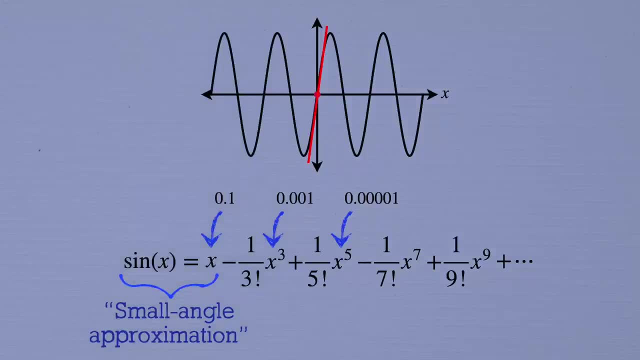 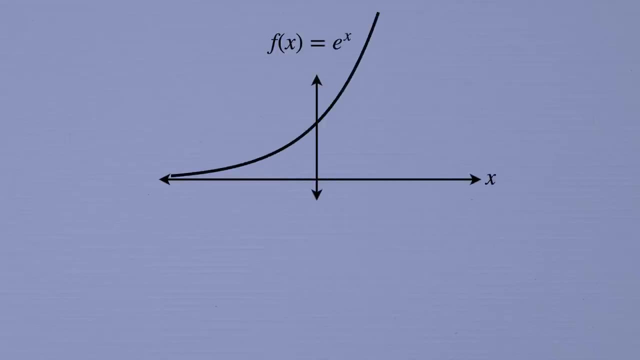 order terms for small x and get a good approximation to our function just by keeping the leading term. Let's do one more quick example. f of x equals e to the x. This will be important in a moment for seeing the slickest way to write down Taylor's formula. This one's easy because the derivative 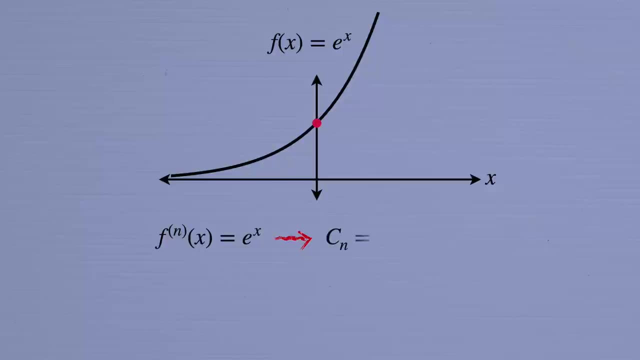 of e to the x is just e to the x again. And when we plug in x equals 0, we get 1.. And the coefficients are 1 over n factorial. So we can just jump right to the Taylor series. e to the x equals 1 plus x. 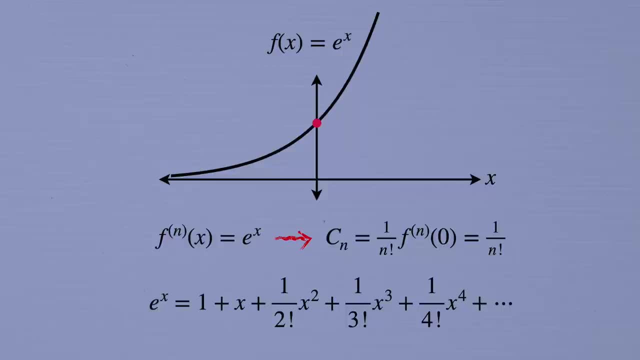 plus 1 over 2 factorial x squared, plus 1 over 3 factorial x cubed, and so on, And once again, if x is tiny, then we can get a good approximation by stopping at the linear term. It's not quite as good as we had for sine of x, though, because in that case the x squared correction vanished. 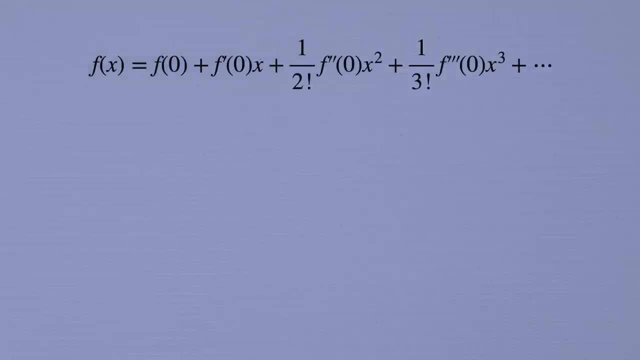 Now, before we get to the physics examples, the last thing I want to do is show you a few convenient ways of writing Taylor's formula. Spelling out the whole sum like this obviously isn't very concise, But we can write the same thing much more compactly using sum notation. 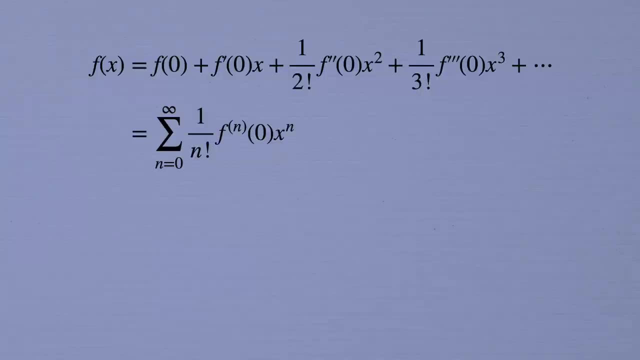 The sum over n of 1 over n factorial. the nth derivative of f, evaluated at zero times n. This is the Taylor series for f of x expanded around x equals 0.. But, come to think of it, there was nothing special about x equals 0 here. That's just where we happened to put the origin. 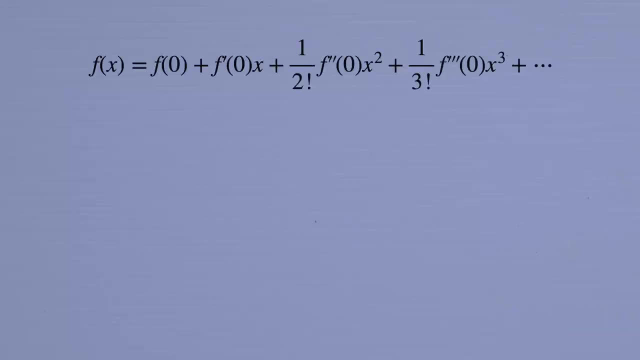 correction vanished. Now, before we get to the physics examples, the last thing I want to do is show you a few convenient ways of writing Taylor's formula. Spelling out the whole sum like this obviously isn't very concise, But we can write the same thing much more compactly using sum notation. 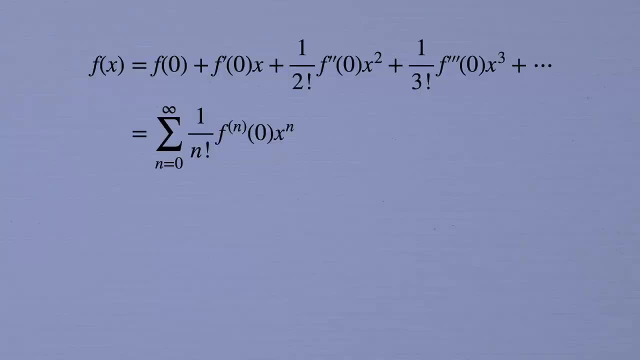 The sum over n of 1 over n factorial. the nth derivative of f, evaluated at 0, times x to the n. The sum over n of 1 over n factorial. the nth derivative of f, evaluated at 0, times x to the n. 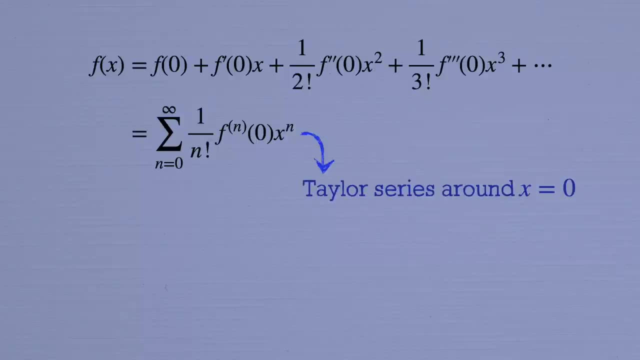 This is the Taylor series for f of x, expanded around: x equals 0.. But, come to think of it, there was nothing special about x equals 0 here. That's just where we happened to put the origin when we drew the graph of f of x. 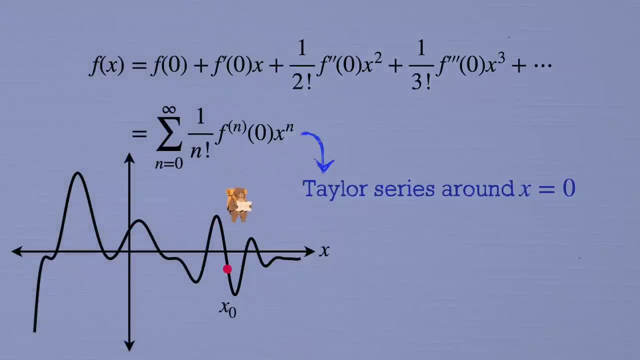 We could just as well write an expansion around any other point. call it x0, say. Then the Taylor expansion of f around x0 is given by the sum of 1 over n factorial times the derivatives of f evaluated at that starting point, x0, times the powers of the distance. 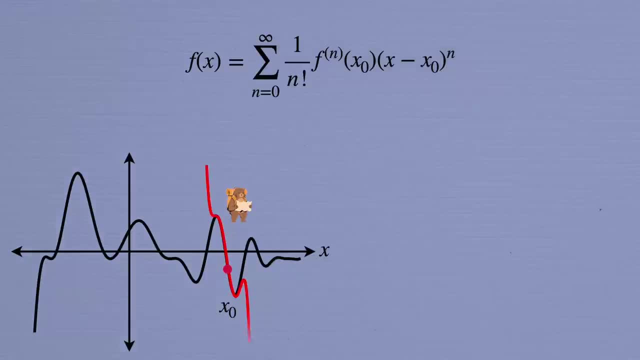 from there x minus x0.. For example, here's what we get with the first few terms of the Taylor series for this function expanded around this given point. Actually, there's another way of writing this expression that's often more useful. 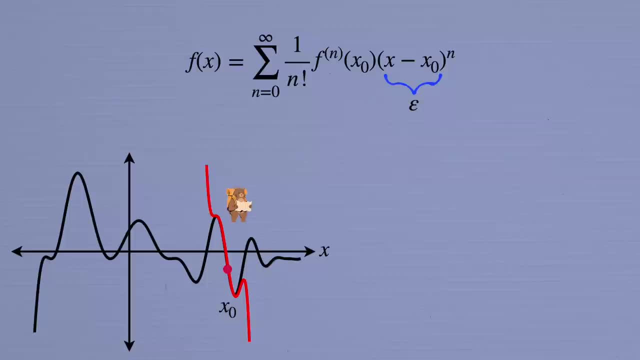 Let epsilon denote this quantity in parentheses: x minus x0. It measures how far away you are from the starting point. So when epsilon is small you're very close to x0, and as it gets bigger you get farther away. Then x is given by x0 plus epsilon. 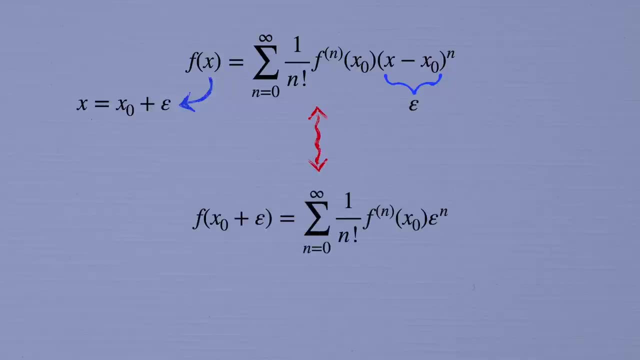 And we can write the same expression like this. This way of writing things makes it really clear that we can think of the Taylor series as starting at the point x0 and then expanding out away from there by evaluating f at x0 plus epsilon in powers of the displacement. 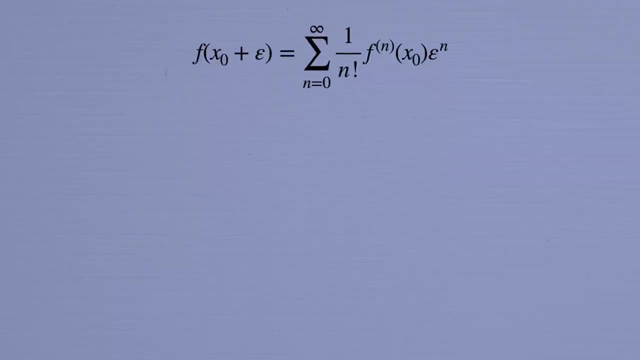 But this isn't even the slickest way to write the Taylor series, which is the formula I showed you at the very beginning of the video. To see how that works, we'll switch to the other notation for derivatives. So the nth derivative of f is obtained by applying d by dx to it n times or in other. 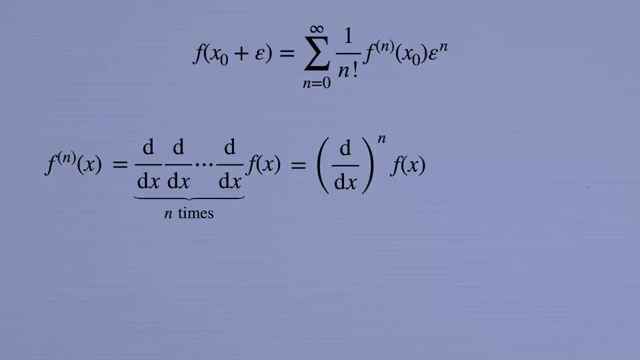 words d by dx to the power n acting on f. Then we'll plug this into the Taylor series And we'll see how that works. I went ahead and dropped the x0 subscript now because that was just a label that we don't need anymore. 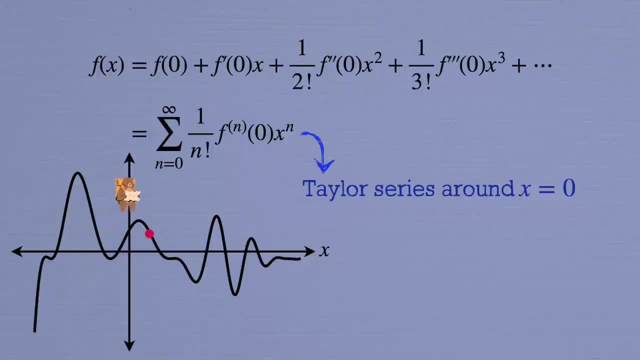 when we drew the graph of f of x, We could just as well write an expansion around any other point. call it x0, say. Then the Taylor expansion of f around x0 is given by the sum of 1 over n factorial times the derivatives of f evaluated at that starting point, x0 times the powers of the distance. 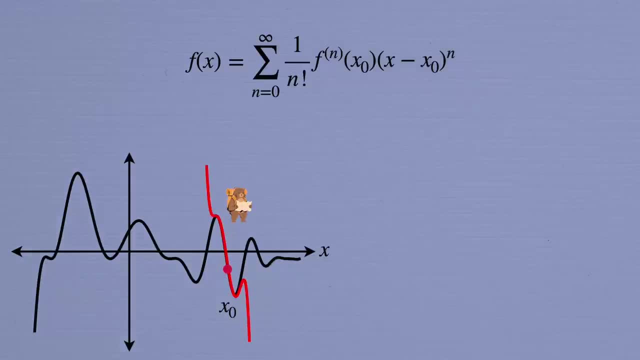 0.. For example, here's what we get with the first few terms of the Taylor series for this function, expanded around this given point. Actually, there's another way of writing this expression that's often more useful. Let epsilon denote this quantity in parentheses: x minus x0.. It measures. 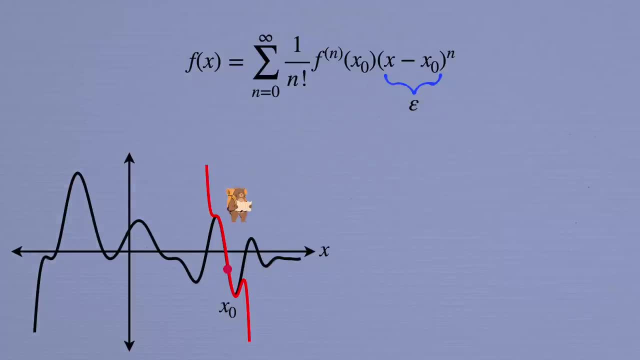 how far away you are from the starting point. So when epsilon is small you're very close to x0, and as it gets bigger you get farther away. Then x is given by x0 plus epsilon And we can write the same expression like this: This way of writing things makes it really. clear that x is the same as x0 plus x0.. This way of writing things makes it really clear that x is the same as x0 plus x0. This way of writing things makes it really clear. that this way of writing things makes it really clear that we can think of the Taylor series as 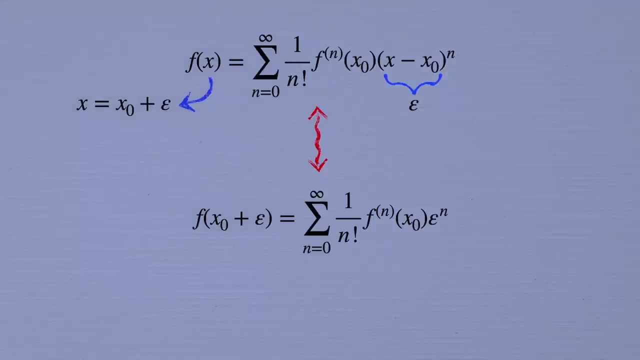 starting at the point x0 and then expanding out away from there by evaluating f at x0 plus epsilon in powers of the displacement. But this isn't even the slickest way to write the Taylor series, which is the formula I showed you at the very beginning of the video To see how that works. 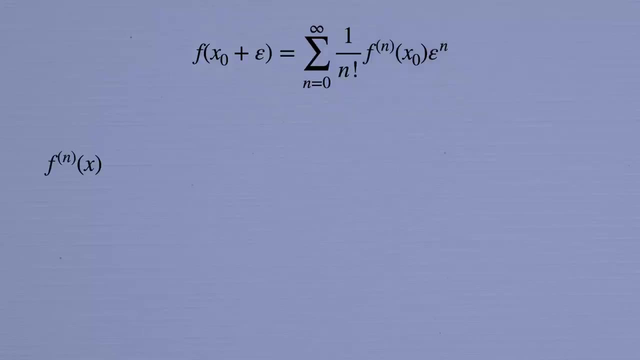 we'll switch to the other notation for derivatives. So the nth derivative of f is obtained by applying d by dx to it n times, or in other words d by dx to the power n acting on f. Then we'll plug this into the Taylor series, which lets us write it like this: I went ahead and dropped the x0. 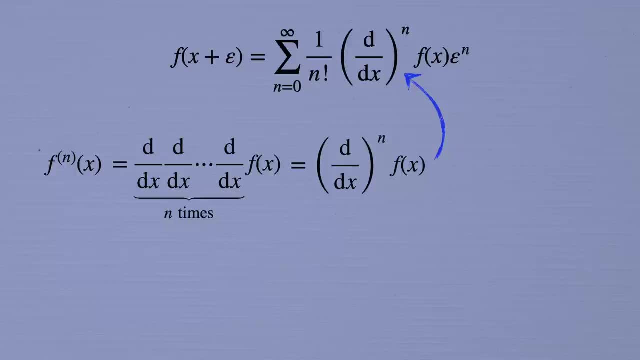 subscript now, because that was just a label that we don't need anymore. So far this doesn't look like a huge simplification, But now let's drag that epsilon to the n, to the left, inside the parentheses. Now this looks really interesting. It says that if we want to know the value of our 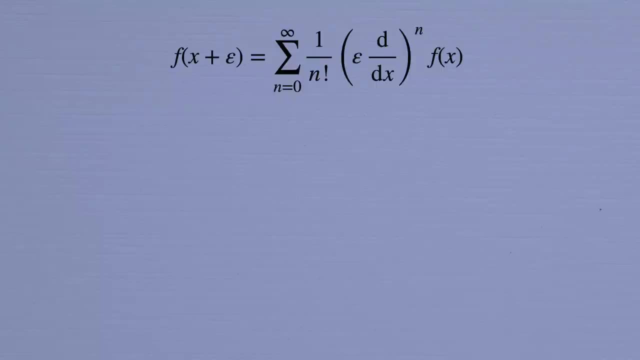 function f at a point that's shifted away from x by an amount epsilon. what we should do is take the function at the original point x and apply this special combination of derivatives, which is the sum of the derivatives, to it. But hang on a second, that might look familiar. 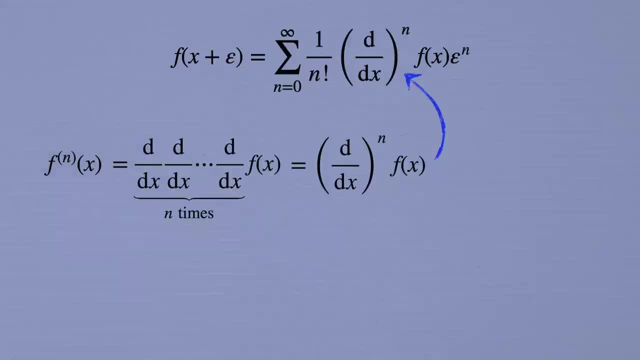 So far this doesn't look like a huge simplification, But now let's drag that epsilon to the n, to the left, inside the parentheses. Now this looks really interesting. It says that if we want to know the value of our function f at a point that's shifted. 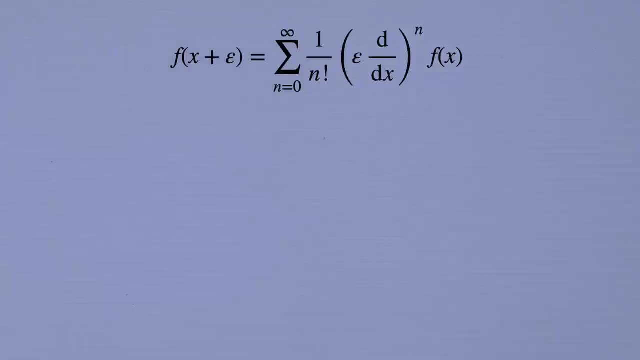 away from x by an amount epsilon. what we should do is take the function at the original point x and apply this special combination of derivatives to it. But hang on a second that might look familiar. Remember from a minute ago that the Taylor series we found for e to the z was one plus. 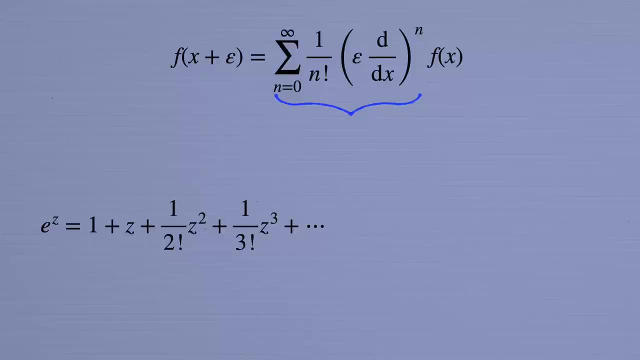 z plus one over two. factorial z squared plus one over three. factorial z cubed plus dot dot dot, Or in some notation, the sum of one over n. factorial z to the n. But that's exactly what this differential operator looks like. where z is this thing? 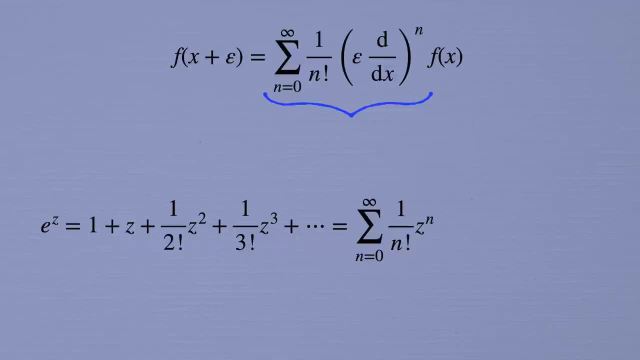 in parentheses- epsilon d by dx. Then this big sum of derivatives is nothing but e to the epsilon d by dx. And so what's the sum of the derivatives? So at least formally we can write: f of x plus epsilon equals e to the epsilon d by. 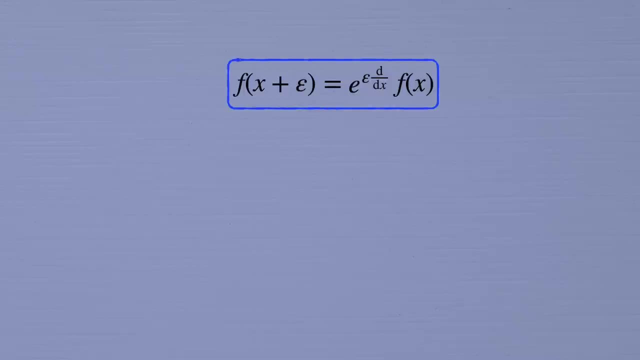 dx acting on f of x. This is the most compact, convenient and beautiful way of writing Taylor's formula. It neatly repackages the whole infinite sum over derivatives of f and powers of the displacement into a single operator, e to the epsilon d by dx acting on the function. 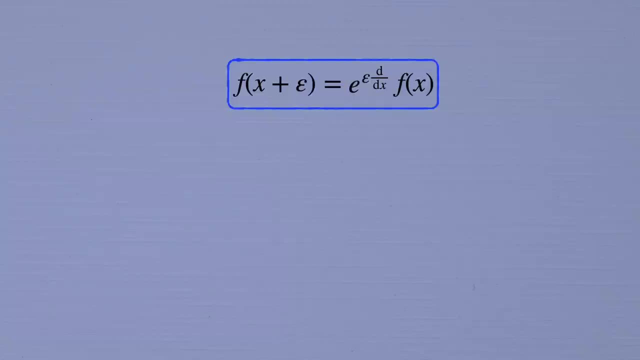 Just to make sure it's clear how this works, let's try applying it to a really simple function. f of x equals mx plus b. Obviously, the Taylor series for this one is really boring. It already is its own Taylor series. We expand out the exponential and get one plus epsilon times the first derivative plus. 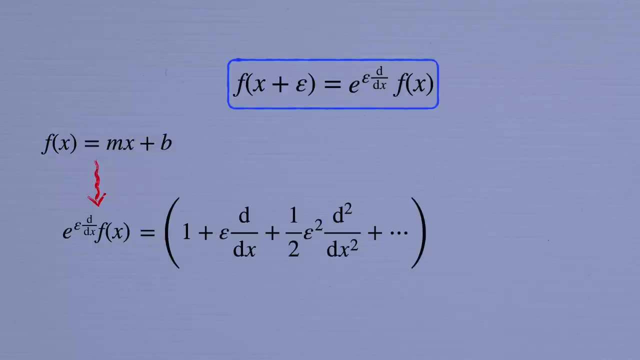 one-half epsilon squared times the second derivative and so on. Then all that acts on the function mx plus b. When we multiply out the one, we just get back mx plus b, And when the first derivative term acts, we get epsilon m. 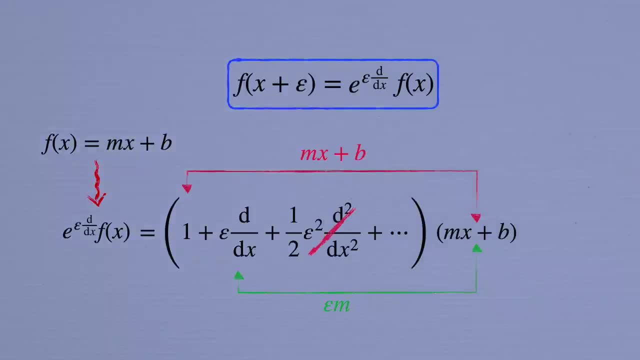 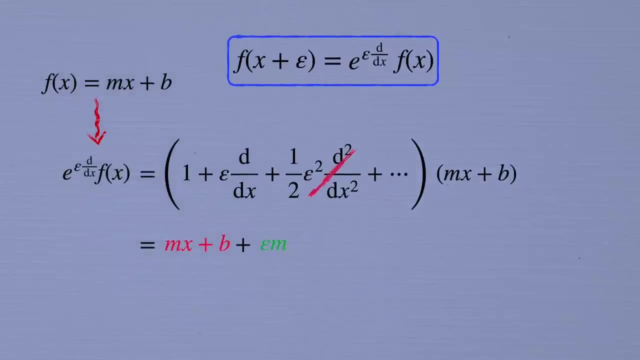 As for that second derivative and everything else, all that disappears, because when you take more than one derivative of a second derivative, you get epsilon m straight line, you get zero. So altogether we've got mx plus b plus epsilon m or equivalently. 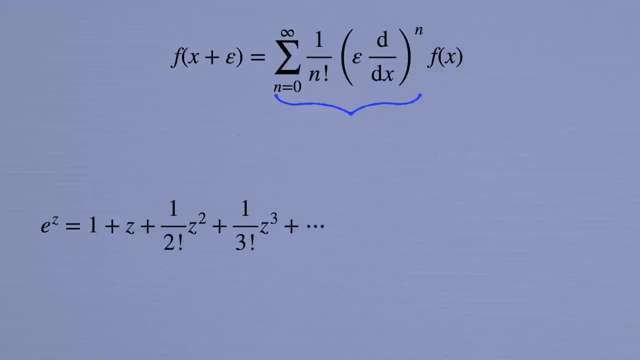 Remember from a minute ago that the Taylor series we found for e to the z was 1 plus z plus 1 over 2. factorial z squared plus 1 over 3. factorial z cubed plus dot dot dot, Or, in some notation, the sum of 1 over n. factorial z to the n. But that's exactly what this differential operator. 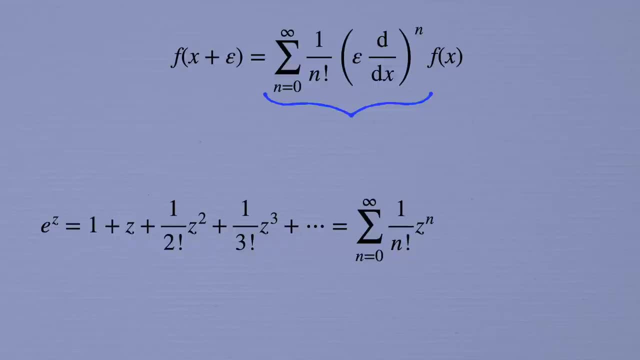 looks like where z is this thing in parentheses: epsilon d by dx. Then this big sum of derivatives is nothing but e to the epsilon d by dx, And so, at least formally, we can write: f of x plus epsilon equals e to the epsilon d by dx. acting on f of x. 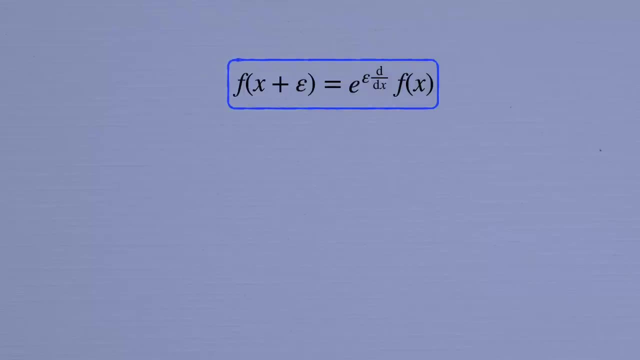 This is the most compact, convenient and beautiful way of writing Taylor's formula. It neatly repackages the whole infinite sum over derivatives of f and powers of the displacement into a single operator, e to the epsilon d by dx acting on the function. 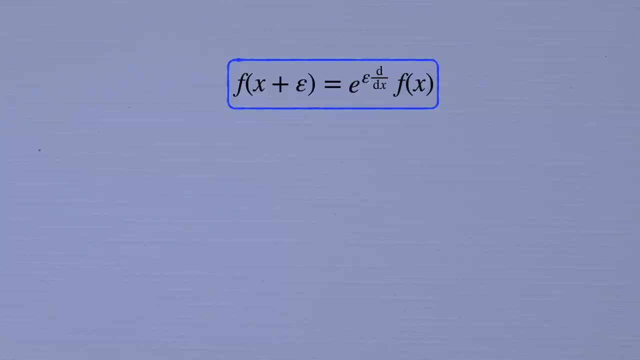 Just to make sure it's clear how this works, let's try applying it to a really simple function. f of x equals mx plus b. Obviously, the Taylor series for this one is going to be really boring. It already is its own Taylor series. We expand out the exponential and get 1 plus epsilon times, the. 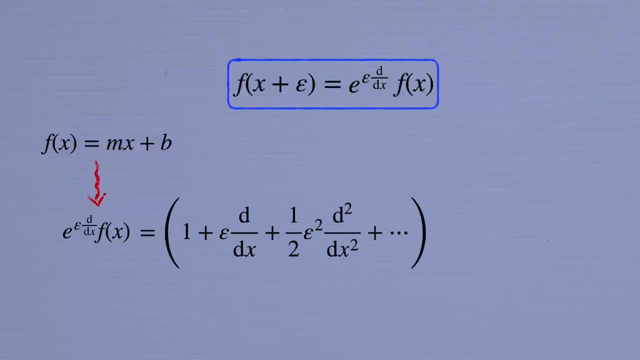 first derivative plus 1, half epsilon squared times the second derivative and so on. And then all that acts on the function mx plus b. When we multiply out the 1, we just get back mx plus b. And when the first derivative term acts, we get epsilon m. 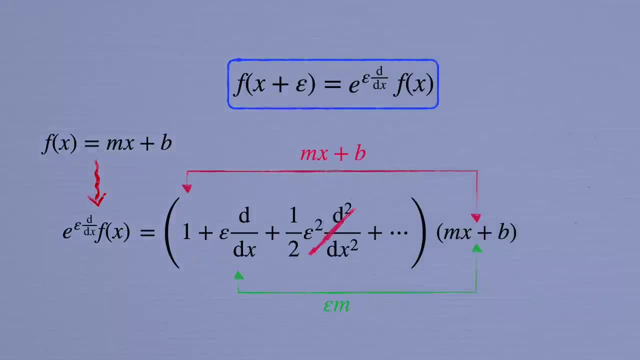 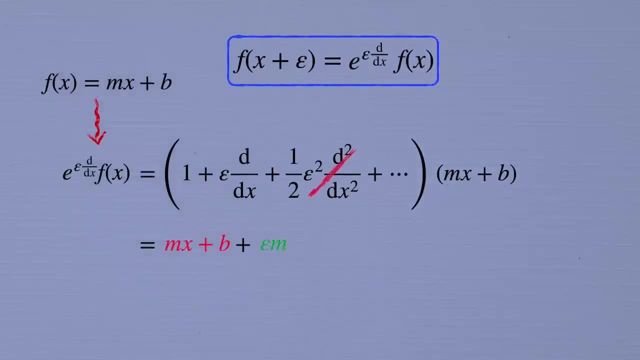 As for that second derivative and everything else, all that disappears, because when you take more than one derivative of a straight line, you get zero. So altogether we've got mx plus b plus epsilon m, or equivalently m times x plus epsilon plus b, which is precisely f of x plus epsilon. 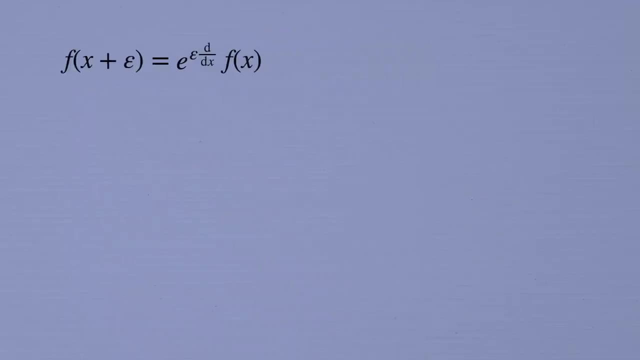 just as expected. One last beautiful thing about this way of writing Taylor's formula before we get to the physics: It makes the generalization to the multivariable Taylor expansion really straightforward. Say, we now have a function f of xyz, For example. 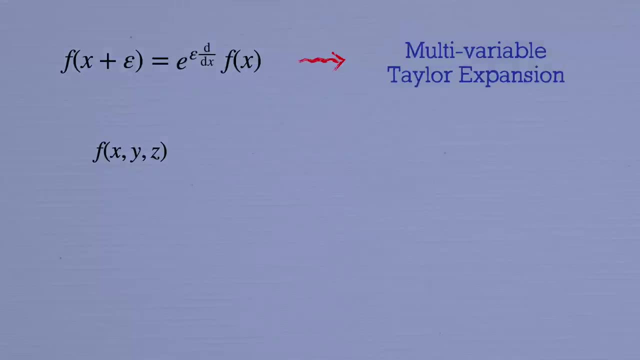 this might be the potential energy function of a particle moving around in three-dimensional space. Then what's the Taylor expansion of this? The most direct way to approach it is to expand, like before, with one variable at a time. If we apply the Taylor expansion just in x, we get f of x, still with y plus epsilon y. 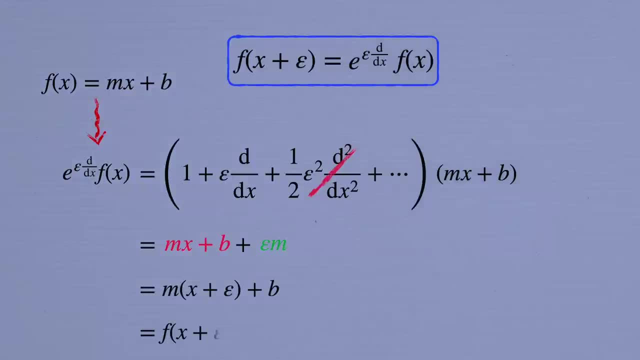 m times x plus epsilon plus b, which is precisely f of x plus epsilon, just as expected. One last beautiful thing about this way of writing Taylor's formula before we get to the physics: It makes the generalization to the multivariable Taylor expansion really. 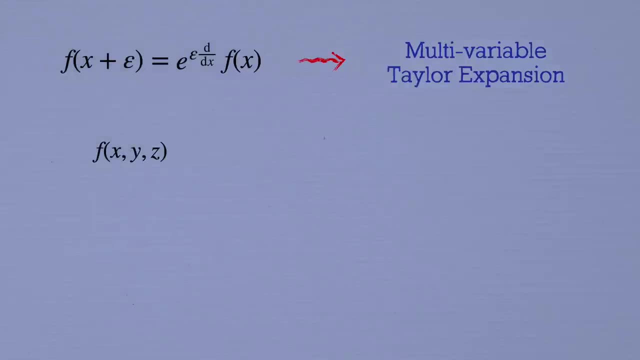 straightforward. Say we now have a function f of xyz, For example, this might be the potential energy function of a particle moving around in three dimensional space. Then what's the Taylor expansion of this? The most direct way to approach it is to expand, like before. 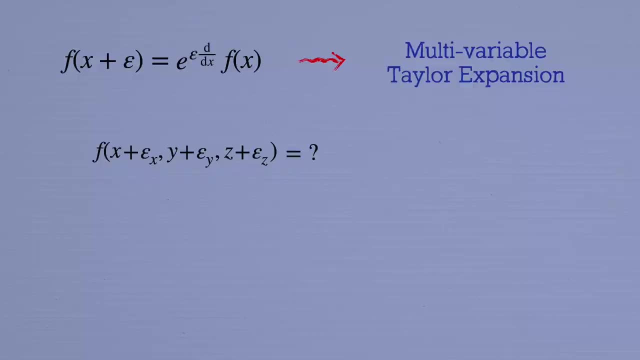 with one variable at a time. If we apply the Taylor expansion just in x, we get f of x, still with y plus epsilon y, z plus epsilon z plus epsilon x, d by dx of that plus half epsilon x squared times the second derivative with respect to x and so on, Where these 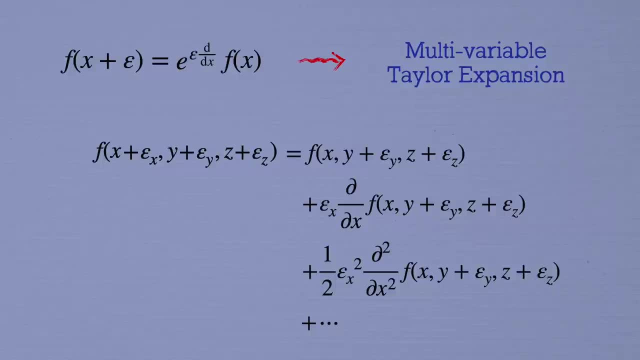 are now partial derivatives because f is a function of more than one variable. All that means is that we take the derivative of f with respect to x, like we would normally would, treating the other variables, y and z, as constants. But now we have to do the same. 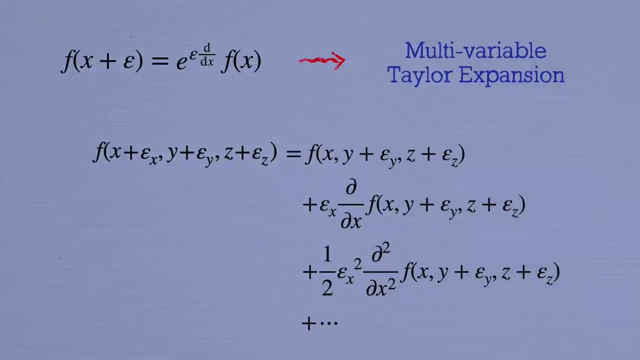 expansion over again in each of these terms for y and then again in each of those terms for z. It's a bit of a mess, But our exponential formula makes the whole thing incredibly simple. Let's write: our vector equals xyz for the position vector and epsilon vector equals. 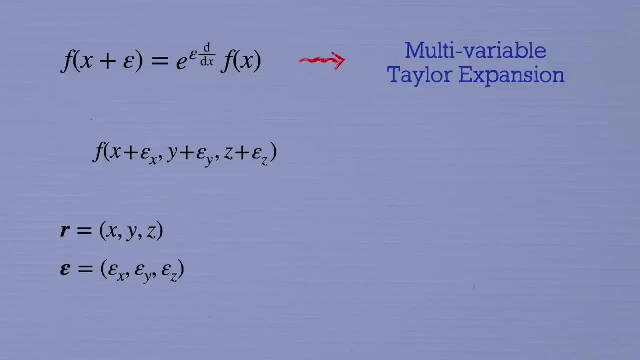 epsilon x, epsilon y and epsilon z for the position vector, the displacement vector. Then we're trying to tailor, expand f of r vector plus epsilon. All we need to do to generalize our original formula is to replace the epsilon d by dx. 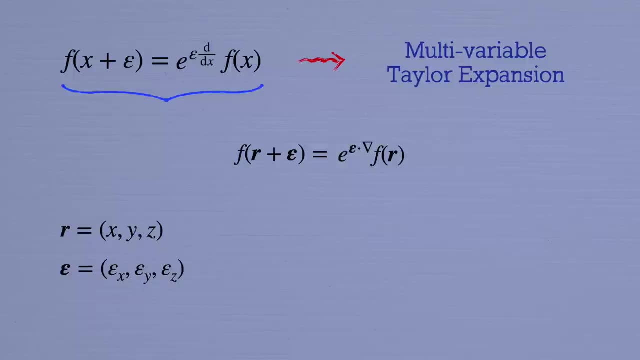 in the exponent with the dot product between epsilon vector and the quote unquote vector of partial derivatives, d by dx, d by dy, d by dz, which is usually denoted by this upside down triangle called del, And so this dot product just means epsilon x, d by dx plus. 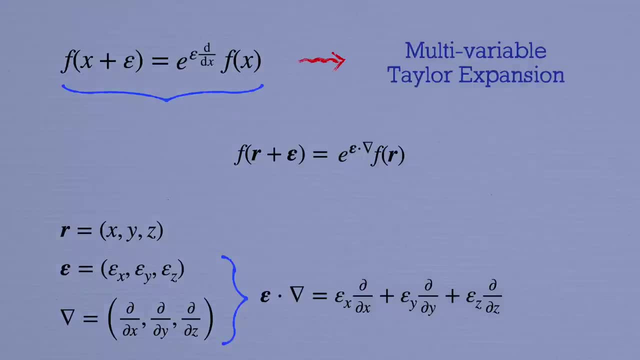 epsilon y- d by dy, plus epsilon z- d by dz. Then by combining the exponential formulas for the Taylor series in x, y and z, we get this beautiful compact formula for the Taylor expansion in three or any number of variables. Okay, that's enough math. Now let's put 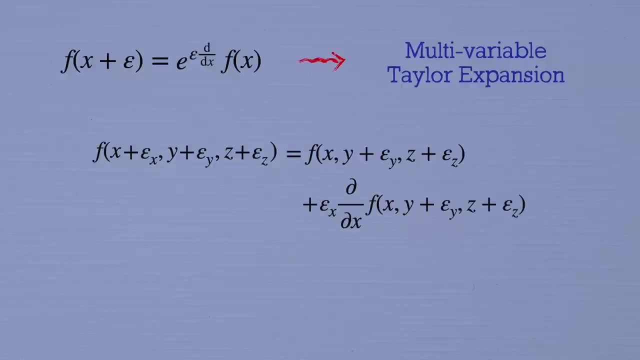 z plus epsilon z plus epsilon x, d, by the x of that plus half epsilon x squared times the second derivative with respect to x and so on, Where these are now partial derivatives because f is a function of more than one variable. All that means is that we take: 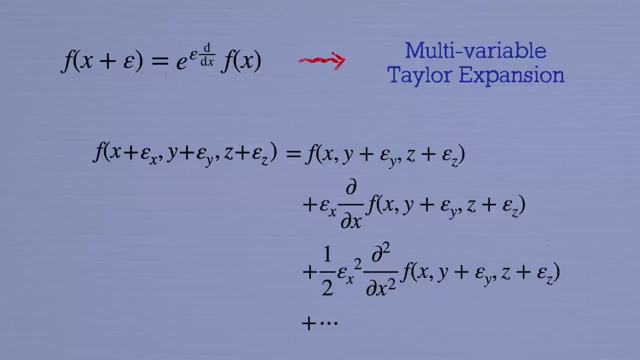 the derivative of f with respect to x, like we normally would, treating the other variables, y and z, as constants. But now we have to do the same expansion over again in each of these terms for y and then again in each of those terms for z. It's a bit of a mess, But our exponential formula 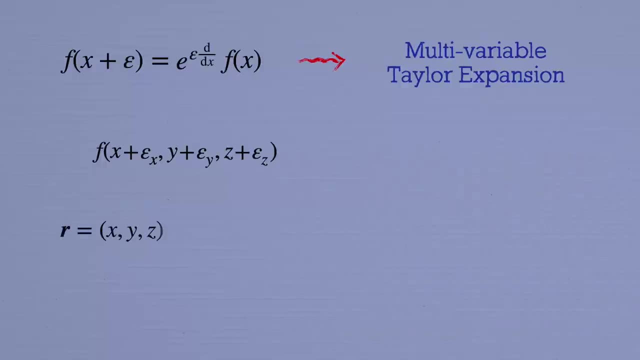 makes the whole thing incredibly simple. Let's write: r vector equals xyz for the position vector, and epsilon vector equals epsilon x, epsilon y, epsilon z for the displacement vector. Then for x, we're trying to Taylor expand f of r vector plus epsilon. All we need to do to generalize our. 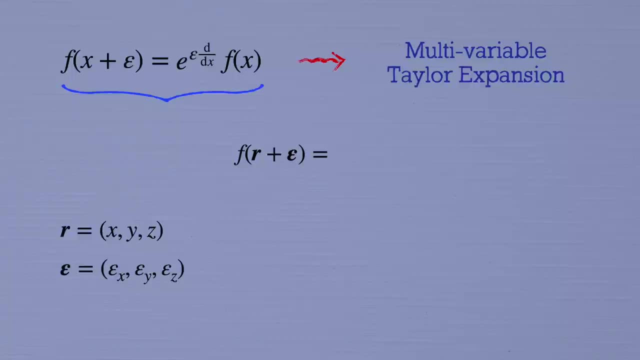 original formula is to replace the epsilon d by the x in the exponent with the dot, product between epsilon vector and the quote unquote vector of partial derivatives, d by the x, d by the y, d by the z, which is usually denoted by this upside down triangle called del, And so 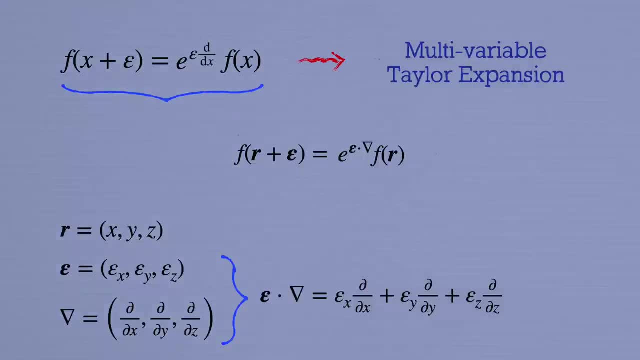 this dot product just means epsilon x- d by the x plus epsilon y- d by the y plus epsilon z- d by the z. Then by combining the exponential formulas for the Taylor series in x, y and z we get this beautiful compact formula for the Taylor expansion in three or any number of. 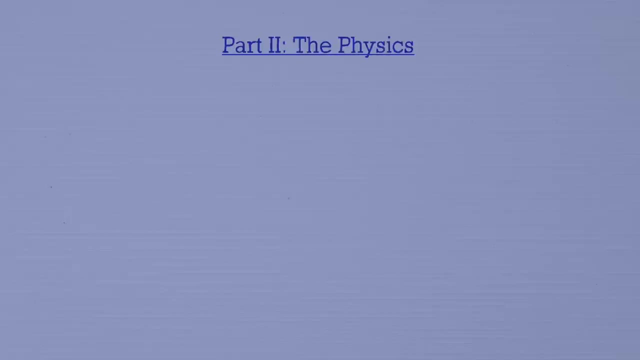 variables. Okay, that's enough math. Now let's put it to work with part two, the physics. I promised to show you three applications. Number one: how to make the complicated equations that we often need to solve in physics simpler by studying special linearized limits. Number two: the non-relativistic. 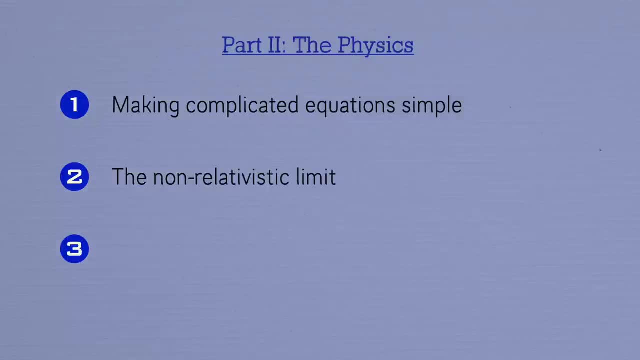 limit of Einstein's energy value. Number three, the non-relativistic limit of Einstein's energy formula and how it contributes to the fine structure of the hydrogen atom. And number three, the definition of the momentum operator in quantum mechanics. Let's go one by one Again. 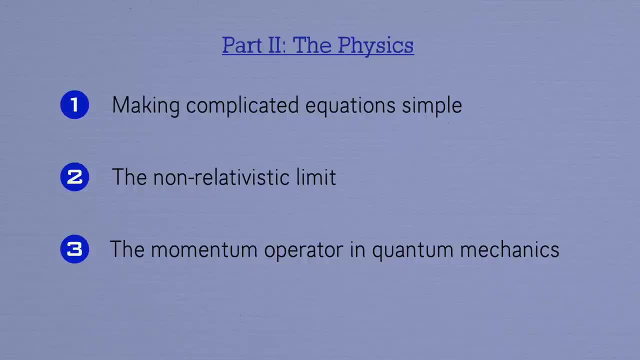 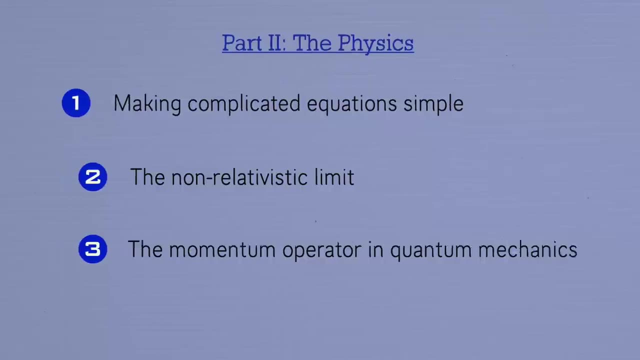 you don't necessarily need to know anything going in about relativity or quantum mechanics. The point is just to get a taste of how Taylor's formula appears in several very different areas of physics, Starting with number one: making complicated problems simple, The basic procedure. 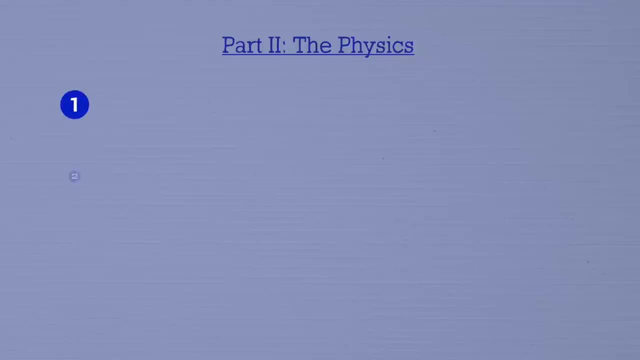 it to work. with part two, the physics, I promised to show you three applications. Number one: how to make the complicated equations that we often need to solve in physics simpler by studying special linearized limits. Number two: the nonrelativistic limit of Einstein's energy formula and how it contributes to the 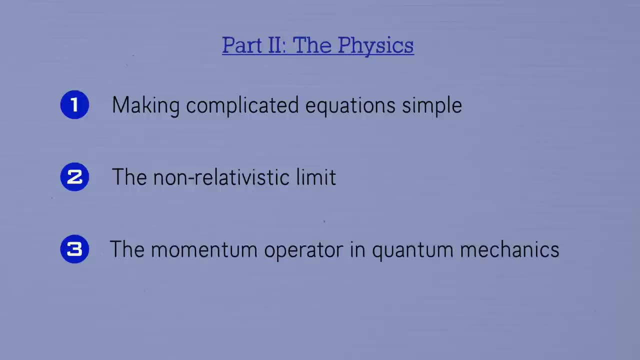 fine structure of the hydrogen atom. And number three, the definition of the momentum operator in quantum mechanics. Let's go one by one. Again, you don't necessarily need to know anything going in about relativity or quantum mechanics. The point is just to get a taste. 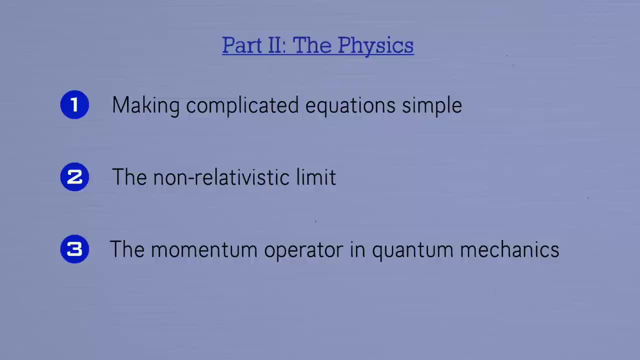 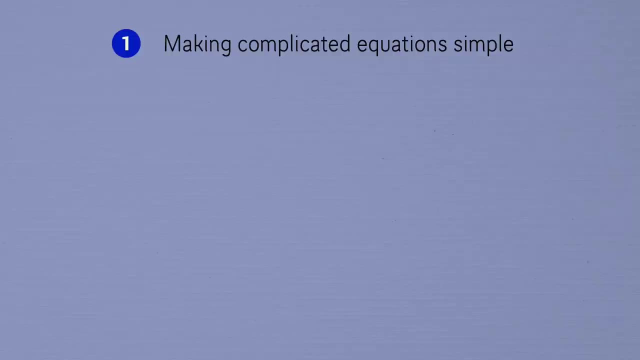 of how Taylor's formula appears in several very different areas of physics, Starting with number one: making complicated problems simple. The basic procedure to solve a problem in quantum mechanics is to write down all the forces on a particle and then add them up and write: F equals ma and then solve this equation for the position of the particle. 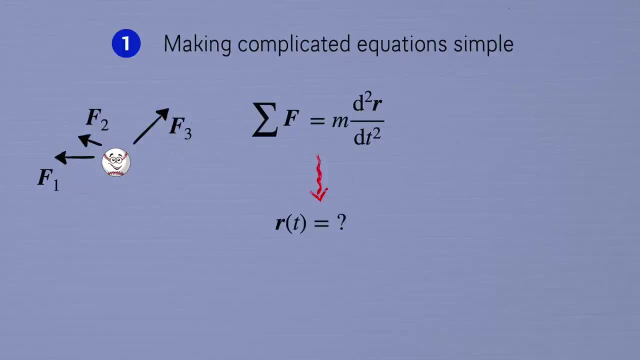 as a function of time, That's easier said than done, though, Especially the last step, solving F equals ma- because for all but the simplest systems, this equation quickly becomes too hard to solve. exactly, F equals ma is a differential equation, which just means 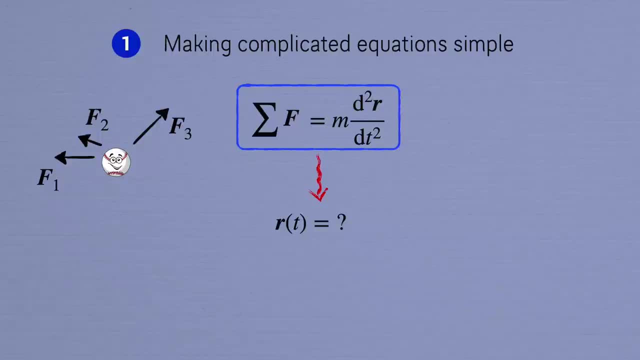 that it contains derivatives of the function that you're trying to solve for R of t. in this case, F equals ma and R of t are much harder to solve than the algebraic equations that we all first learn about in middle school and high school. A simple example that I've 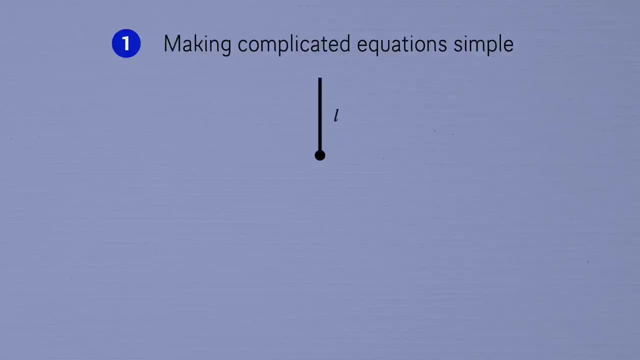 told you about in a few past videos is the pendulum. When solving for the motion of a pendulum, the main force we're interested in is the component of gravity that points along the tangent direction to the circle where the particle is constrained to move. 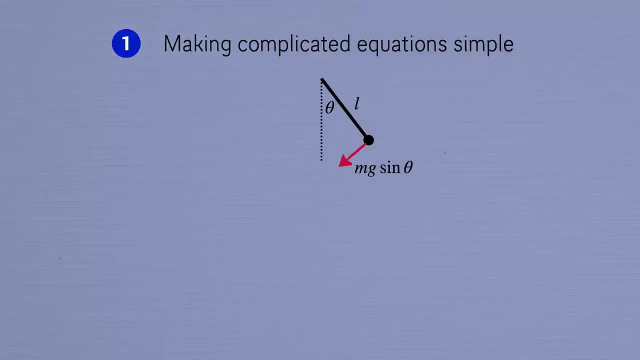 That's given by mg sine of theta, where theta is the angle that the pendulum makes with the vertical axis. Like I showed you in the very first video I posted here on the channel, This ma equation for theta can be written, after a little simplifying, as the second, 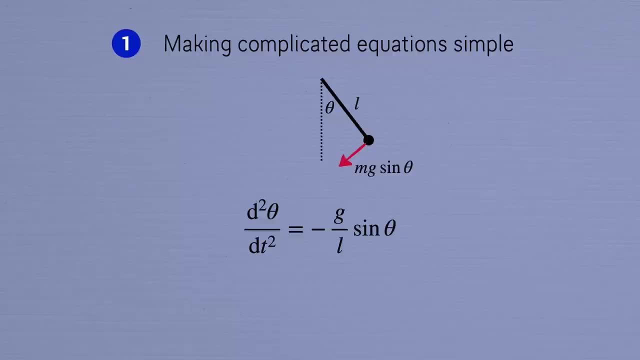 derivative of theta with respect to time equals minus g over l sine of theta. Simple as this physical setup looks, this equation is already very complicated because of this factor of sine of theta. It makes it what we call a non-linear differential equation, which can be very nasty to try to solve. 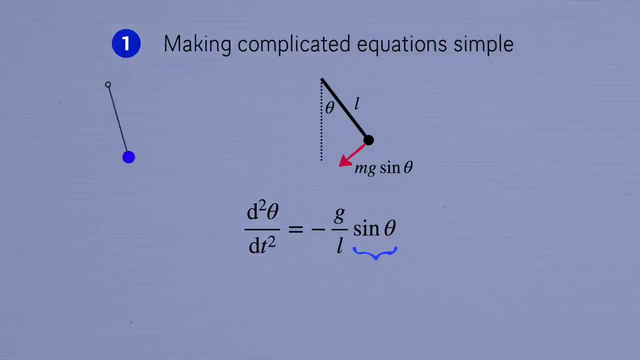 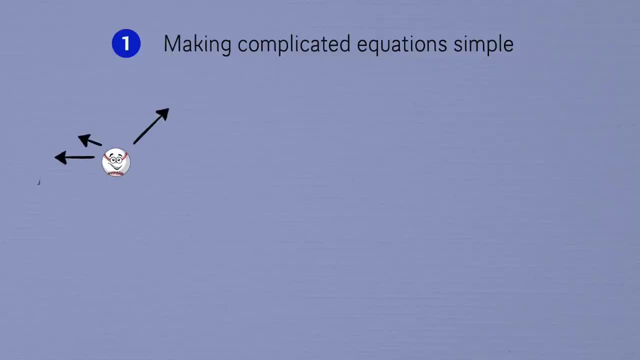 to solve a problem in classical mechanics is to write down all the forces on a particle and then add them up and write: f equals ma and then solve this equation for the position of the particle as a function of time. That's easier said than done, though, Especially the last step. 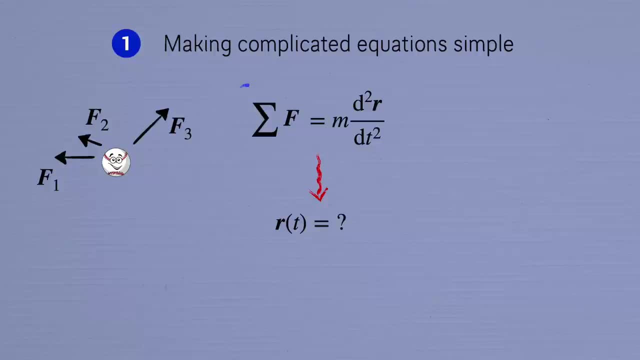 solving f equals ma, Because for all but the simplest systems, this equation quickly becomes too hard to solve. exactly, F equals ma is a differential equation, which just means that it contains derivatives of the function that you're trying to solve, for r, of t in this case, And differential equations are much harder to solve than algebraic equations. 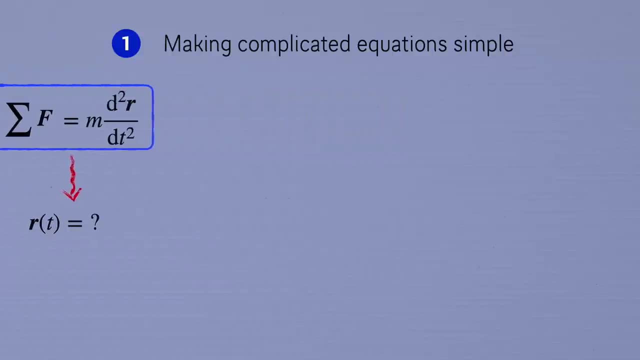 that we all first learn about in middle school and high school. A simple example that I've told you about in a few past videos is the pendulum. When solving for the motion of a pendulum, the main force we're interested in is the component of gravity that points along the 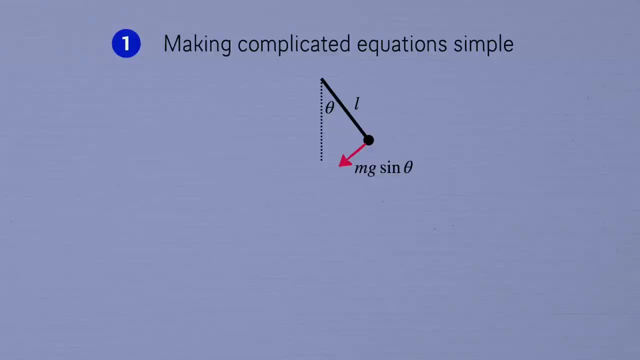 tangent direction to the circle where the particle is constrained to move. That's given by mg sine of theta, where theta is the angle that the pendulum makes with the vertical axis, like I showed you in the very first video I posted here on the channel. Then the f equals ma equation for theta can be: 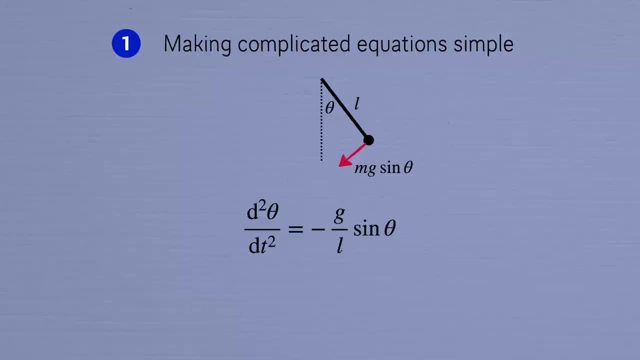 written as the second derivative of theta with respect to time equals minus g over l sine of theta. Simple as this physical setup looks, this equation is already very complicated because of this factor of sine of theta. It makes it what we call a non-linear differential equation, which can 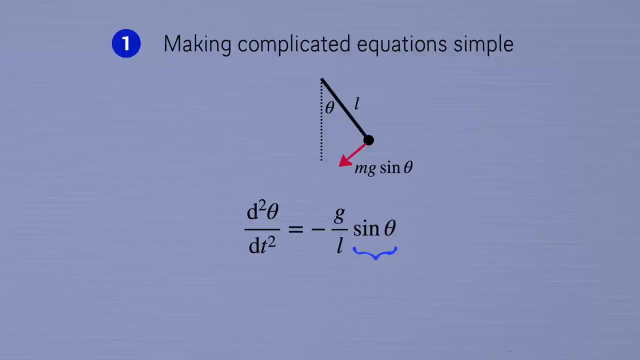 be very nasty to try to solve. On the other hand, when theta is small, you can picture a pendulum gently rocking back and forth like a grandfather clock, and that motion certainly doesn't seem very complicated. Is it possible, then, that we can simplify this equation when theta is? 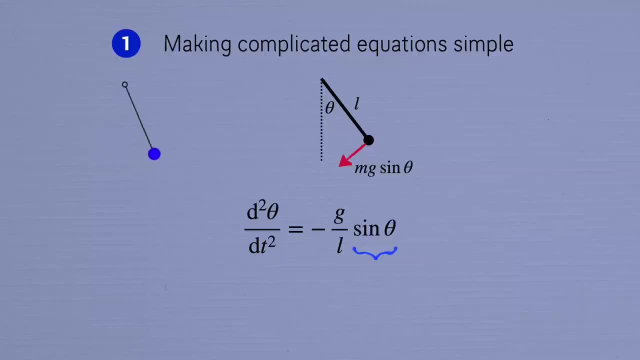 relatively small. The Taylor series lets us do just that, Like we worked out before. the Taylor series for sine is theta minus 1 over 3 factorial theta, cubed plus 1 over 5 factorial theta to the fifth, plus dot, dot, dot. Then for tiny thetas we can apply the small angle approximation. 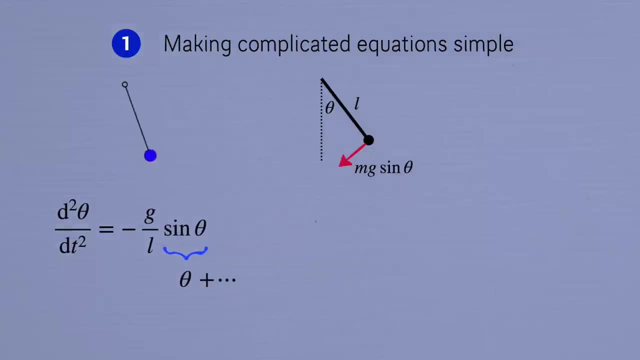 like we saw before. Then this complicated f equals ma equation becomes vastly simpler. There's no sine theta factor here anymore, making this equation complicated and non-linear. By applying the Taylor series, we've been able to memorize the differential equation, To turn it into a problem we can solve. 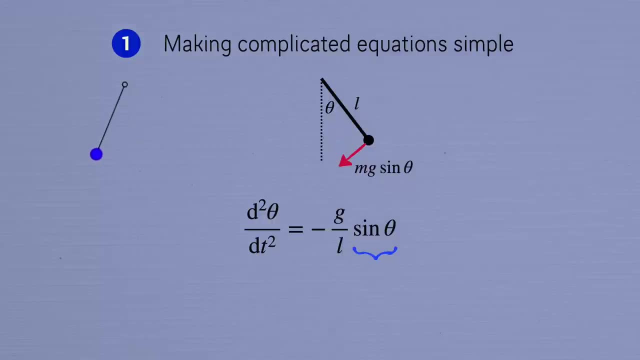 Is it possible, then, That we can simplify this equation when theta is relatively small? The Taylor Series. let's us do just that, Like we worked out before. the Taylor Series for sine is theta minus one over three. factorial theta cubed plus one over five. factorial theta to the fifth plus dot, dot, dot. 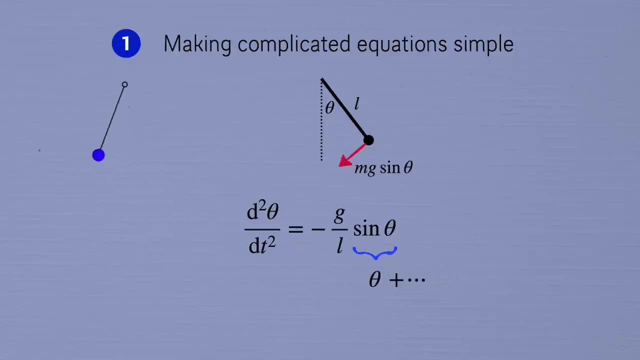 Then for tiny thetas we can apply the small angle approximation like we saw before. Then this complicated F equals ma equation becomes vastly simpler. There's no sine theta factor here anymore, making this equation complicated and nonlinear. By applying the Taylor series we've been able to linearize the differential equation. 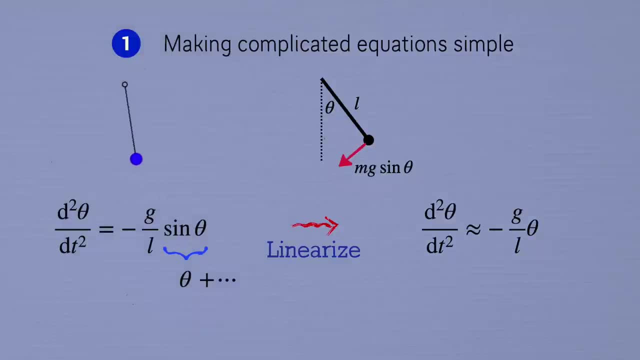 To turn it into a problem we can solve much more easily in this special case, when the pendulum isn't too far away from equilibrium. This is just the equation of a simple harmonic oscillator, now like a mass on a spring, And the general solution is a sum of sines and cosines with angular frequency square. 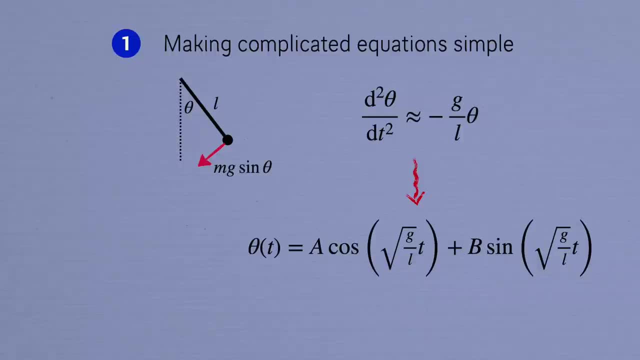 root g over L, So the pendulum indeed rocks gently back and forth from side to side. If you've been watching my recent videos and all this looks familiar, it's no accident. I told you a few weeks ago about how the first thing we should do in any physics problem 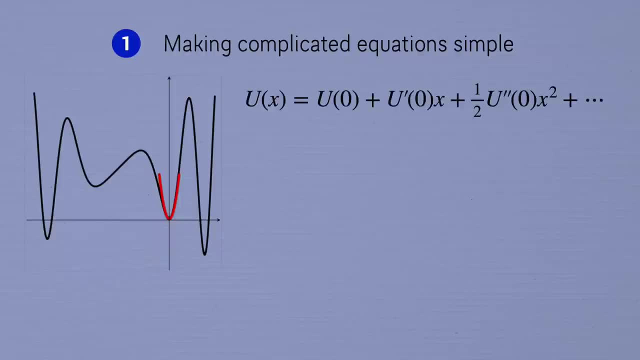 is expand the potential energy function around a stable equilibrium point in a Taylor series: u of x equals u of zero, plus u prime of zero times x plus half u double prime of zero, x squared plus dot dot dot, Where I chose my coordinates here so that the equilibrium point is at x equals zero. 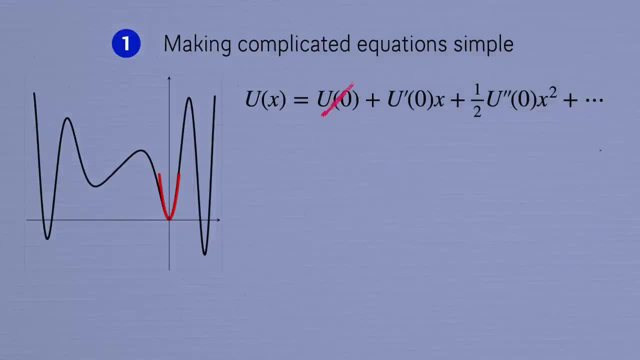 The first term, u of zero is just a constant, and that doesn't matter. You're always allowed to change what you call the ground level of your potential energy function and shift this constant away. The second term, meanwhile, vanishes because we've chosen to expand around a minimum of 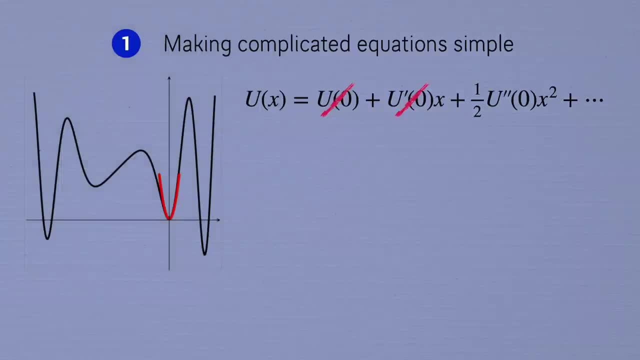 the potential where u prime is equal to zero. So typically the first interesting term in the Taylor expansion of a potential around equilibrium is the quadratic term, which is just like the potential energy, one half kx squared of a block on a spring. 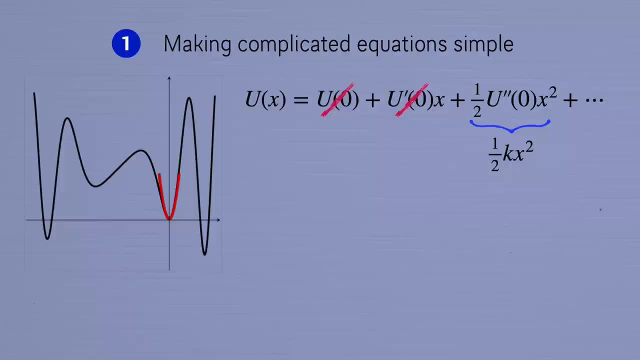 This is why systems oscillate back and forth around their equilibrium position. I'll put a link in the description. As for the force that's related to the potential energy, by f equals minus du by dx, And therefore the Taylor series for the force on a particle near equilibrium starts with: 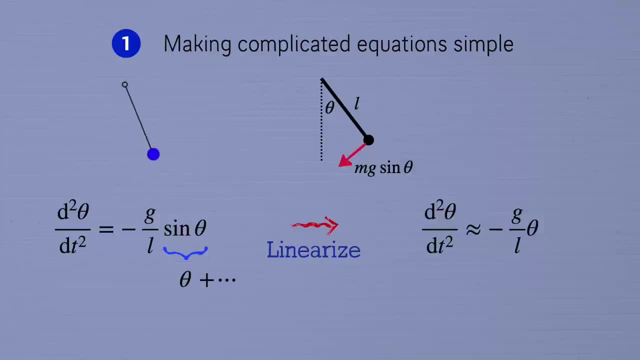 much more easily in this special case, when the pendulum isn't too far away from equilibrium. This is just the equation of a simple harmonic oscillator, now like a mass on a spring, and the general solution is a sum of sines and cosines with angular frequency square root g over. 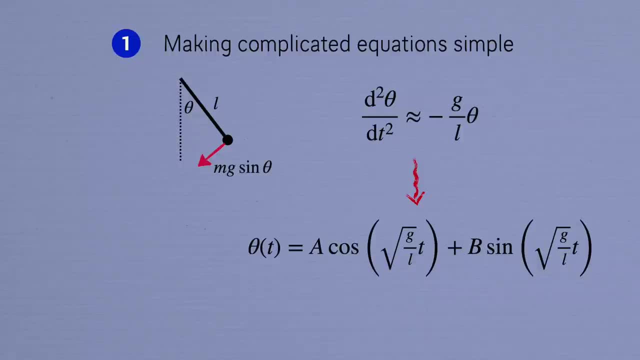 L. So the pendulum indeed rocks gently back and forth from side to side. If you've been watching my recent videos and all this looks familiar, it's no accident. I told you a few weeks ago about how the first thing we should do when we want to solve a problem is to solve a problem. 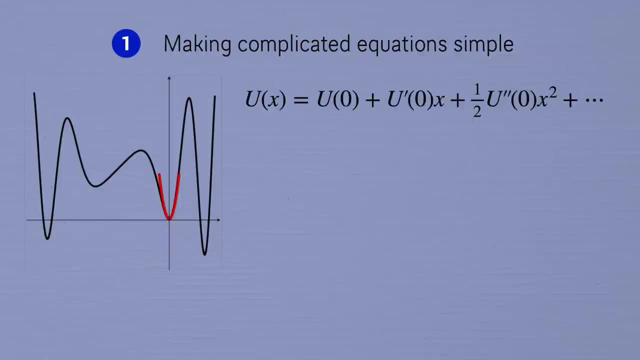 The first thing we should do in any physics problem is expand the potential energy function around a stable equilibrium point. in a Taylor series, u of x equals u of zero plus u. prime of zero times x plus half u double prime of zero x squared plus dot dot dot, Where I chose my 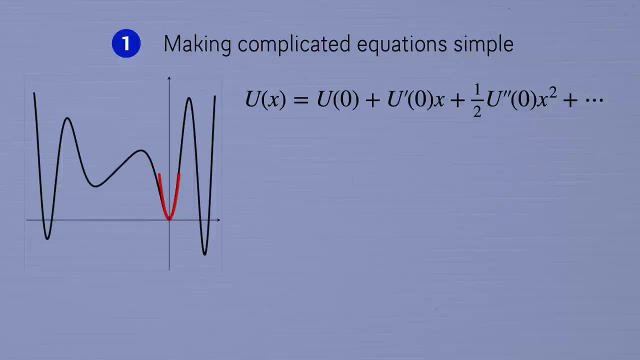 coordinates here, so that the equilibrium point is at: x equals zero. The first term: u of zero is just a constant and that doesn't matter. You're always allowed to change what you call the ground level of your potential energy function and shift this constant away. The second term: 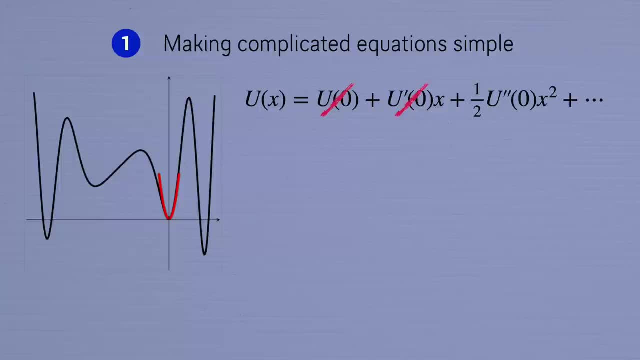 u of x equals u of zero vanishes because we've chosen to expand around a minimum of the potential where u prime is equal to zero. So typically the first interesting term in the Taylor expansion of a potential around equilibrium is the quadratic term, which is just like the potential energy. 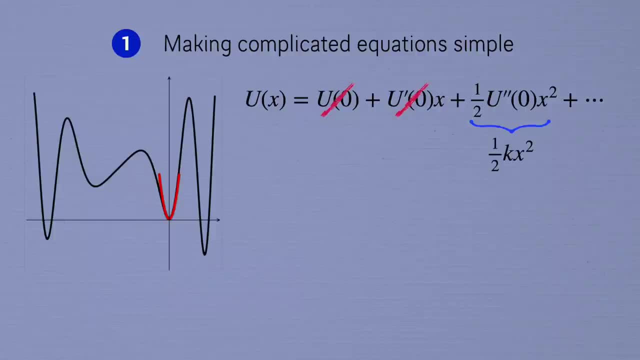 one half kx squared of a block on a spring. This is why systems oscillate back and forth around their equilibrium position. I'll put a link in the description to the video where I talked all about this. As for the force that's related to the potential energy by, f equals minus. 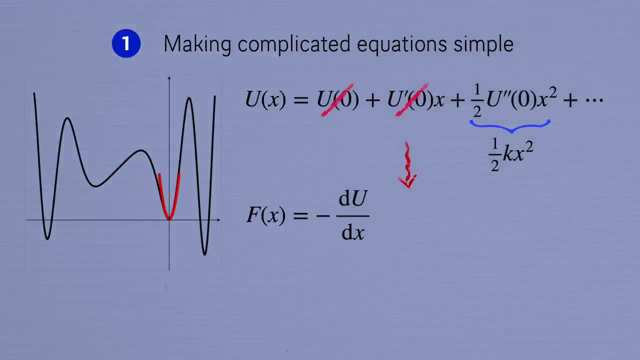 kx, And therefore the Taylor series for the force on a particle near equilibrium starts with: f equals minus u, double prime of zero times x. Again, just like the spring force minus kx, In particular, the force is linear. So the trick I taught you a couple of weeks ago about the simple 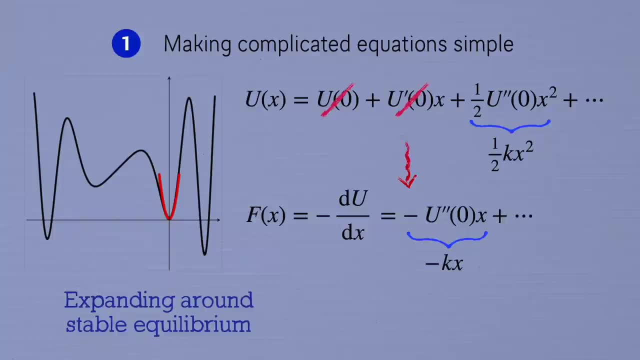 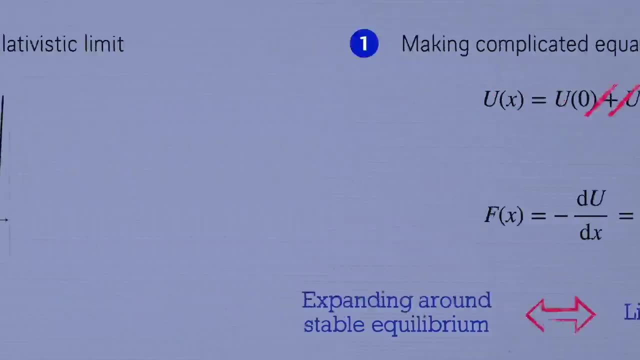 harmonic motion you discover when you expand the potential energy around a stable equilibrium is secretly the same thing as linearizing the f equals ma equation. Next up, let's look at the Newtonian limit of Einstein's theory of special relativity. In Newtonian mechanics, a free 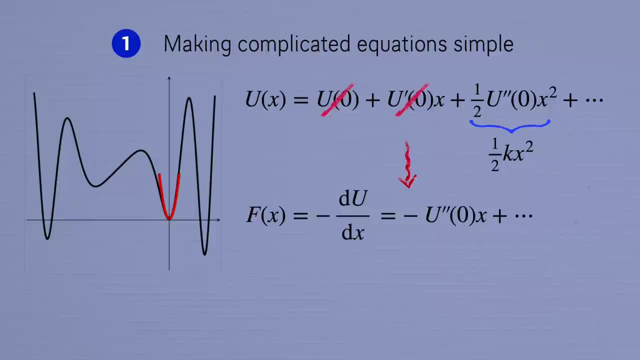 f equals minus u, double prime of zero times x. Again, just like the spring force minus kx, In particular, the force is linear. So the trick I taught you a couple of weeks ago about the simple harmonic motion you discover when you expand the potential energy around a stable equilibrium point is that you can: 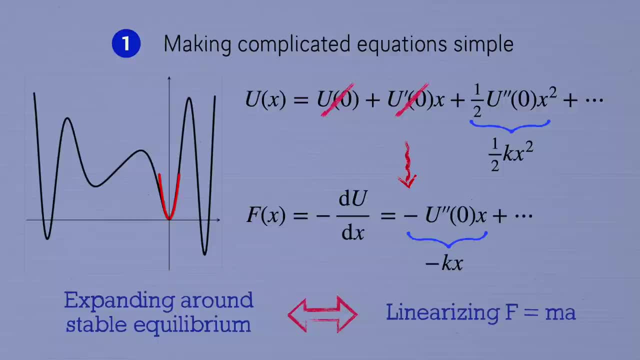 expand the potential energy around a spring, And so you grow up to a setting of 2 pi times x a spring. That's the t squared, on the other hand, the rise and fall of this spring. So the result is the same as the initial limit. 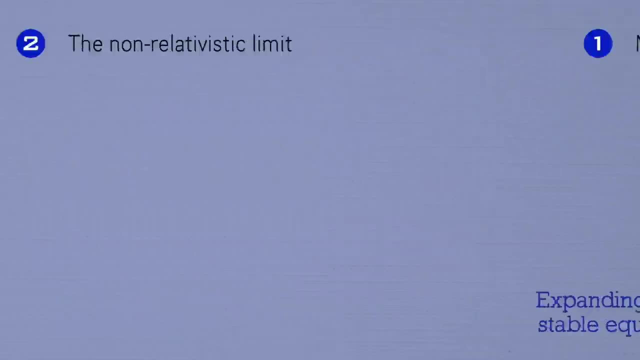 You know the secret to that which you can find in your equation. If you're interested in the equation you're talking about, you can look at the Newton's limit. The 관심 element is equal to the linearity of the f equals ma equation. 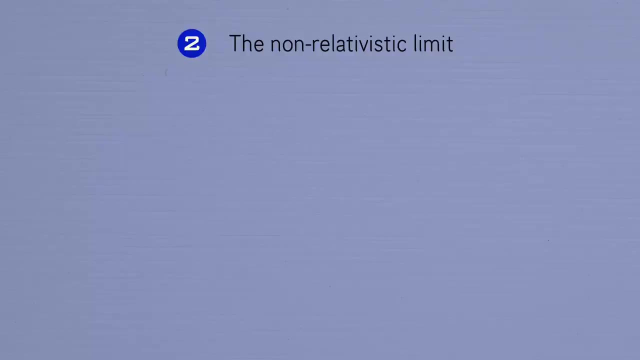 Now let's look at the Newtonian limit of Einstein's theory of special relativity. In Newtonian mechanics a free particle has kinetic energy one half mv squared. Alternatively, if we plug in the momentum p equals mv, we can write the same as p squared. 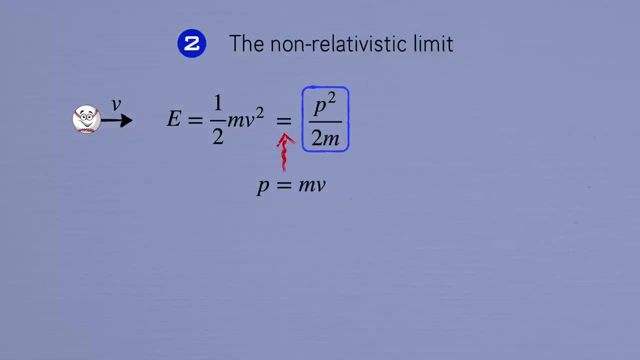 over 2m. This is the energy of a non-relativistic free particle. U is equal to u square, u squared, u squared. What does that mean? particle isn't moving very fast compared to the speed of light. When particles do approach. 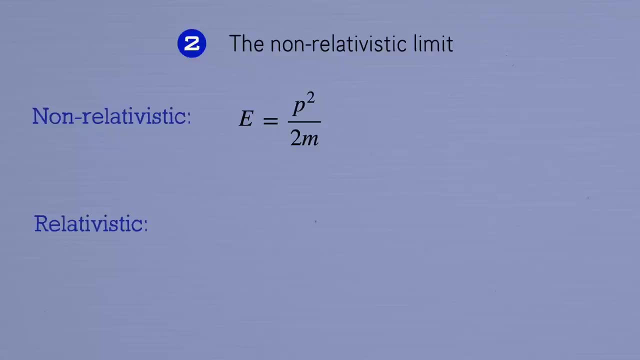 the speed of light, some weird and wild things happen that were discovered by Einstein a hundred and some years ago when he wrote down his special theory of relativity. In special relativity, the energy of a free particle of mass m and momentum p is given. 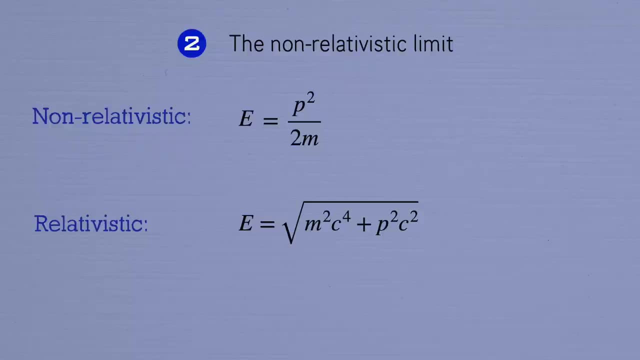 by this new formula, the square root of m squared c to the 4 plus p squared c, squared where c is the speed of light. You've seen this before, even if you've never studied special relativity, because if the particle is at rest, so that p equals zero, we get. 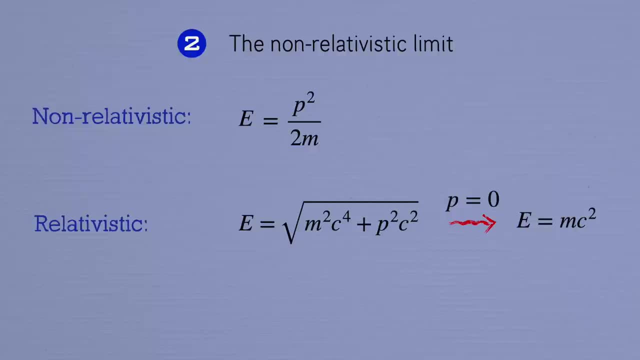 e equals mc squared, which might be the most famous equation in physics, But when the particle is moving, we need this more general formula, including the contribution from the momentum. This formula holds even if the speed of the particle approaches the speed of light, But on the other hand, we know what the energy is supposed to be when. 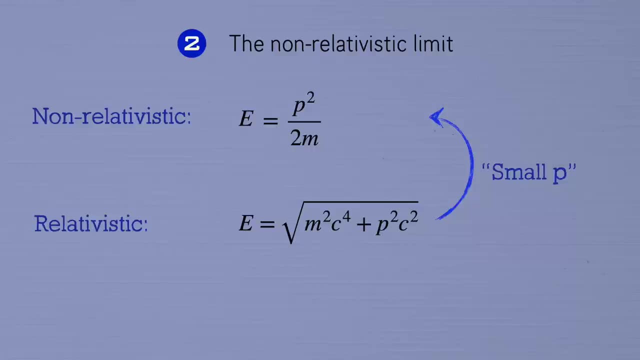 p is small. So how do we see that Einstein's formula correctly reproduces Newton's formula for a slow moving particle? The idea is, of course, to apply the Taylor expansion of Einstein's energy when p is small. Let's first of all pull this factor of m squared c to the 4 outside the square. 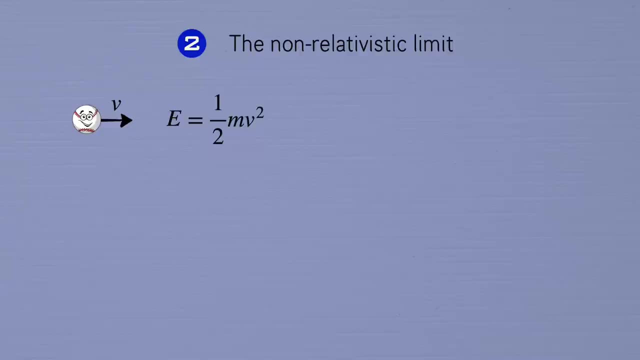 particle has kinetic energy one half mv squared. Alternatively, if we plug in the momentum, p equals mv, we can write the same thing as p squared over 2m. This is the energy of a non-relativistic free particle with momentum p. Non-relativistic means that the particle isn't moving very fast compared. 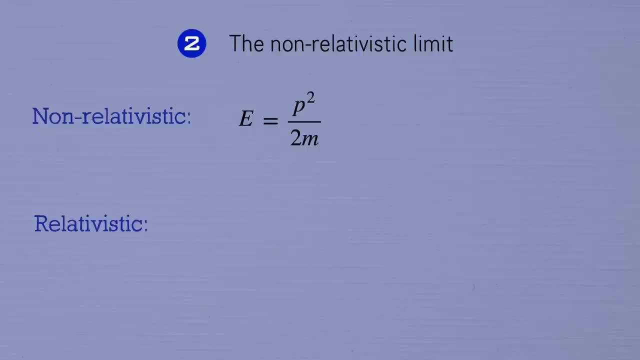 to the speed of light. When particles do approach the speed of light, some weird and wild things happen that we're just going to see in the next video discovered by Einstein a hundred and some years ago when he wrote down his special theory of relativity. 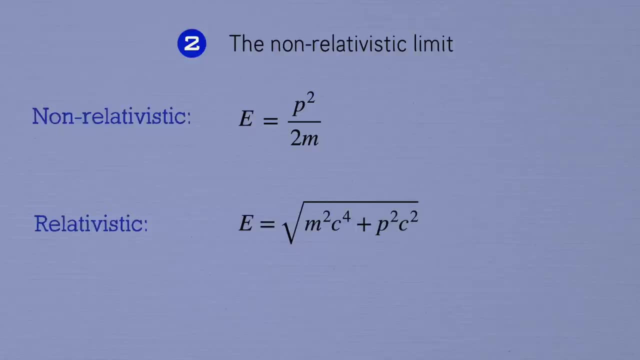 In special relativity, the energy of a free particle of mass m and momentum p is given by this new formula, the square root of m squared c to the 4 plus p squared c, squared where c is the speed of light. You've seen this before, even if you've never studied special relativity, because 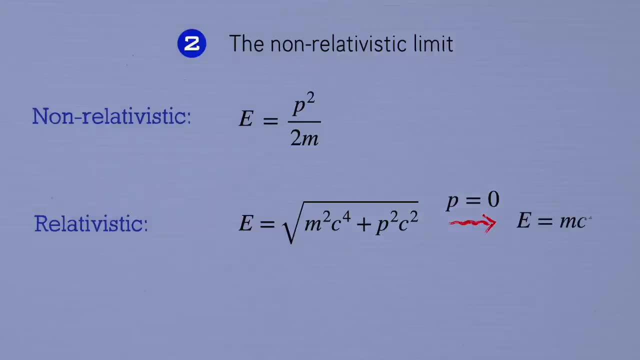 if the particle is at rest, so that p equals zero, we get e equals mc squared, which might be the most famous equation in physics. But when the particle is moving, we need this more general formula, including the contribution from the momentum. This formula holds even if the speed of the particle approaches the speed of light. 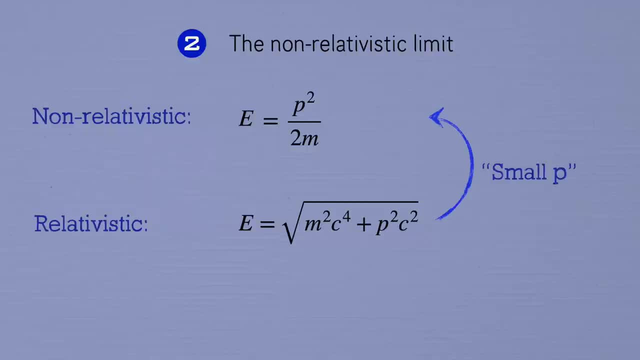 But on the other hand we know what the energy is supposed to be when p is small. So how do we see that Einstein's formula correctly reproduces Newton's formula for a slow moving particle? The idea is, of course, to apply the Taylor expansion of Einstein's energy when p is. 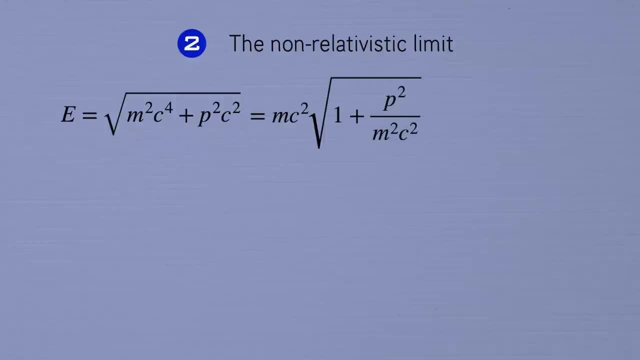 small. Let's first of all pull this factor of m squared c to the 4 outside the square root. Then we can write the whole thing like this: This makes it clear that what we want to do here is compute the Taylor series for f of. 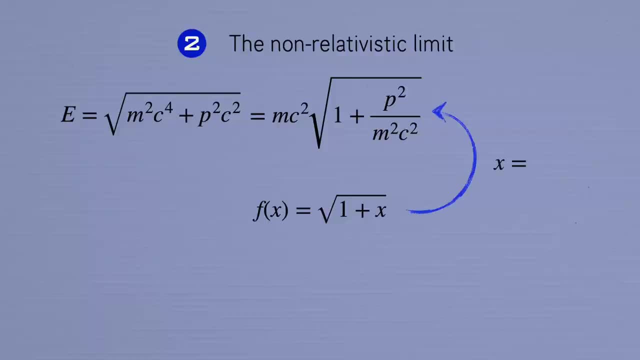 x equals 1 plus x square root. when x equals p squared over m squared c, squared is small. Actually, this kind of Taylor series shows up so often in physics that it's worth writing down the slightly more general case for f of x equals 1 plus x to some power q. 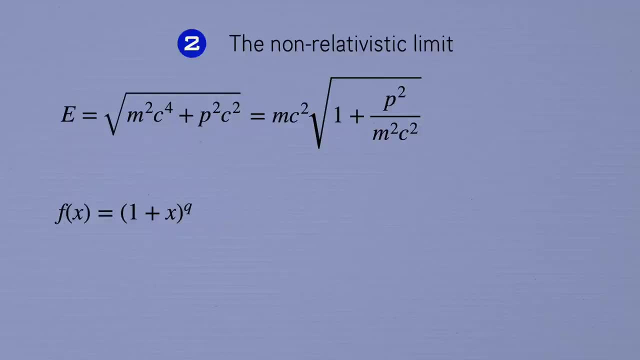 Our current case with the square root would be q equals half. I'll let you work out the first few terms of this Taylor series for yourself. for practice, I also go through the details. I get f of x equals 1 plus qx plus half q. q minus 1 times x squared. 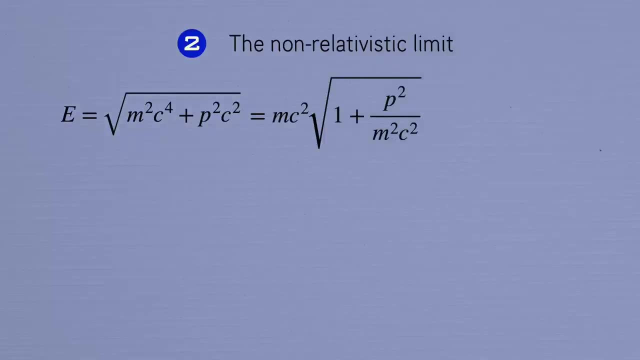 root. Then we can write the whole thing like this: This makes it clear that what we want to do here is compute the Taylor series for f of x equals 1 plus x square root. when x equals p squared over, m squared, c squared is small. Actually, this kind of Taylor series. 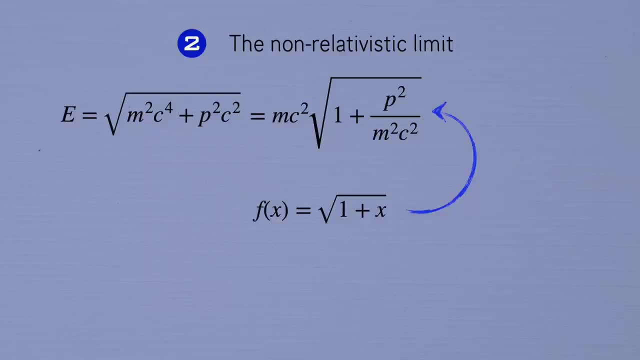 shows up so often in physics that it's worth writing down the slightly more general case for f of x equals 1 plus x. Our current case with the square root would be: q equals half. I'll let you work out the first few terms of this Taylor series for yourself, for practice. I also go through the 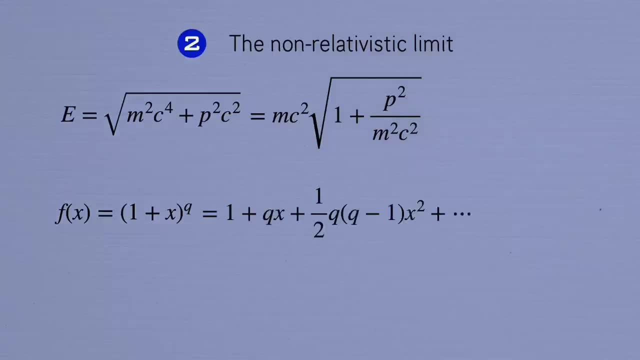 details in the notes. I get: f of x equals 1 plus qx plus half, q times x squared. The first pair of terms here is again a very useful approximation that comes up a lot in physics. Now back to the relativistic energy. We just plug in: q equals half and x equals p squared. 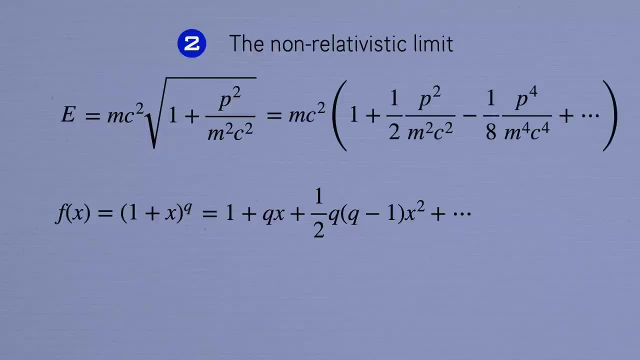 over m squared c squared, Then here's what we get. And if we multiply through by the mc squared, here's where we end up. e equals mc squared plus p squared over 2m, minus p to the 4 over 8m cubed c squared. 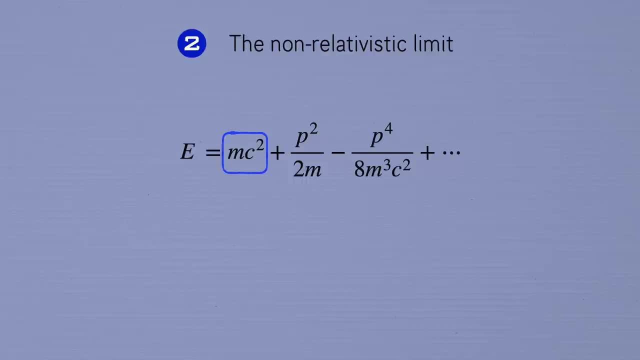 plus the higher powers of p. The first term is: e equals mc, squared again. That's what we get by evaluating the energy of a particle at rest in relativity. It doesn't have a direct analog in Newtonian mechanics, But on the other hand it's just a constant, And you're always free to add a constant to. 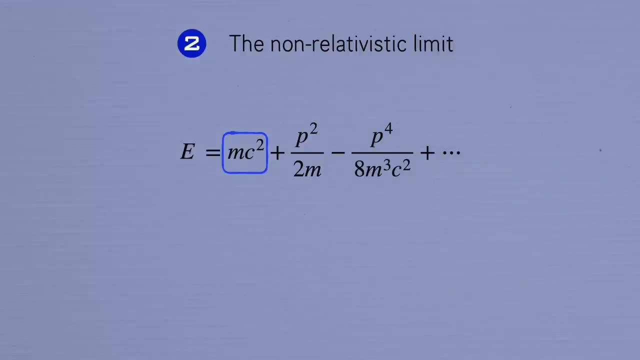 the total energy in Newtonian mechanics without changing the value of that constant. That's what we get. As for the second term, there we see how the Taylor series reproduces precisely the kinetic energy that we expect in Newtonian mechanics. Actually, I'm being slightly sloppy here, because the definition of the momentum p actually 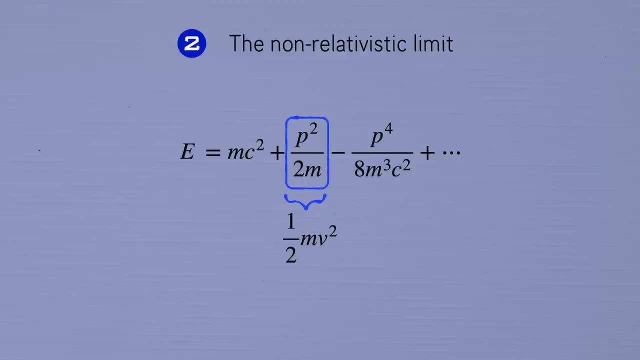 gets modified in relativity And we should really Taylor expand that as well. But in the non-relativistic limit we of course get back the Newtonian momentum p equals mv. But what about this next term in the Taylor series that goes like p to the 4?? What are we supposed to make of that? The point is that the Newtonian momentum is actually a little bit complicated because we can complement something else. but we can also make the Newtonian momentum harder. What about the r-term in the Taylor series that goes like p to the 4?? What are we supposed? 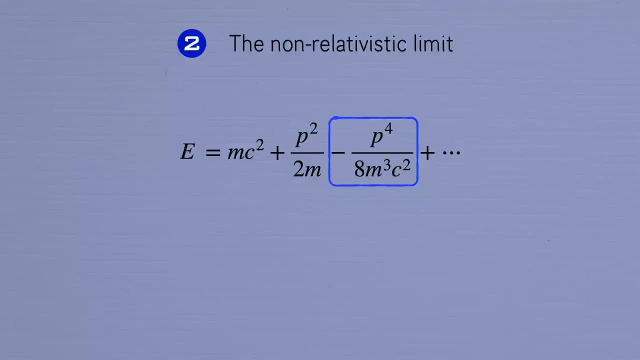 Newton mechanics is a good description of the world for particles that aren't moving anywhere close to the speed of light, but it's only in approximation. This next term in the Taylor expansion is the leading relativistic correction to the Newtonian energy. When the speed is tiny compared to the speed of light, then this additional term gives: 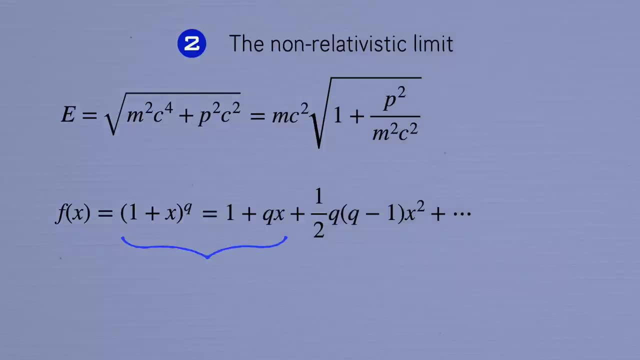 The first pair of terms here is again a very useful approximation that comes up a lot in physics. Now back to the relativistic energy. We just plug in: q equals half and x equals, p squared over, m squared, c squared. Then here's what we get. 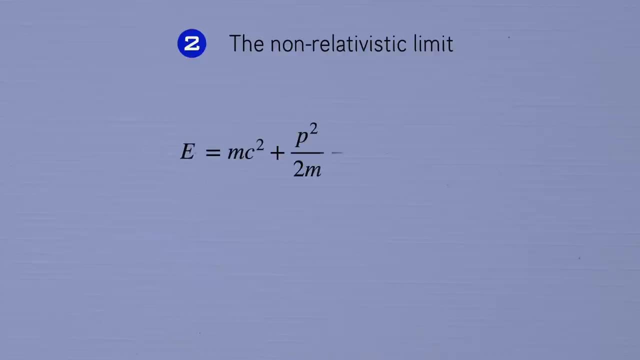 And if we multiply through by the mc squared, here's where we end up: e equals mc squared plus p squared over 2m, Minus p to the 4 over 8m cubed c squared Plus the higher powers of p. 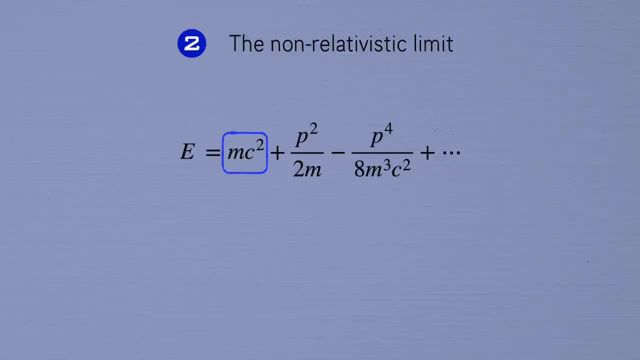 The first term is: e equals mc, squared again, That's what we get by evaluating the energy of a particle at rest in relativity. It doesn't have a direct analog in Newtonian mechanics, but on the other hand it's just a constant and you're always free to add a constant to the total energy in Newtonian. 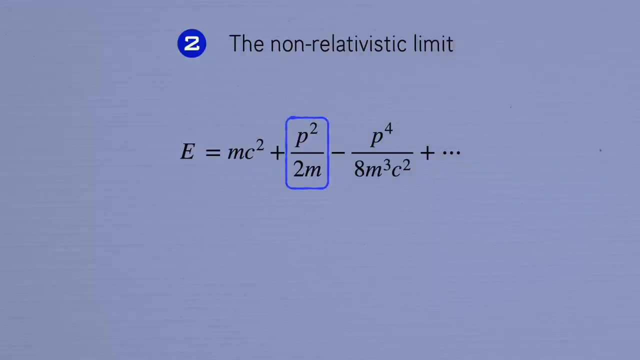 mechanics without changing anything. As for the second term, there we see how the Taylor series reproduces precisely the kinetic energy that we expect in Newtonian mechanics. Actually, I'm being slightly sloppy here, because the definition of the momentum p actually gets modified in relativity, and we should really, Taylor, expand that as well. 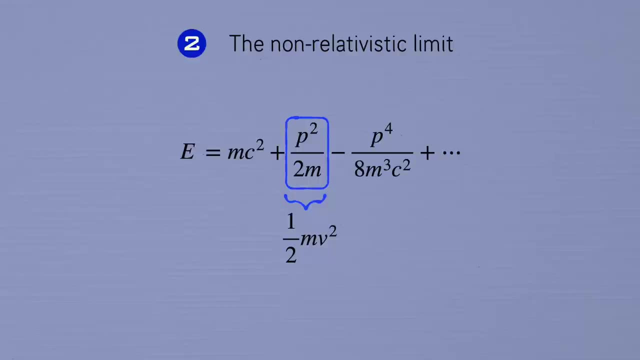 But in the non-relativistic limit we of course get back the Newtonian momentum. p equals mv. But what about this next term in the Taylor series that goes like p to the 4? What are we supposed to make of that? 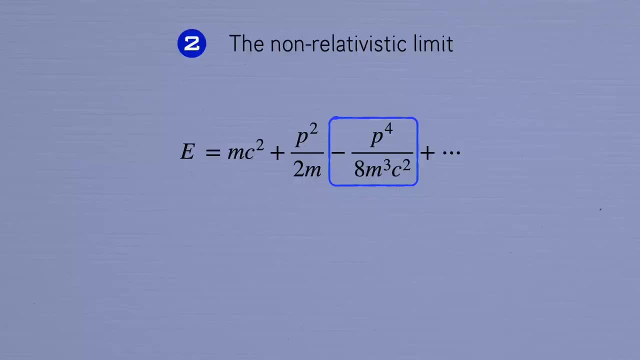 The point is, Newtonian mechanics is a good description of the world for particles that aren't moving anywhere close to the speed of light, but it's only in approximation. But what about this next term in the Taylor series that goes like p to the 4?? 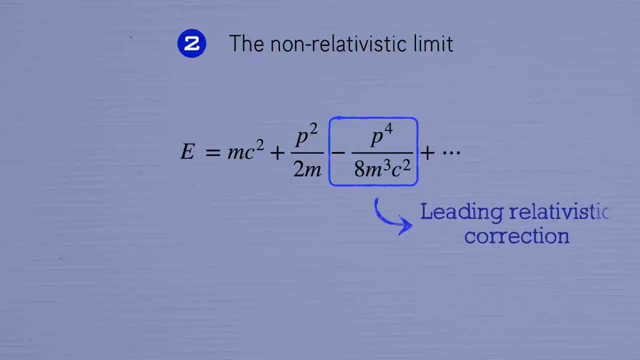 What are we supposed to make of that term? in the Taylor expansion is the leading relativistic correction to the Newtonian energy. When the speed is tiny compared to the speed of light, then this additional term gives a very small correction to Newton's result and we can ignore it without losing much accuracy. But as 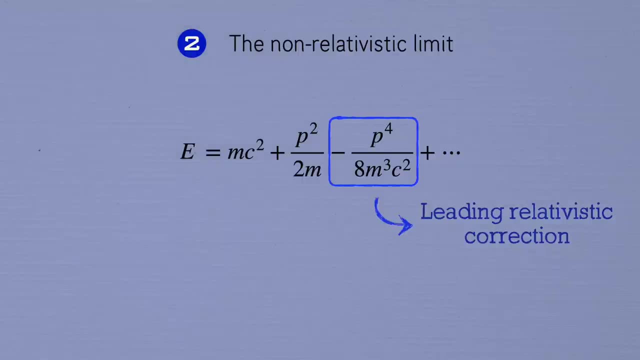 the speed gets larger, this correction becomes increasingly important. One place we can see this correction in action is in the binding energy of a hydrogen atom. That's the amount of energy you would need to kick the electron out of its quote-unquote orbit around the proton at the 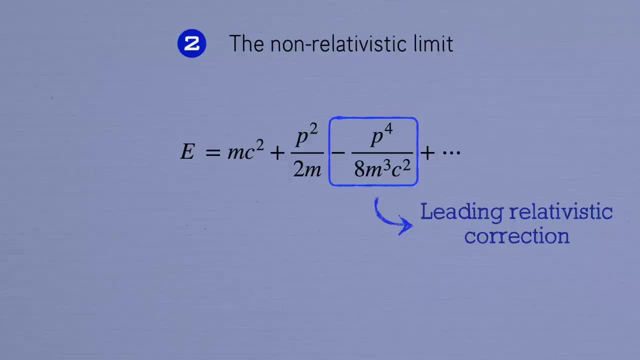 a very small correction to Newton's result and we can ignore it without losing much accuracy, But as the speed gets larger, this correction becomes increasingly important. One place we can see this correction in action is in the binding energy of a hydrogen atom. 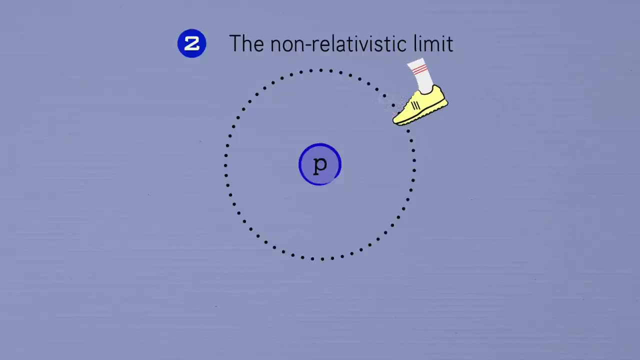 That's the amount of energy you would need to kick the electron out of its quote unquote orbit around the proton at the center of the atom. In a video from a couple of months ago, I showed you how we can get 90% of the way to. 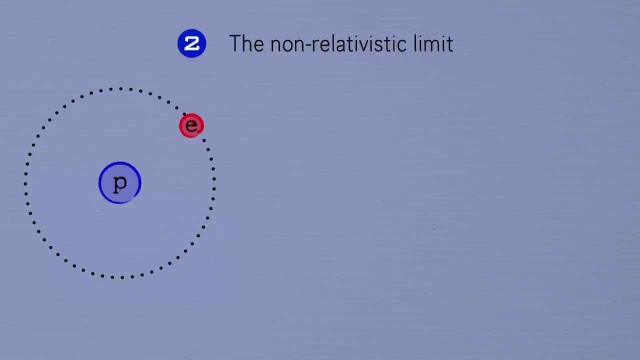 the answer for the binding energy just by applying dimensional analysis, In other words, by making a list of the parameters we have available to play with and their units and seeing how we can combine them to get something with the units that we want. In this case, we saw that we can combine the electron mass m in kilograms. its electric 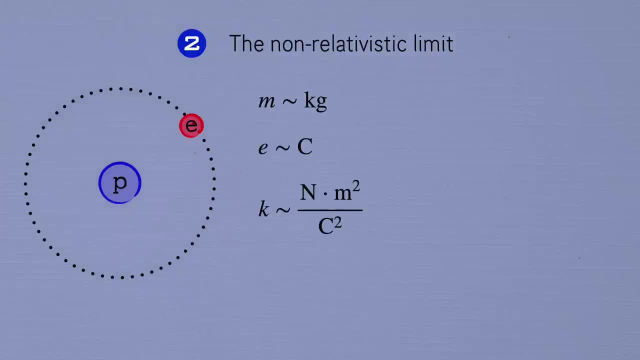 charge e in coulombs, coulombs. constant k, which sets the strength of the electric force in newtons meters squared per coulombs squared, and Planck's constant h-bar, which sets the scale of quantum mechanics in kilograms meters squared per second. 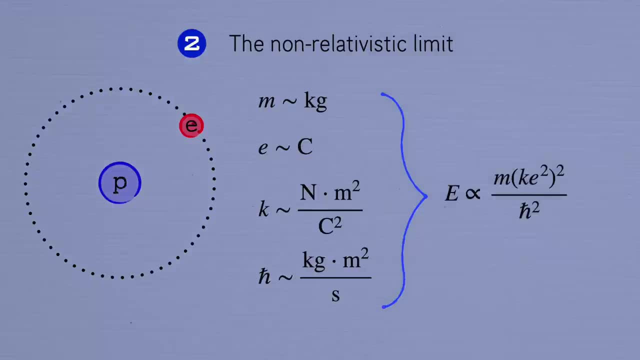 To get units of energy like: so, then the binding energy of the hydrogen atom must be proportional to this. Just by thinking about the units like, this gets us almost all the way to the answer. for the answer, The actual formula for the binding energy comes with a factor of half, though, which 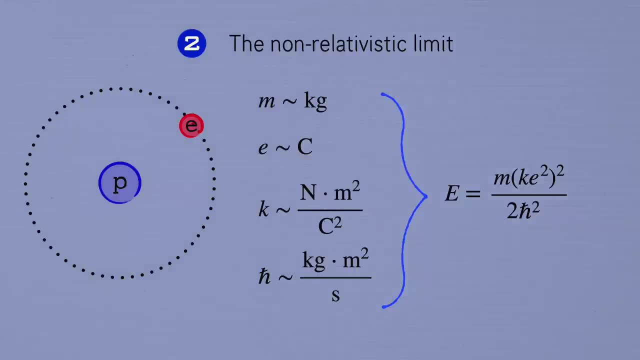 we can't get by only thinking about the units, because 2 doesn't have any units. This is Bohr's formula for the binding energy of hydrogen, and it was one of the first great accomplishments of quantum mechanics. Its numerical value, about 13.6 electron volts, matches very closely to the experimental value. 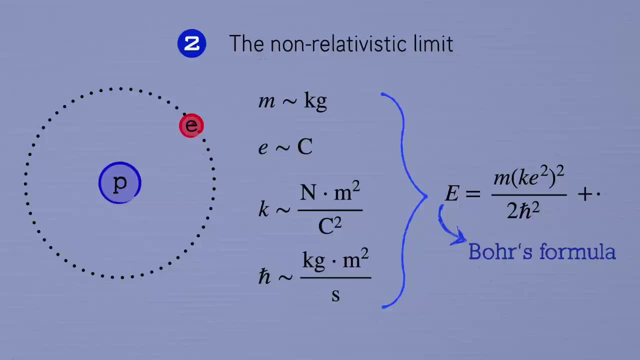 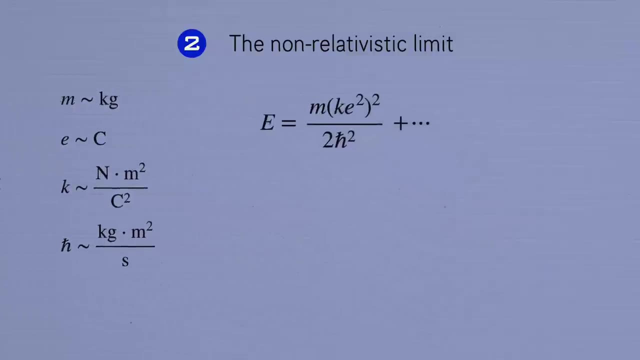 of the binding energy. And yet Bohr's formula is only an approximation. it neglects the small but fascinating and subtle effects of special relativity. But where do we go wrong? in our dimensional analysis argument, We wrote down the only possible way to combine m, e, k and h-bar to make units of energy. 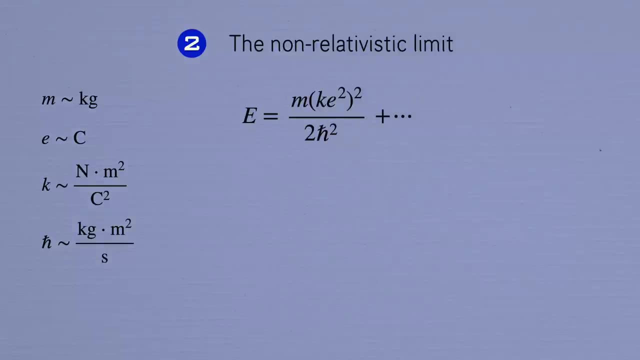 Well, it's not that we went wrong per se, It's that in writing down the non-relativistic approximation to the binding energy, we omitted the speed of light, c, from our list of parameters. So if we want to include the effects of special relativity, we need to consider how c can. 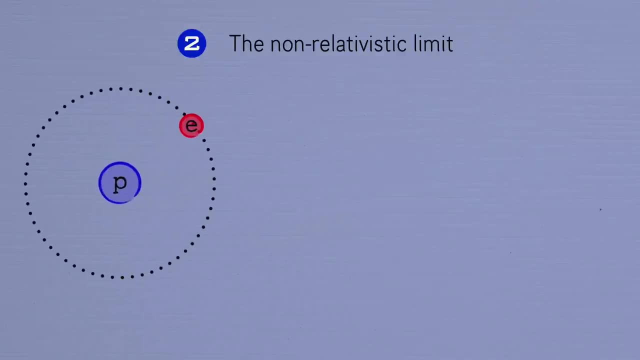 center of the atom. In a video from a couple of months ago, I showed you how we can get 90% of the way to the answer for the binding energy just by applying dimensional analysis, In other words, by making a list of the parameters we have available to play with and their units, and 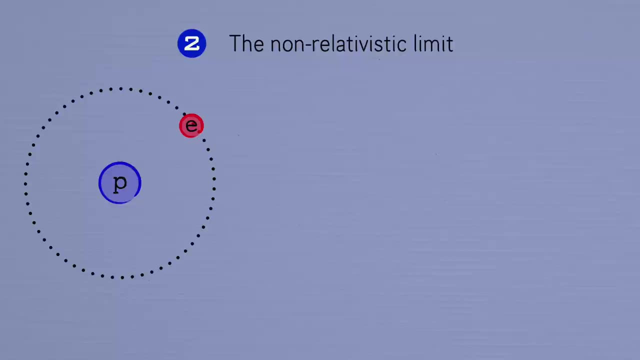 seeing how we can combine them to get something with the units that we want. In this case we saw that we can combine the electron mass, m, in kilograms, its electric charge, e, in coulombs. coulombs constant k, which sets the strength of the electric force. 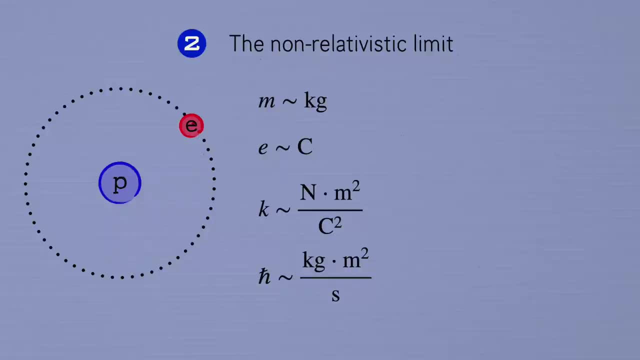 and Newton's meters squared per coulomb squared, and Planck's constant h-bar, which sets the scale of quantum mechanics in kilograms meters squared per second. To get units of energy like so, then the binding energy of the hydrogen atom must be proportional to this. Just by thinking about: 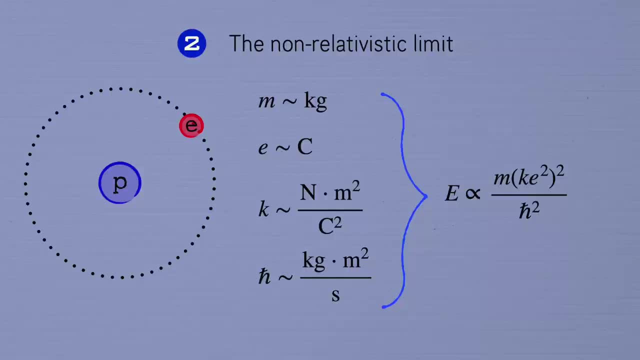 the units. like this gets us almost all the way to the answer. The actual formula for the binding energy comes with a factor of half, though, which we can't get by only thinking about the units, because two doesn't have any units. This is Bohr's formula for. 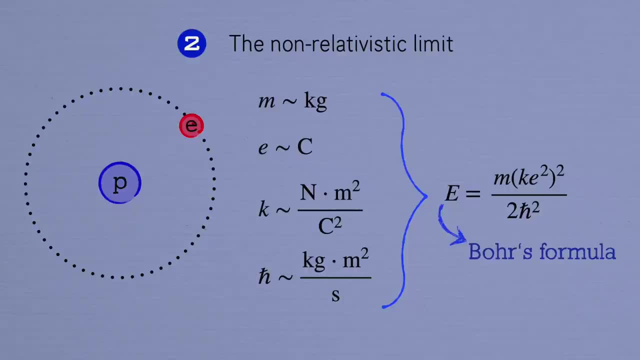 the binding energy of hydrogen, and it was one of the first great accomplishments of quantum mechanics. Its numerical value, about 13.6 electron volts, matches very closely to the experimental value of the binding energy. And yet Bohr's formula is only an approximation. 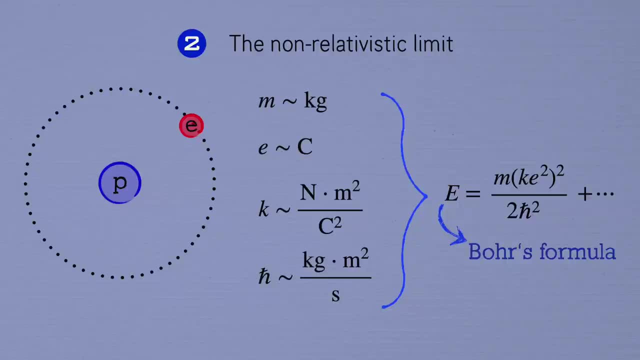 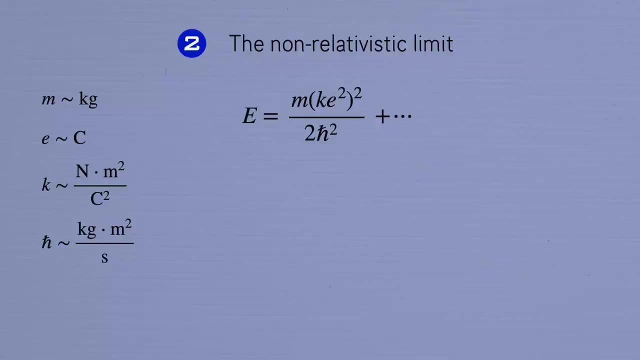 It neglects the small but fascinating and experimentally observable effects of special relativity. But where do we go wrong? in our dimensional analysis argument We wrote down the only possible way to combine m, e, k and h-bar to make units of energy. 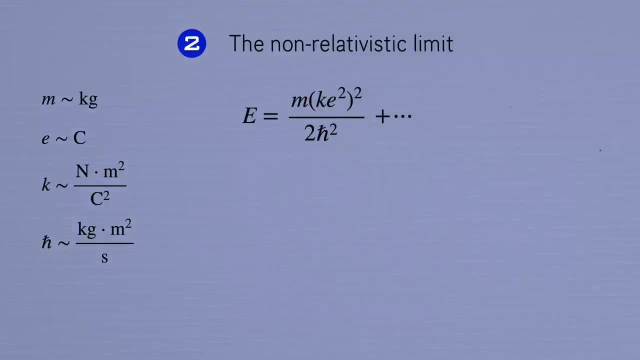 Well, it's not that we went wrong per se, It's that in writing down the non-relativistic approximation to the binding energy, we omitted the speed of light, c, from our list of parameters. So if we want to include the effects of special relativity, we need to consider how c can enter. 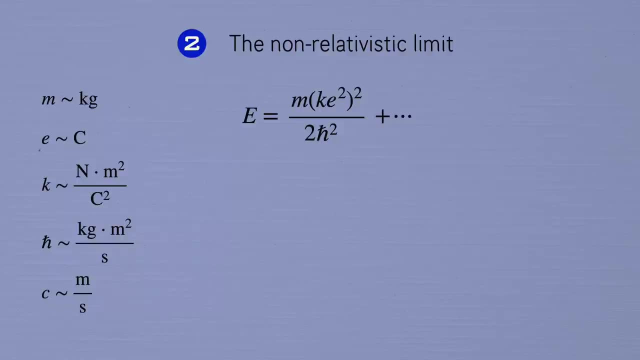 the formula for the energy. But something remarkable happens: when we add c to the list of parameters. We can form a dimensionless combination by alpha equals k, e squared over h-bar c. This combination is called the fine structure combination. I'll leave it for you to check that all the dimensions really do cancel out here when. 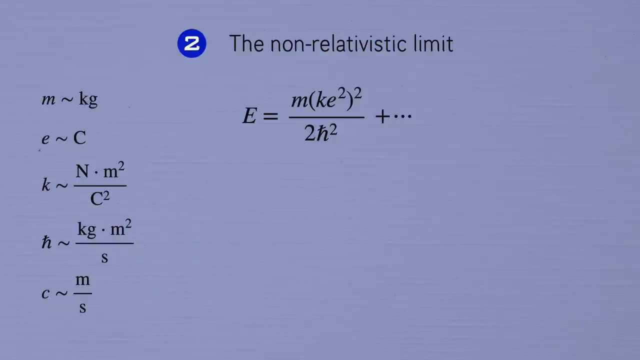 enter the formula for the energy. But something remarkable happens When we add c to the list of parameters. we can form a dimensionless combination by alpha equals ke squared over h-bar c. This combination is called the fine structure constant. I'll leave it for you to check that all the dimensions really do cancel out here when. 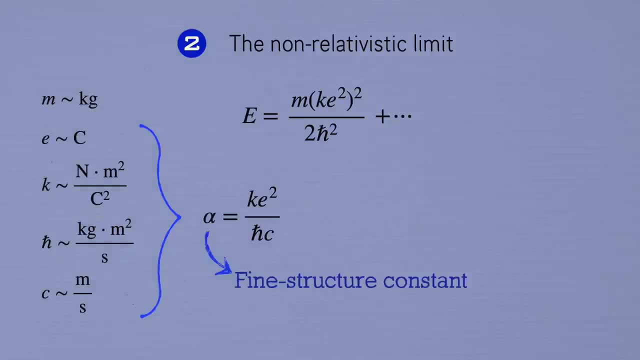 you plug in the units. If you put in the numbers, you'll find that alpha is about 0.0073, or, a little more memorably, about 1 divided by 137.. Since alpha is unitless, dimensional analysis doesn't tell us anything about how it appears. 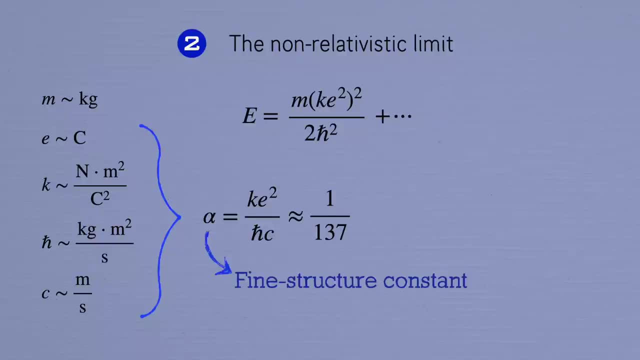 in the formula for the energy, No more than it could tell us about the factor of 2 in the denominator. Any function of alpha can multiply our expression for the energy without spoiling the units. This is how relativity allows small corrections to Bohr's formula, which, remember, was: 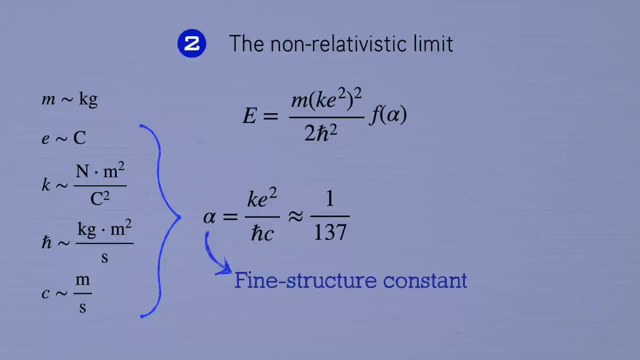 itself already an excellent approximation to the experimental value of the hydrogen binding energy. But we can get an even better theoretical prediction by considering the relativistic corrections. With that leading relativistic correction that we derived by applying the Taylor series, we can now calculate the energy of the unit. 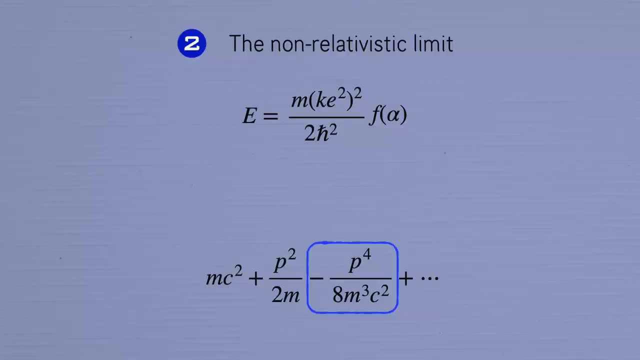 By applying the Taylor series to Einstein's formula we can determine the small modification that relativity makes to Bohr's formula. The details require quantum mechanics, so I won't go into that here, but the result is that this function f is given by 1, that was for the original Bohr answer plus 5 fourths. 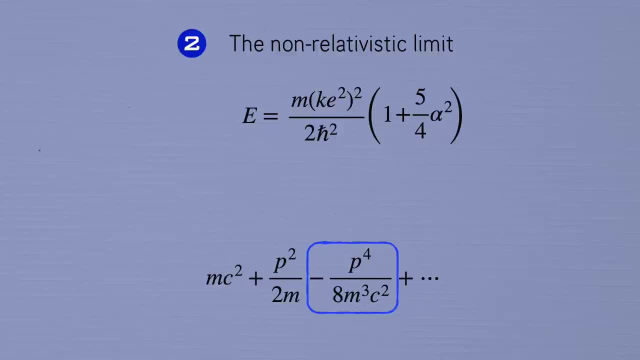 alpha squared. Remember that alpha is a tiny number, so this correction that goes like alpha squared is even tinier still. It's therefore called a fine structure correction to the energy. There are, in fact, further corrections to this formula, Both at order alpha squared, as well as even smaller corrections at higher orders in. 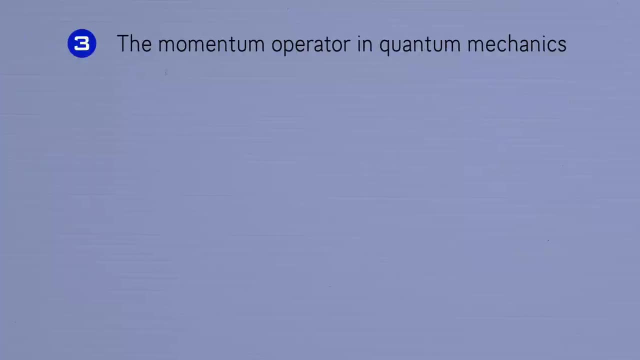 alpha from various physical effects. Finally, while we're on the subject of quantum mechanics, let's finish by seeing how Taylor's formula is related to the definition of momentum in quantum mechanics. In classical mechanics, the main question is to solve for the trajectory x of t, of a. 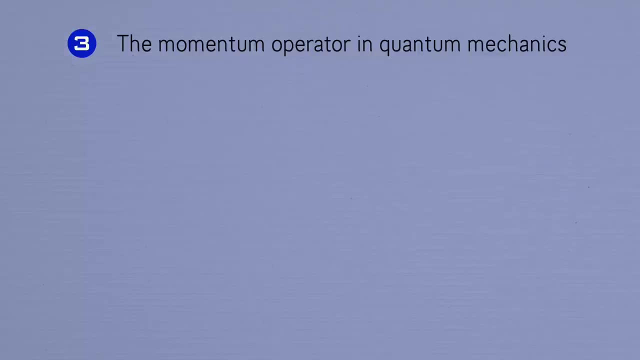 particle as a function of time. In quantum mechanics, on the other hand, the goal is to find the wavefunction psi of x and how it evolves with time. Wherever the wavefunction, or rather its square, is located, it is possible to find the wavefunction. 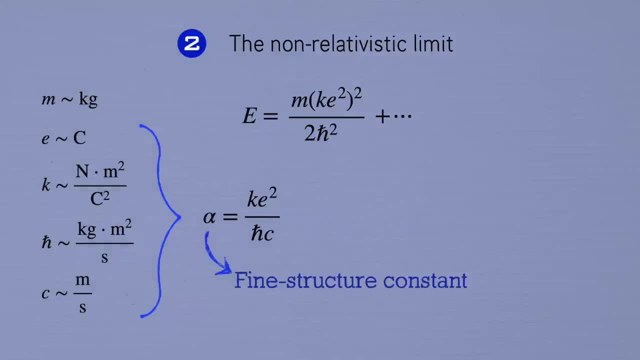 you plug in the units. If you put in the numbers, you'll find that alpha is about 0.0073, or, a little more memorably, about 1 divided by 137.. Since alpha is unitless, dimensional analysis doesn't tell us anything about how it appears in the formula for the energy. 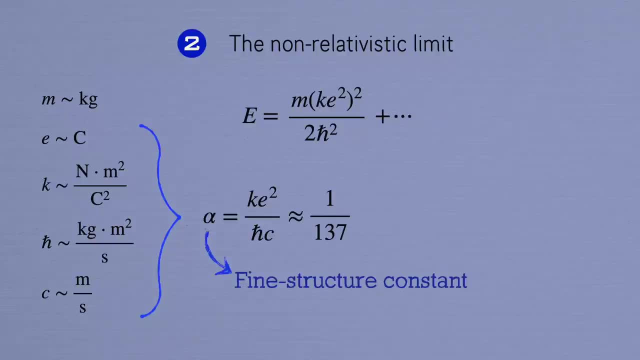 no more than it could tell us about the factor of 2 in the denominator. Any function of alpha can multiply our expression for the energy without spoiling the units. This is how relativity allows small corrections to Bohr's formula which, remember, was itself already. 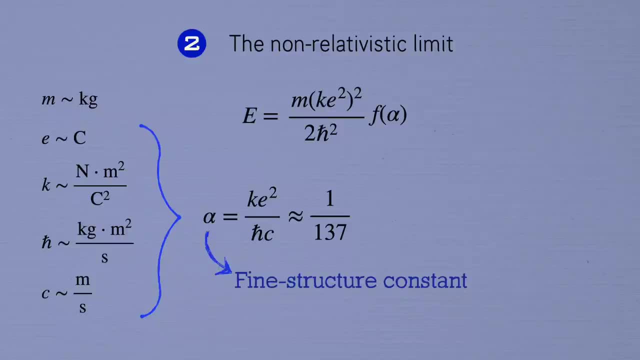 an excellent approximation to the experimental value of the hydrogen binding energy. But we can get an even better theoretical prediction by considering the relativistic corrections. With that leading relativistic correction that we derived by applying the Taylor series to Einstein's formula, we can determine the small modification that relativity makes to Bohr's. 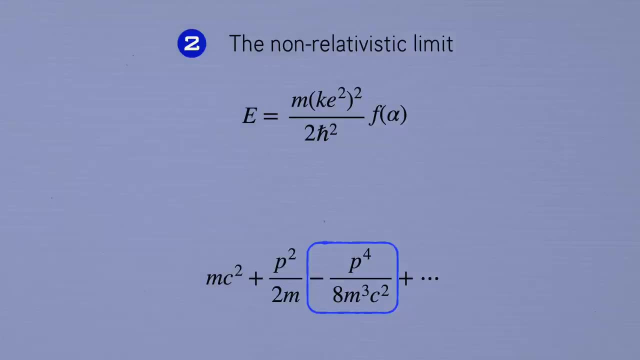 formula. The details require quantum mechanics, so I won't go into that here. But the result is that the function f is given by 1, that was for the original Bohr answer plus 5, fourths alpha squared. Remember that alpha is a tiny number. so this correction that goes like alpha squared. 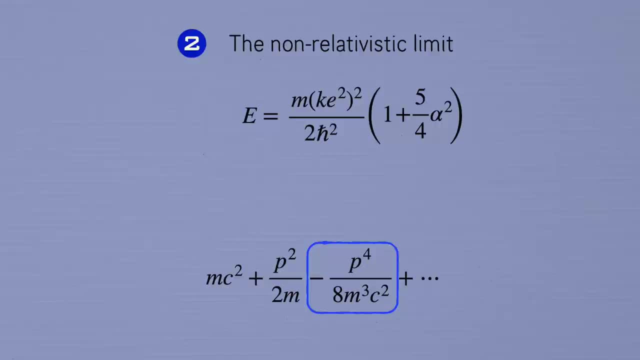 is even tinier still. It's therefore called a fine structure correction to the energy. There are in fact further corrections to this formula, both at order alpha squared, as well as even smaller corrections at higher orders in alpha from various physical effects. Finally, 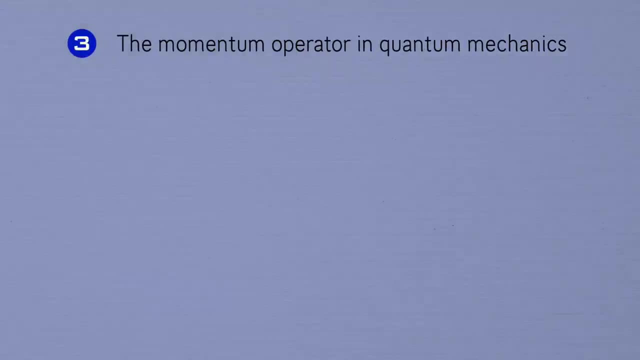 while we're on the subject of quantum mechanics, let's finish by seeing how Taylor's formula relates to the definition of momentum in quantum mechanics. In classical mechanics, the main question is to solve for the trajectory x of a particle as a function of time. 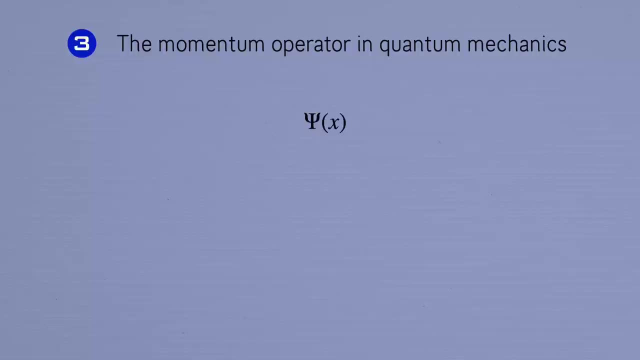 In quantum mechanics, on the other hand, the goal is to find the wave function psi and how it evolves with time. Wherever the wave function, or rather its square, is bigger, the more likely you are to find the particle at that location when you make a. 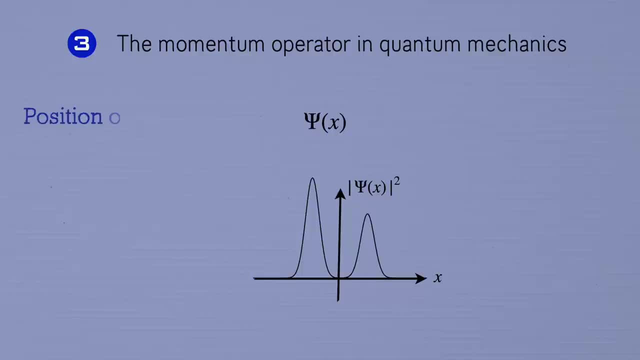 measurement. Those things that we measure about the particle, like its position and momentum, are represented by operators that act on the given moment. They're all equal in their own way. on the wavefunction We write x-hat for the operator that measures the position and p-hat. 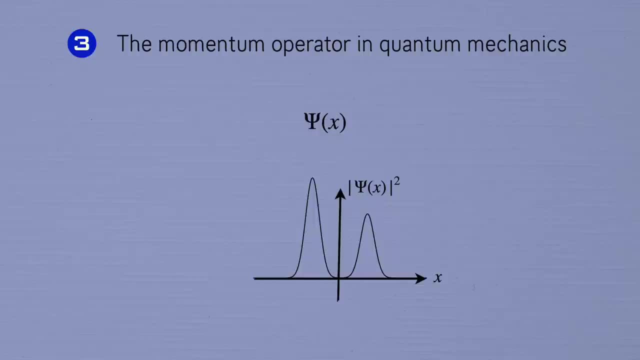 psi of x and how it evolves with time. If the wavefunction, or rather its square, is bigger, the more likely you are to find the particle at that location. when you make a measurement, Those things that we measure about the particle, like its position and momentum, are represented. 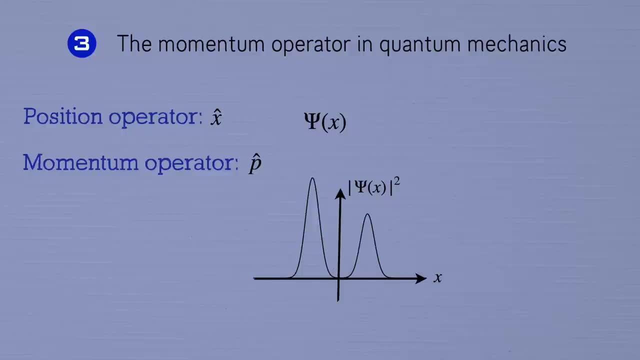 by operators that act on the wavefunction. We write x-hat for the operator that measures the position and p-hat for the operator that measures the momentum. The point of this video isn't to learn quantum mechanics right now, but I gave you a bit. 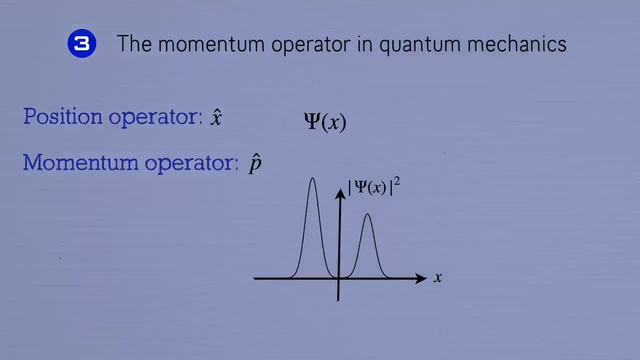 of a crash course in the video I posted about symmetries in quantum mechanics that I'll link in the description if you want to see more. I told you there about how the momentum operator works. The momentum operator is closely related to translations in space. 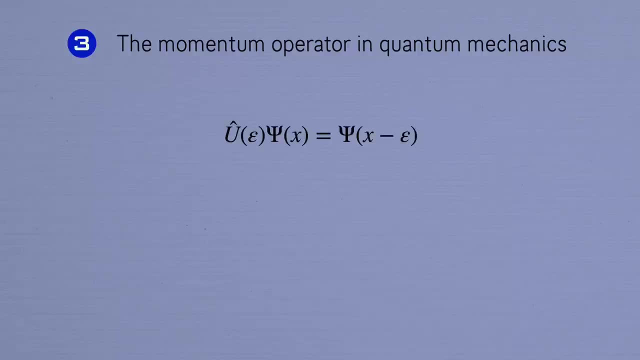 So let's define an operator- call it u- of epsilon that shifts the wavefunction over by epsilon. If you haven't seen those earlier videos where I explained more about what all this means, don't sweat it. right now We'll just take this as a definition and discover how it's related to Taylor's. 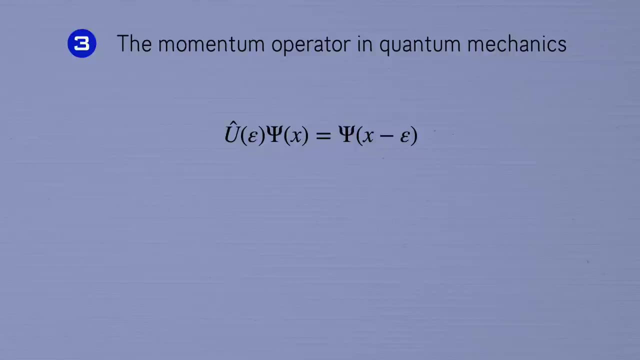 formula, And indeed this looks familiar. Physics aside, psi of x is just a function, And this formula tells us that we're looking for an operator that shifts psi of x over to psi of x minus epsilon, And that's exactly what Taylor's formula does. 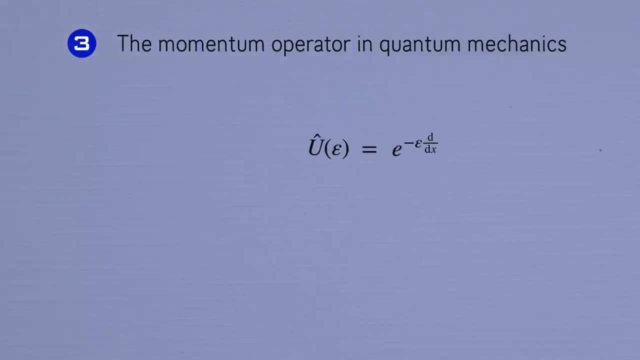 Therefore we identify the translation operator u with e to the minus epsilon d by dx. For reasons we won't delve into right now, this translation operator u is related to the momentum operator by u of epsilon. equals e to the minus i over h bar epsilon times. 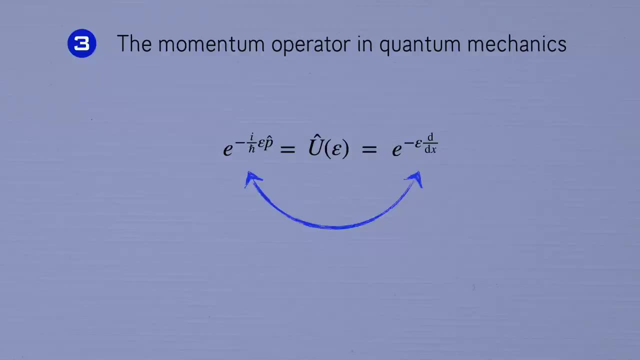 p. Then, comparing the two sides, Taylor's formula shows us that we should identify the momentum operator in quantum mechanics with p equals h bar over i d by dx. So we get p equals h bar over i d by dx And p equals h bar over i d by dx. 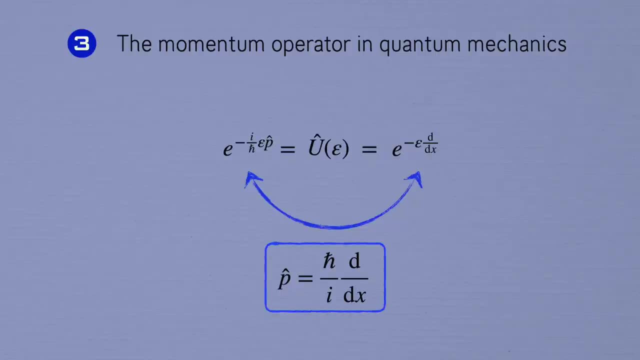 So we get p equals h bar over i, d by dx, And that's all we need to do to get the momentum. start studying quantum mechanics. this will be one of the first formulas you'll learn. It follows directly from Taylor's formula. This has been just a small selection of physics. 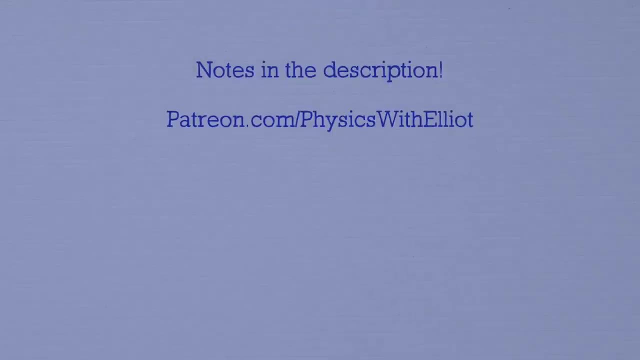 applications where Taylor's formula shows up. but again, you'd really be hard pressed to find any chapter of any physics textbook where it isn't applied. Keep your eyes open and you'll see Taylor's formula everywhere. You can find the notes for this video, as well as links to 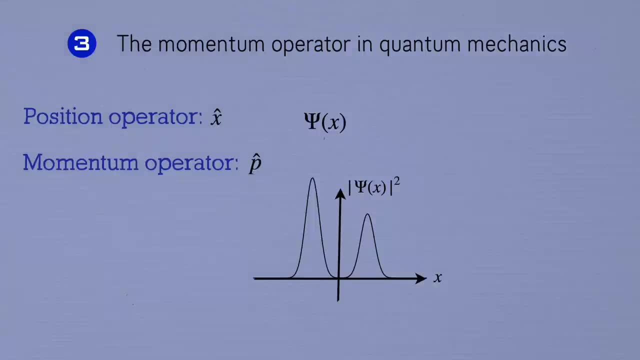 for the operator that measures the momentum. The point of this video isn't to learn quantum mechanics right now, but I gave you a bit of a crash course in the video I posted about symmetries in quantum mechanics. that I'll link in the description if you want to see. 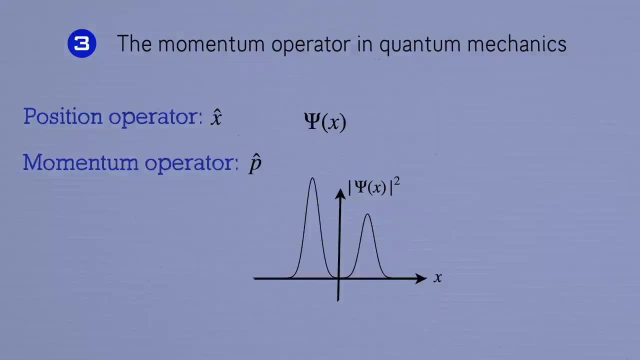 more. I told you there about how the momentum operator is closely related to translations in space. So let's define an operator- call it u of epsilon, that shifts the wavefunction over by epsilon. If you haven't seen those earlier videos where I explained more about, 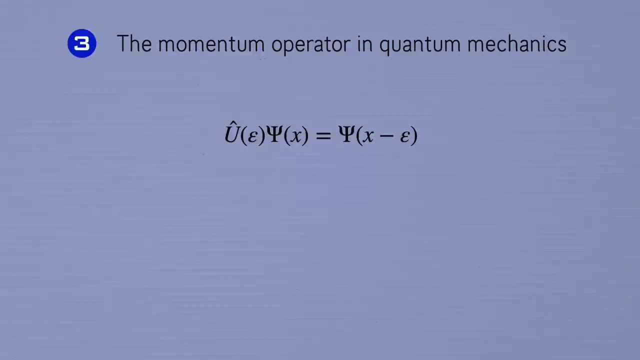 what all this means. don't sweat it right now. We'll just take this as a definition and discover how it's related to Taylor's formula, And indeed this looks familiar. Physics aside, psi of x is just a function, And this formula tells us that we're looking. 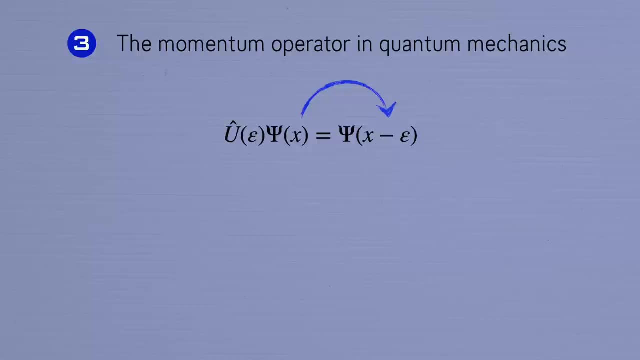 for an operator that shifts psi of x over to psi of x minus epsilon, And that's exactly what Taylor's formula does. Therefore, we identified the translation operator u with e to the minus epsilon d by dx, For reasons we won't delve into right now. this translation operator u is related to: 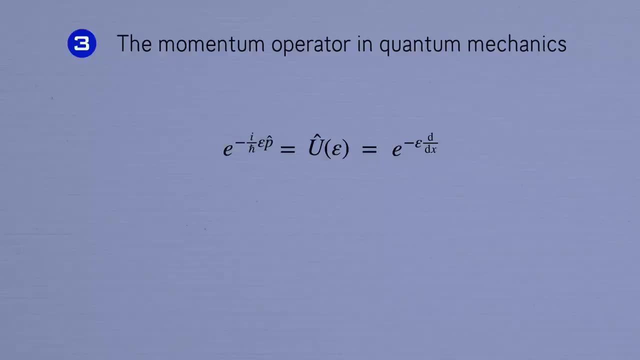 the momentum operator by u of epsilon equals e to the minus i over h-bar epsilon times p. Then, comparing the two sides, Taylor's formula shows us that we should identify the momentum operator in quantum mechanics with p equals h-bar over i d by dx. When you do, 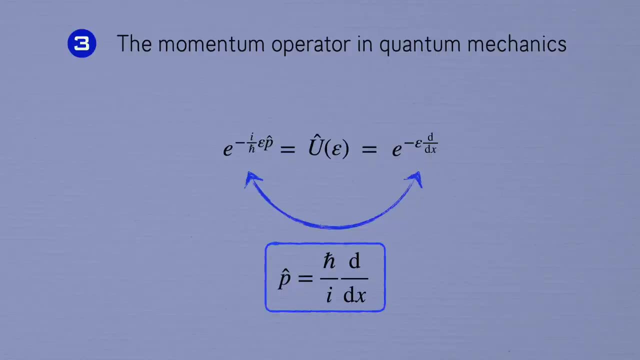 start studying quantum mechanics, this will be one of the first formulas you'll learn. It follows directly from Taylor's formula. This has been just a short video. If you have any questions, feel free to leave a comment. I'll be happy to answer any questions you may have. If you have any questions, feel free to 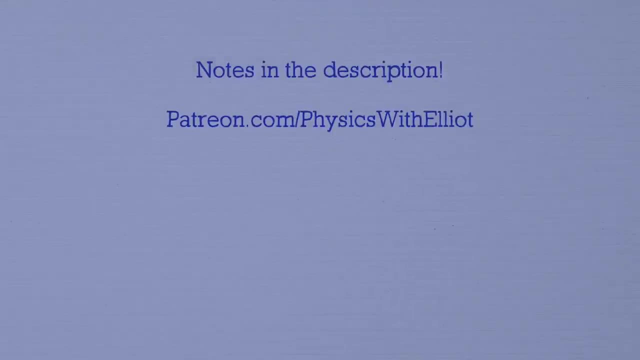 leave a comment. I'll be happy to answer any questions you may have. There's a small selection of physics applications where Taylor's formula shows up, But again, you'd really be hard-pressed to find any chapter of any physics textbook where it. 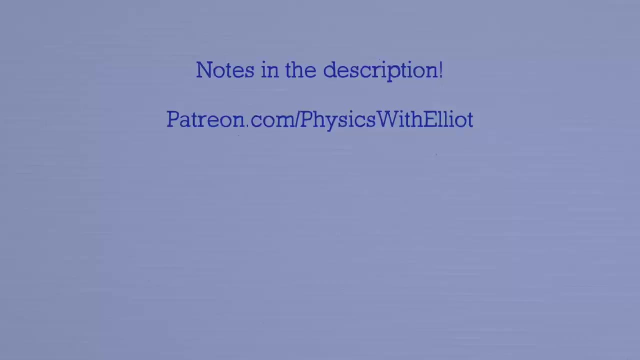 isn't applied. Keep your eyes open and you'll see Taylor's formula everywhere. You can find the notes for this video, as well as links to all the earlier videos that I mentioned down in the description, If you liked the video and you want to help support. 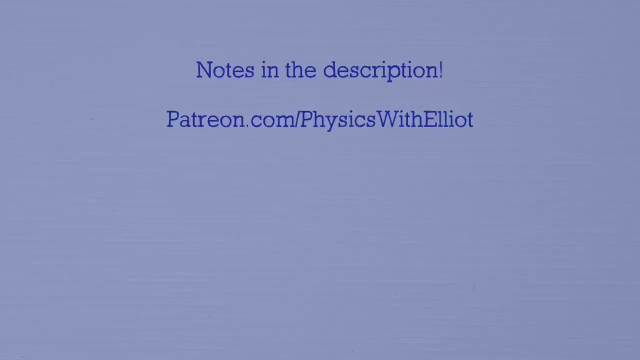 the channel. I'll also put a link to my Patreon page. Thank you so much for watching and I'll see you back here soon for another physics lesson. 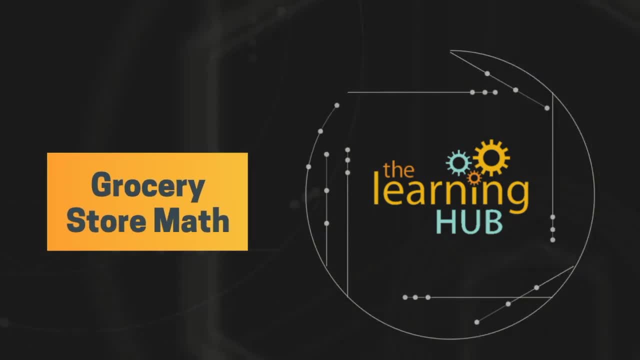 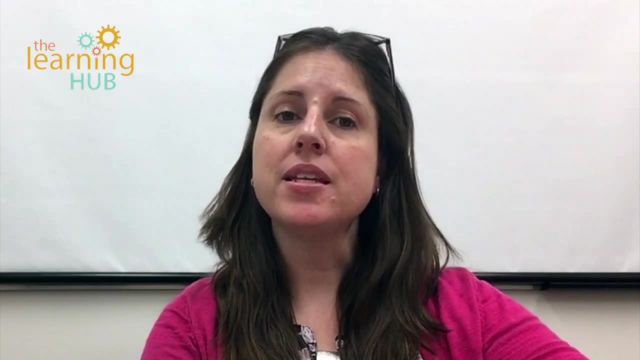 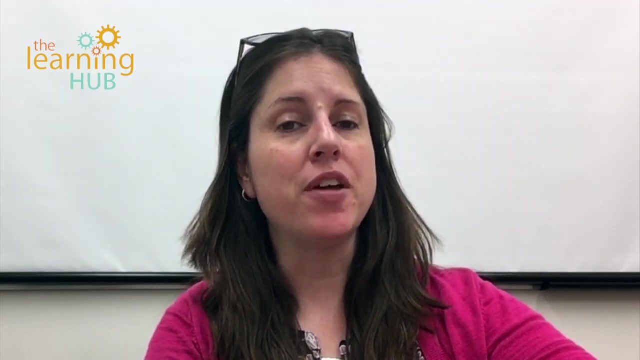 How to use math to comparison shop and save money. Math isn't scary, and when you use it in everyday life, you'll become more comfortable with math. Today, I'm going to show you how to find the unit price of a product in a grocery store.